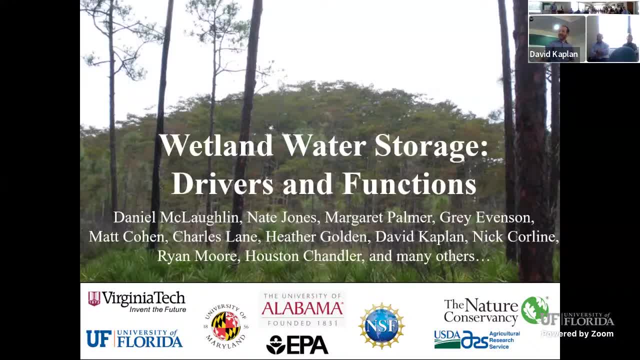 here, but he got an additional undergraduate degree in mathematics. So if you have any questions about complex mathematics, you can ask Dr McLaughlin. Dr McLaughlin is, let's make sure we got our stream going. Megan tells me looking good All. 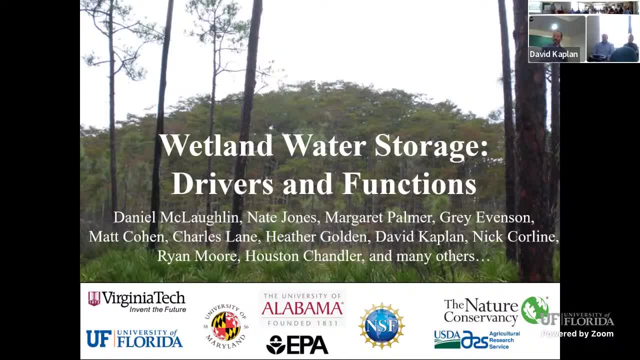 right. So he's an associate professor in the Department of Forest Resources and Environmental Conservation at Virginia Tech. Welcome y'all, Have a seat. His research integrates hydrological and ecological processes and includes interest in watershed hydrology, forest and ecosystems and basically everything eco-hydrology. So Daniel loves tromping through wetlands You won't find. 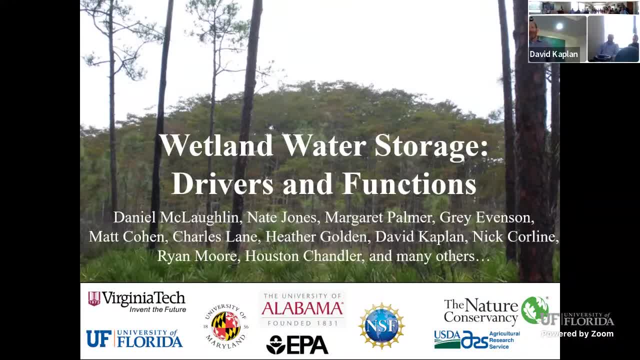 him in a pair of waders. He has these old sneakers that he walks And these are new sneakers that he has today. But he's walking through wetlands to feel the squish below his feet and try to understand how water plants, biogeochemistry all interact. to. 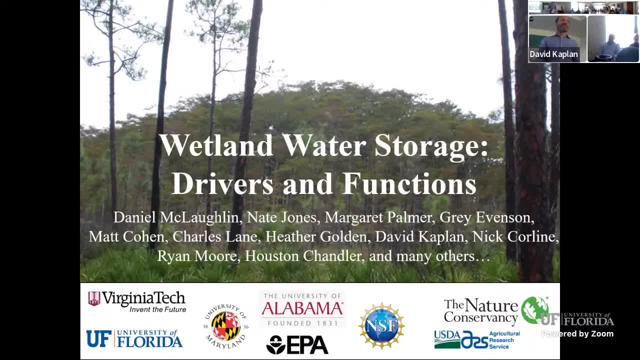 basically make wetlands work, And they work either for ecosystems in their own rights or just their own value. But a lot of times he's looking at water and other water quality services that wetlands provide for humans, for us, and tries to do that in a very analytical way, while 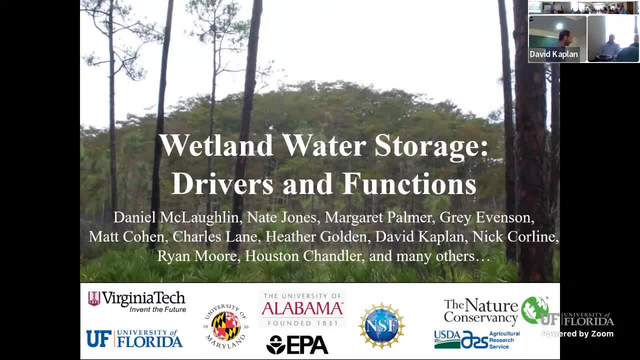 still getting out and squishing at the mud. So with that, Daniel, I give you the floor And you should be good to go, All right, Well, yeah, this is an honor for me. It was a big pleasure. I was just telling Matt that. 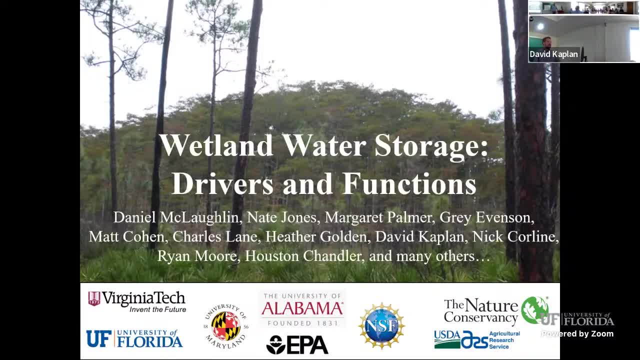 I think this is the first time I've been in this room since 2014.. And it hasn't changed. But I had my defense in here and several other talks and everything else, And I've seen many of you talk in here as well. So, yeah, again, it's a big pleasure to be here. see the town, see how it. 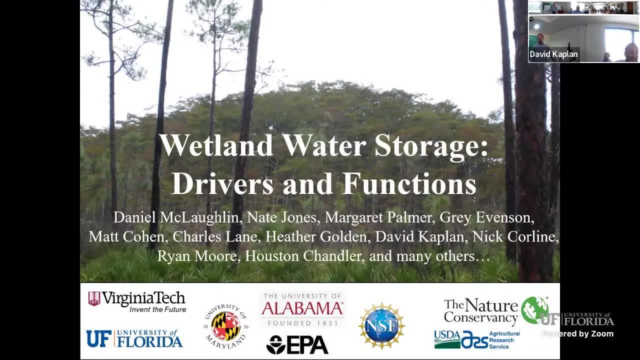 has changed how. it hasn't changed what's the topic? Yeah, it's a big pleasure to be here. It's a big pleasure to be here. So, yeah, I plan on staying through Sunday. So I'm trying to see the sites. I'm supposed to be here. This is our first semester. 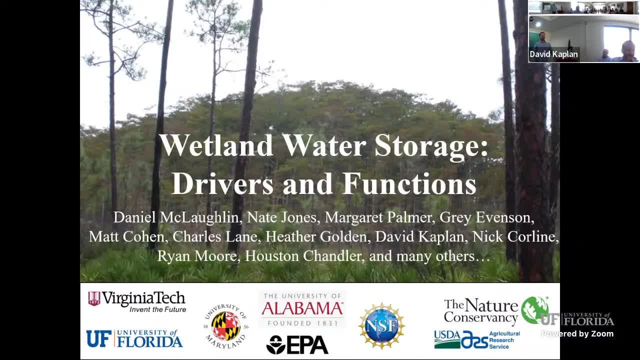 at Virginia Tech. Yeah, so I've got to record the lecture so they can see it. So today I want to give just a high level look at multiple different projects, starting with projects here with colleagues here that I've kept up with that have motivated other projects that 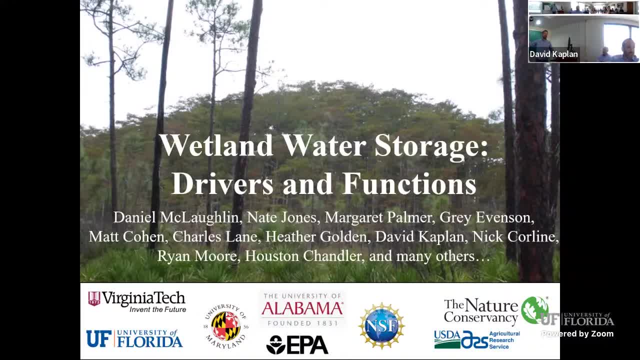 I'm working on now. under this broad umbrella of wetland water storage right, It's distributed in landscape, particular landscapes, and what drives that water storage, which might be kind of obvious in terms of the first order, would be topography right, But then the functions that emerge from. 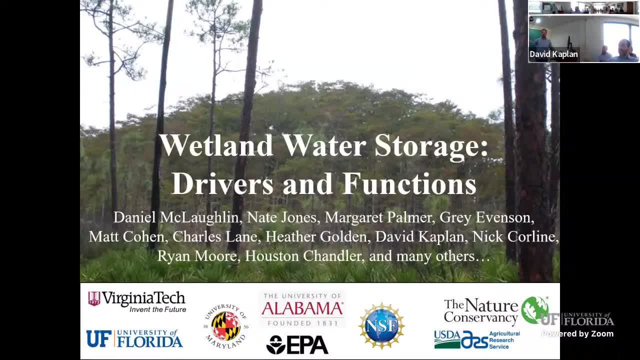 that distributed water storage. A lot of folks listed here, some are in the room, Many. I could still list a lot of different places in terms of funding and collaborations, And you might recognize some of those names. Okay, Before I get to really the theme of today, which is about 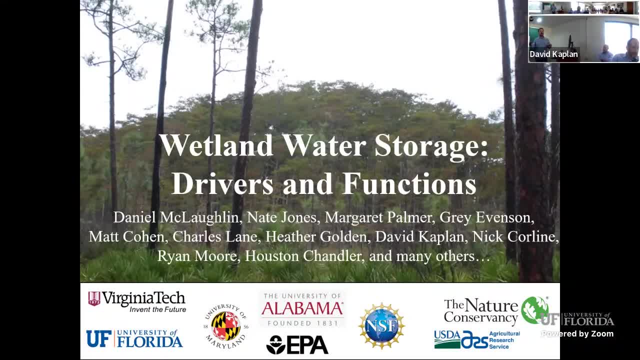 a pretty broad class of wetlands, smaller depressional wetlands, that many landscapes. I do want to take a step back just because I'm here And I just walked by that poster that's been there for a long time, So to where I got introduced to wetlands, So I visited. 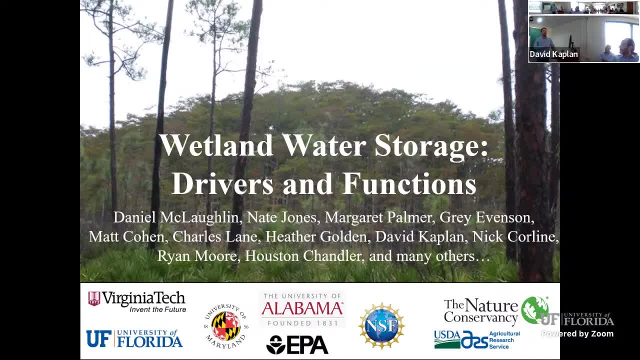 here. I think it was in February of 2004.. And I was walking around. I got here a day early for the recruiting weekend And I noticed that people were playing volleyball and didn't have any clothes on. This is great. And then I somehow stumbled to the Center for Wetlands. I've already talked to 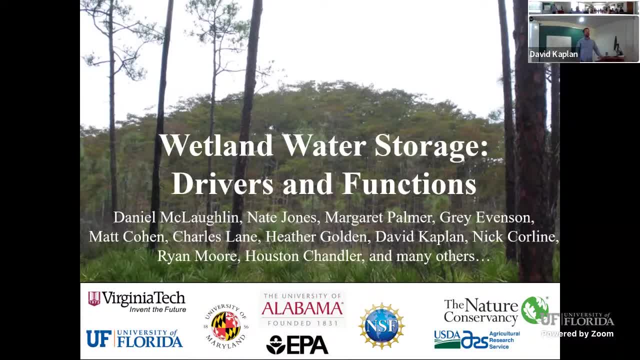 Mark Brown via email and invited him to here, but he didn't offer me a project or anything And I wasn't trying to find this place. I was just walking, aimlessly walking around, as you know I can. And then so well didn't? you? were in the office when it was, when you had your green ceiling. 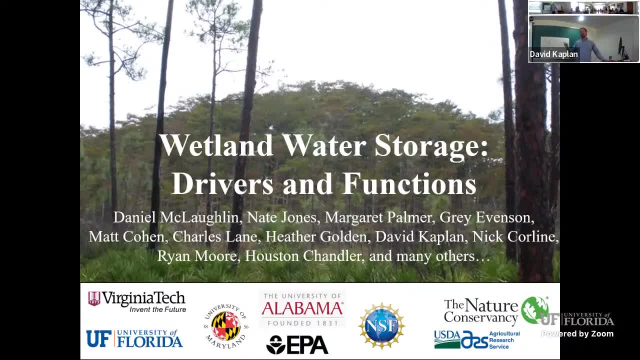 that office down there And we talked about the beautiful Bone Valley district and how that would be a great project to work on And I think about that- Yeah, restoration. I came back so excited. I called my girlfriend at the time. I had a pay phone in the right. 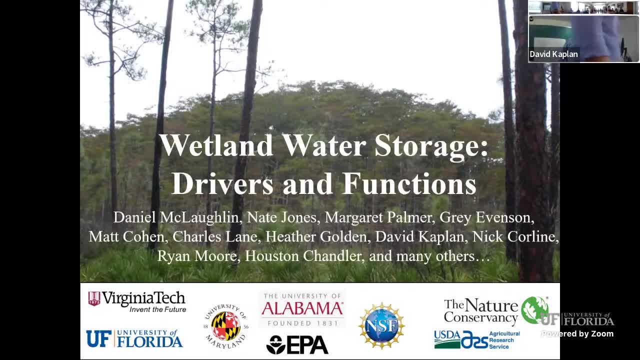 I didn't have a cell phone at the time and you have to write this into your abstract. and then I got back to Clemson, where I was, and I started emailing Wes Ingersoll, who was already on the project. yeah, it's not a great place to stay at. 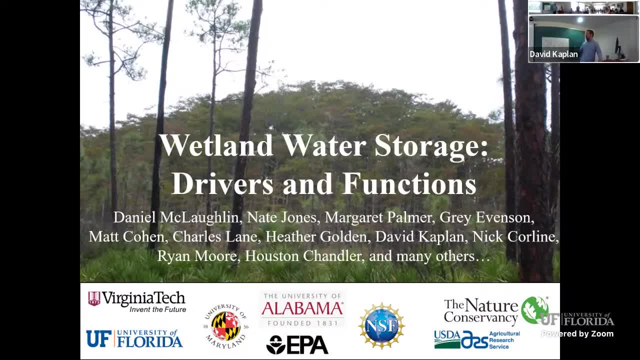 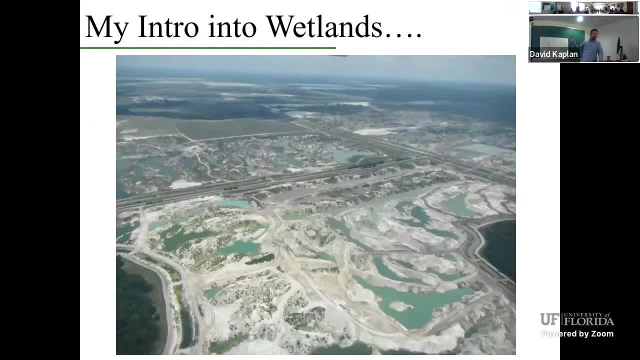 Davis Brothers Motor Lodge. so I can't get back to this what I want to before at least showing you how nasty that landscape can be. I think this is actually a picture from you, Mark, I'm not sure. but our goal in the larger: what was the Fipper? there you go. 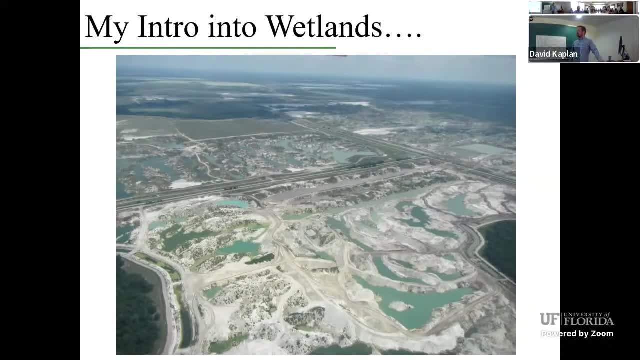 to look at wetland restoration and creation on these one of the post-Fosset landscape elements which are place settling areas, and looking at what's naturally occurring in restoration. so we got to go out there there and I didn't wear waders, I didn't plan this. 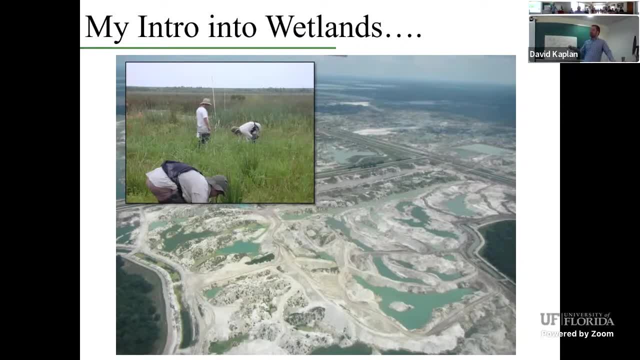 that's when I first wore waders. I think that was my first day in the building. I was like, why are we wearing waders? this is hot as hell. so I've ditched those and the hat, because it's kept on falling off. and I believe that is Wes Ingersoll. 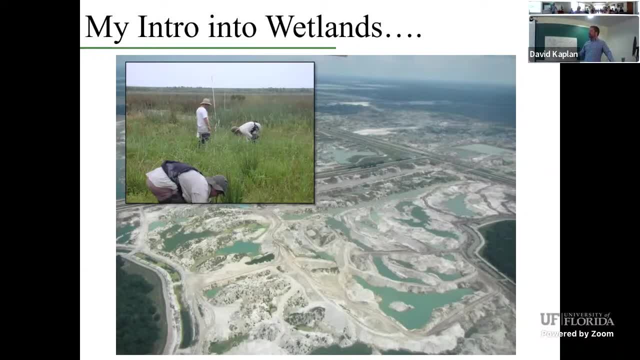 that is Wes Ingersoll. right there there's his brother, Lance. he helped out. we had a lot of people help out on that project. we met a lot of cool people, and so we were looking at what's naturally occurring in terms of vegetation, the topography. 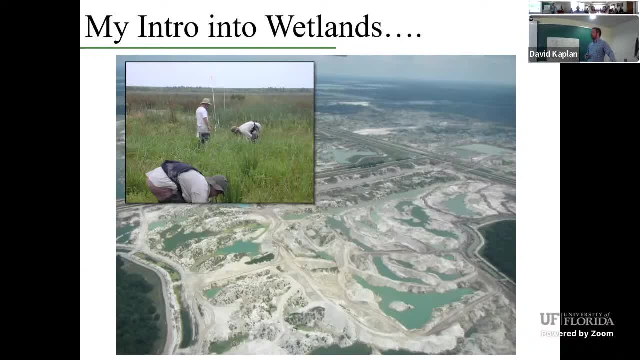 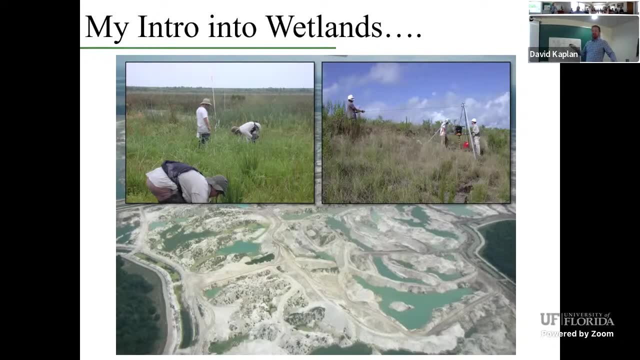 the soils come back and particularly the hydrology, and we went down the road for hydrology even a little more. we found this general hole digger back in some shed- I think was at the- and that thing was terrible. we'd get stuck. we had to have a pulley anyway. trying to figure out dyke. 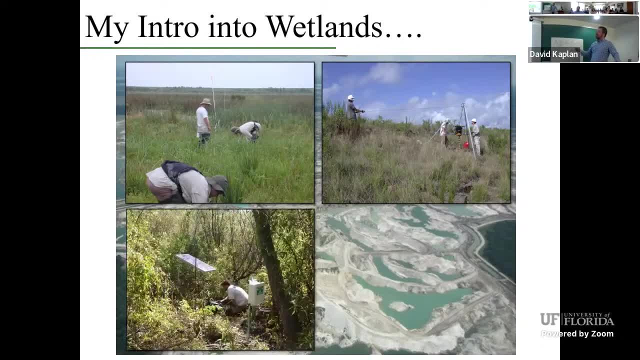 seepage, which I think became one figure in my defense, our money dissertation, um. and then where I really focused some of my work was on that term. the buzzword at the time was ecohydrology and thinking about feedback of vegetation that indeed was coming in there, which was primarily willow. 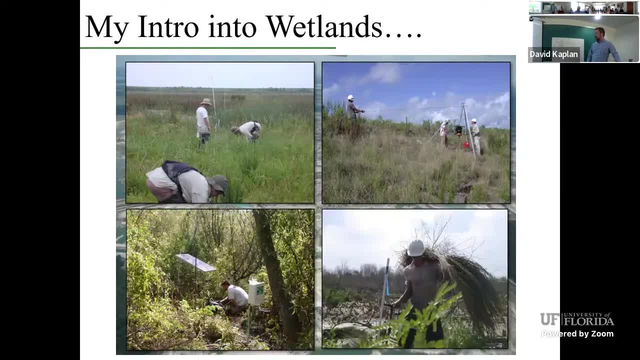 but all of that part of the larger project was to inform active restoration. there's Wes bringing in some vegetation, working alongside with contractors, and there's one of this tree in the foreground. I'd love to get back there and see what it looks like. I don't know if you've been. 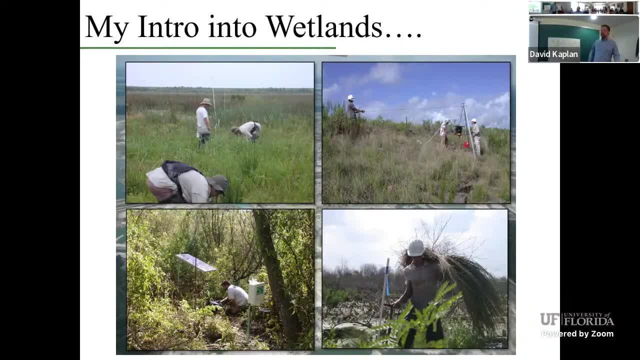 back, but no, not to. so that was somebody said: if you've been back there, what's going on with? I think Sherilyn does, I have no idea. I left there in joy, okay, um, and so then I started, uh, moved on to work with Matt Cohen at. 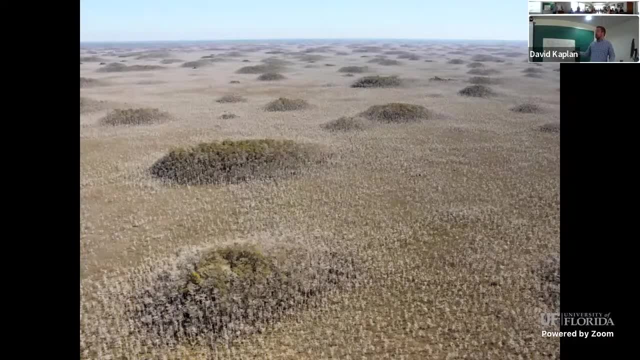 SFRC- which I don't think it's called that anymore- and um, and working on wetlands that are naturally occurring, and found our way working on a particular set of wetlands, um, one of which is not where I started, but this is Big Cypress, as an example, a great example of um, a landscape where you have 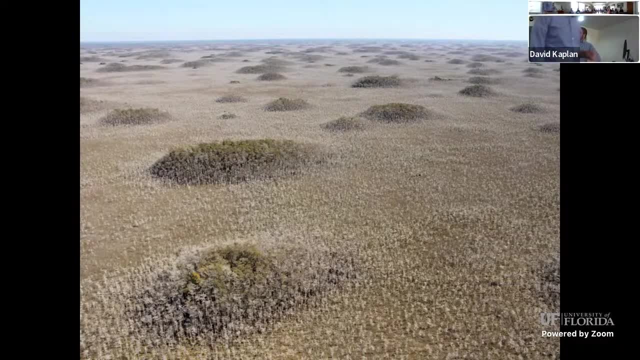 these smaller depressional wetlands, in this case cypress stones dotting the landscape that most often do not connect the surface line right. you can walk around and keep your feature, as we say most of the time um. these types of wetlands exist in other regions, like the Prairie Pothole region. we can actually 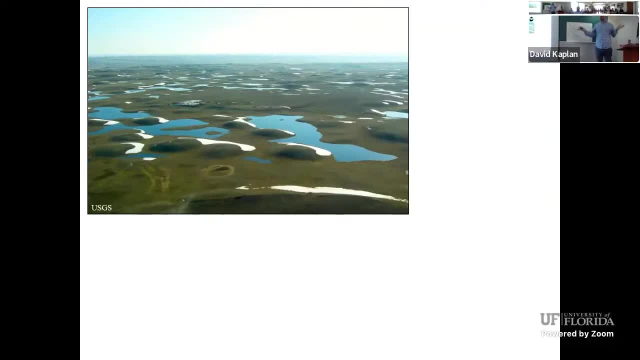 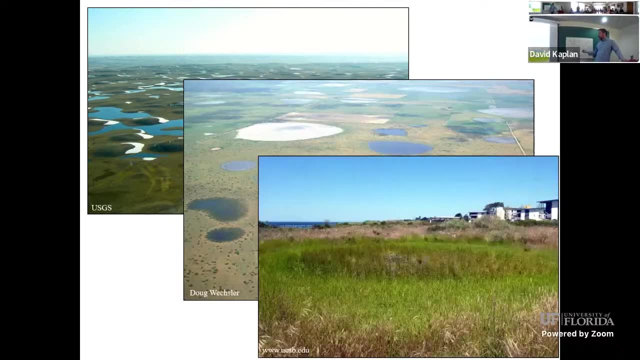 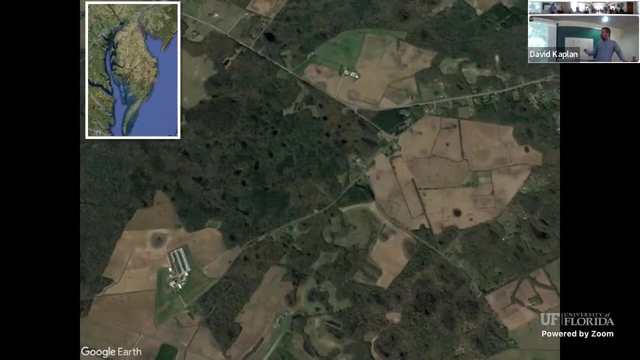 argue if those are truly wetlands or lacustrine systems. nonetheless, they're distributed water storage on the landscape. uh, Texas flyers, West Coast thermal pools and now, somewhat closer to home, not really. it still takes me six hours to get there and drive across the bay. um, what is the? 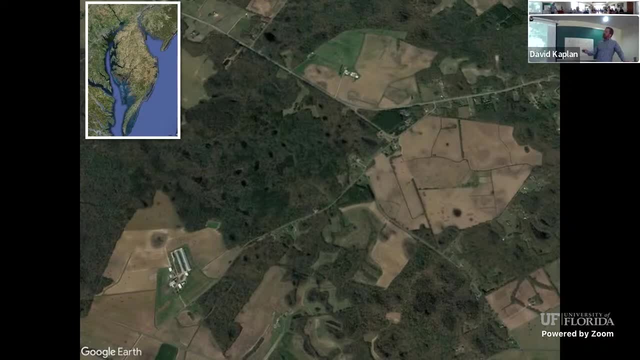 that's not it, because the middle one, um, the bay which is this really tall like eight mile bridge, which it took me a while to figure, that was called the Delmarva because, as the state of Delaware in Maryland, Virginia, and I didn't know that until I got there, which is pretty sad, um, but they also. 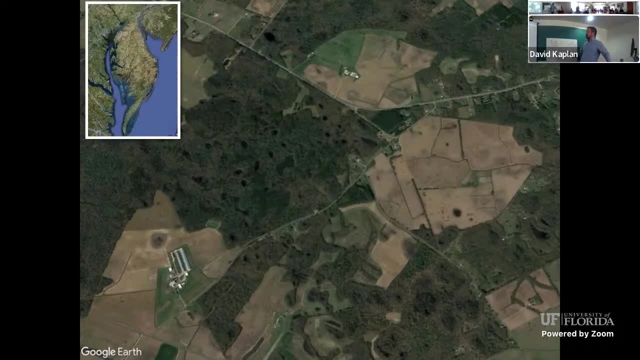 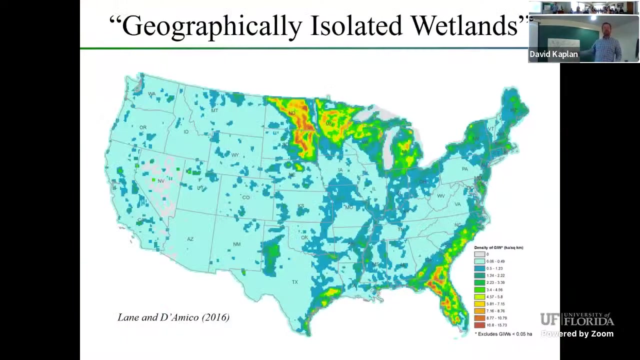 have distributed wetlands, a lot of agriculture and chicken farms and what have you, but still in big sections of existing kind of uh lands, that where you can clearly see these, what they call their Delmarva bays, another low relief, depressional, rich landscape. okay, and then you, some of you've probably 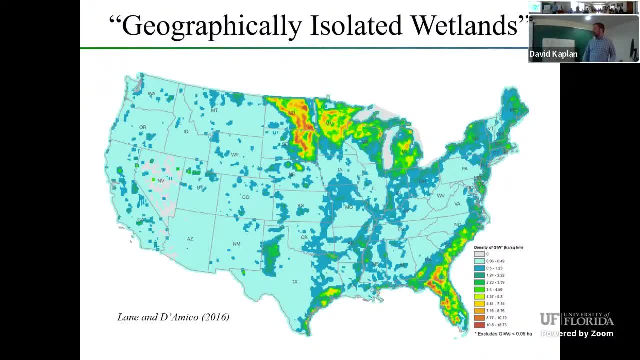 seen this map from Chuck Lane, another graduate from the program. He and his colleague Ellen made this map some time ago of the continental US, just looking at the distribution of density of these. if you want to call them geographically isolated, you want to call them non-flat plain wetlands, whatever depressional wetlands that have limited surface. 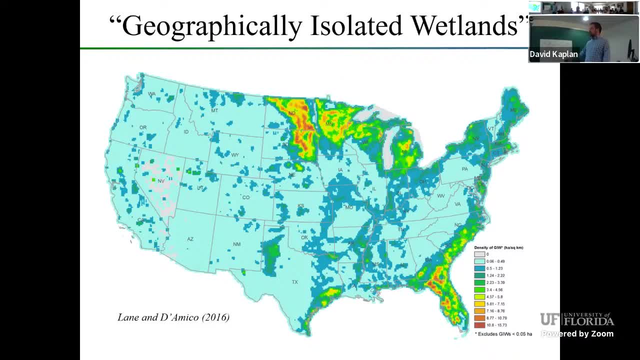 water connectivity to the rest of the drainage system. You see them dotting the prairie pothole region in the Midwest Nebraska, Sandhills, West Coast Texas Plains, even somewhat. there should be some there that are not where I live now, which is about right there And of course, a lot. 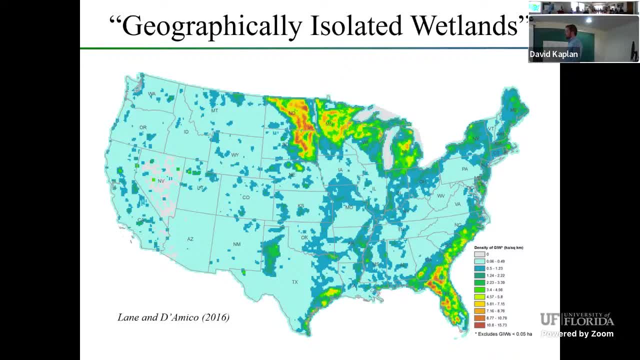 where we are today and throughout the coastal plain, And in some of those landscapes they can be small and look quite different, but they can be up to 30% of the landscape, So clearly there's some reason to want to understand what they do on that landscape, there and downstream in a landscape. 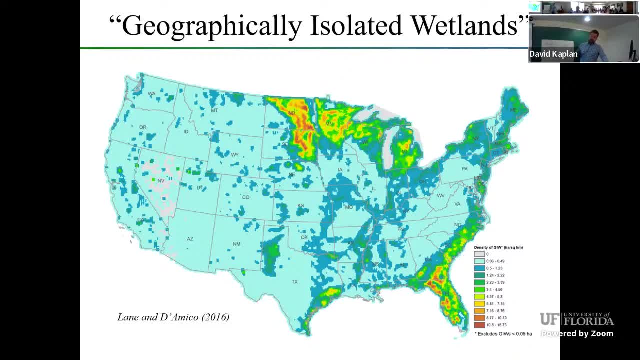 level just because they're so present and because we've lost a lot. Putting it in a policy framework around the landscape, I think it's important to understand that there are a lot of things that are not So clearly. there's some reason to want to understand what they do on that landscape, but 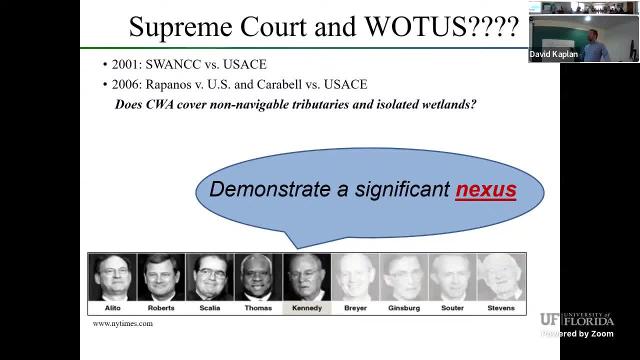 context, I should say it's even add- motivates the work even more So. before the 2000s, what is the waters of the US under the Clean Water Act and what's not was somewhat questionable. There was limited guidance from the Army Corps and the EPA. Until the 2000s, there were two. 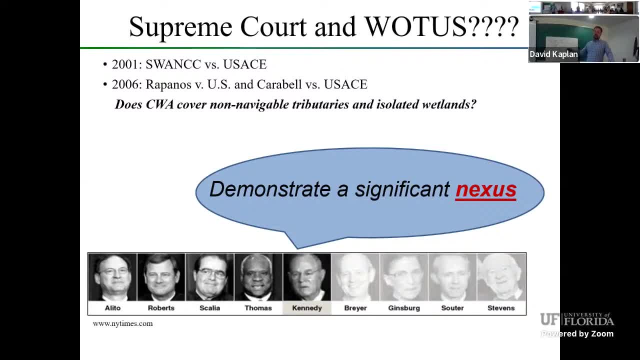 Supreme Court case rulings, which essentially questioned and debated if tributaries that don't have perennial flow and are wetlands that don't connect to what are otherwise waters of the US and navigable waters and therefore be under federal protection under our jurisdiction. for the Clean 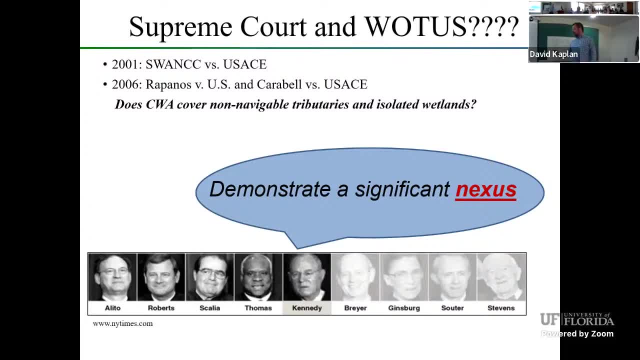 Water Act. And what came out of that question? well, Scalia said: well, they have to have a relatively permanent surface water connection, which was agreed upon. But then Kennedy, who was recently retired, came out and said: in addition, if you could see that that wetland. 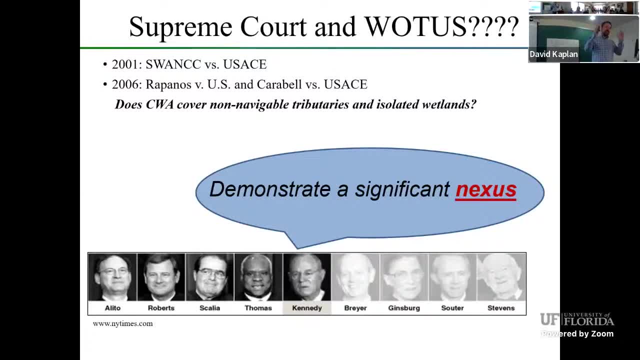 by itself or with its buddies, all those cypress stones in a similarly situated area has a significant next As to what otherwise would be considered waters of the US. I don't. I kind of think that maybe that wasn't the best choice of word nexus, because it kind of takes connection And what he meant. 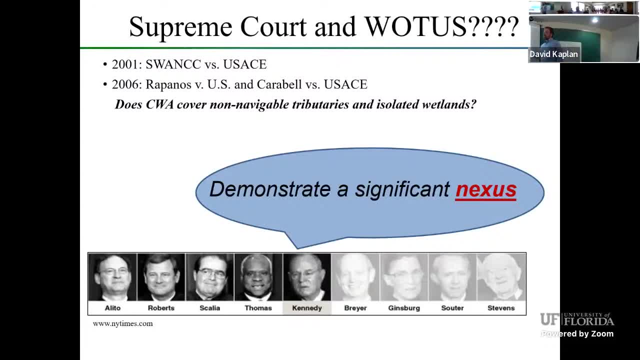 later on his comments was: was that an observable effect on the physical, biological or chemical integrity of down gradient or what otherwise now waters? And I would say effect is probably a broader term than what nexus. It's more about what it connotates, which is more about connection. So a lot of the talks and 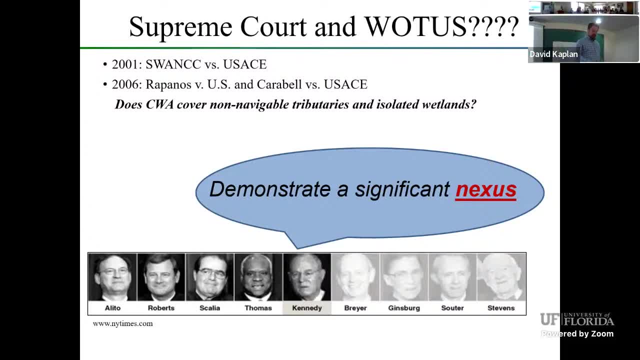 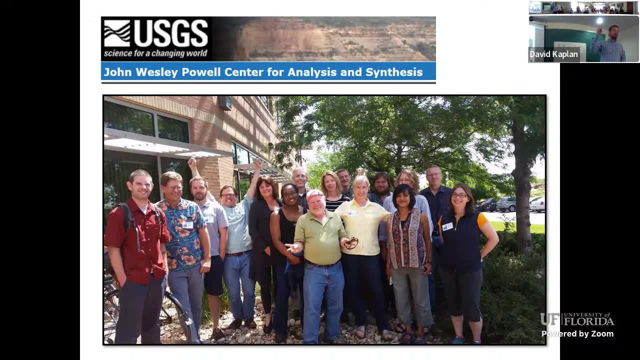 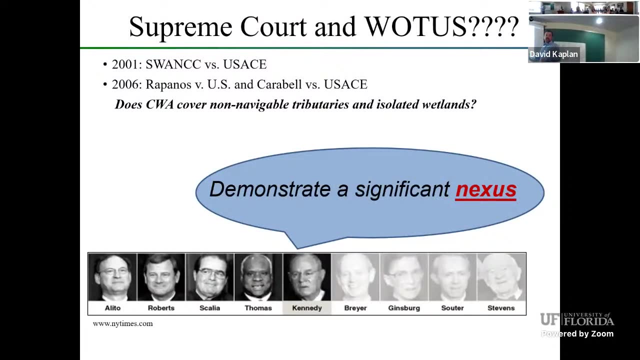 science and conferences and papers, connectivity, kind of all the day. OK, and it motivated a lot more. There was there was a special issue in wetlands in 2003 because what it said was: well, there was still some guidance to be had on. well, how would you demonstrate a significant nexus? 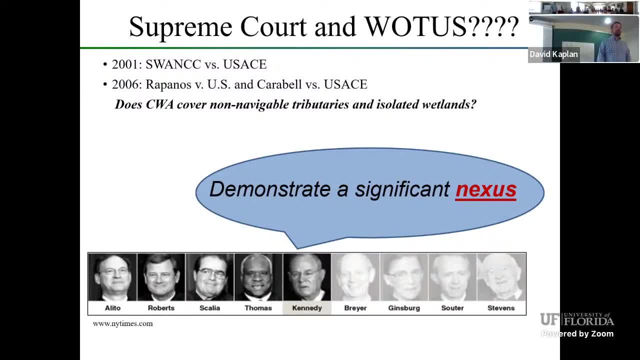 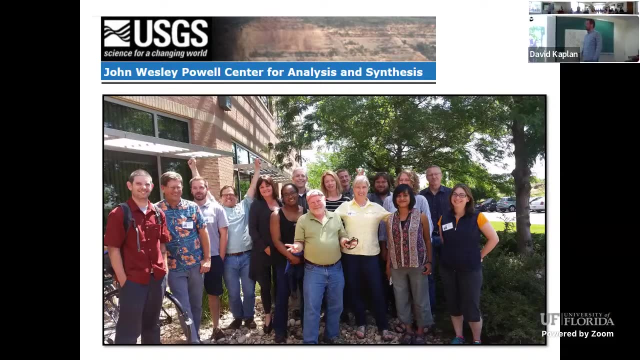 The burden is on the regulators and that's not an easy thing to do, right to demonstrate that right. But there's a lot of science to inform what has become and continues to be a conversation. So one of the things that motivated was the Powell Center group, which Chuck was first again here. 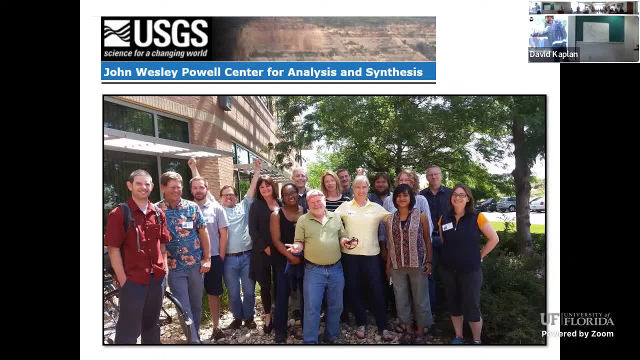 Chief scientist. Yeah, there's me with a little skinnier. So you know Mark Raines, right? That's the chief science officer for the state of Florida, right? And then some people know that guy, Yeah, wow. 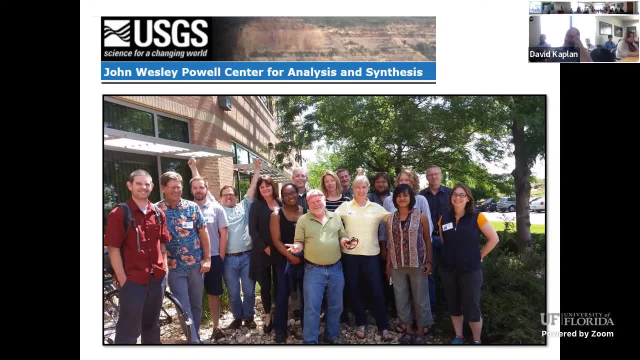 But he's funny. And then there's Larry Alexander, who was a lead on the connectivity. That guy in the very front is Scott Leibowitz, who graduated from the University of California. That's right. Yeah, we can't forget Scott, right. 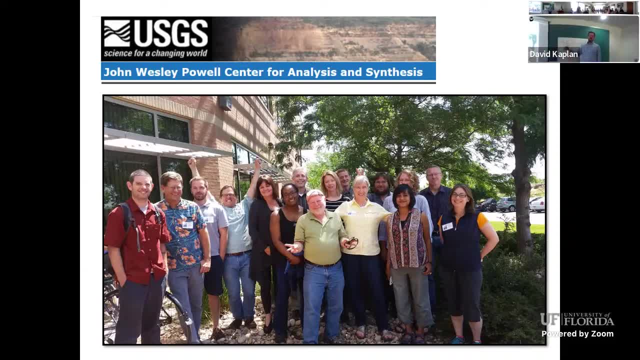 So, yeah, a great group. We ended up meeting what? three, four times in Fort Collins, which is not a bad place. They give you bikes. I think I had Alvin and Leopold's bike and we used to go to breweries and everything in terms of the court and stuff. 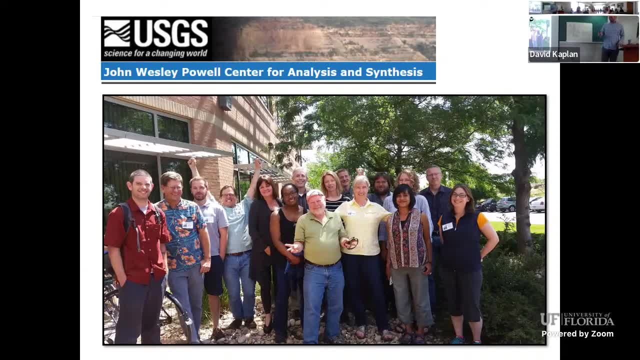 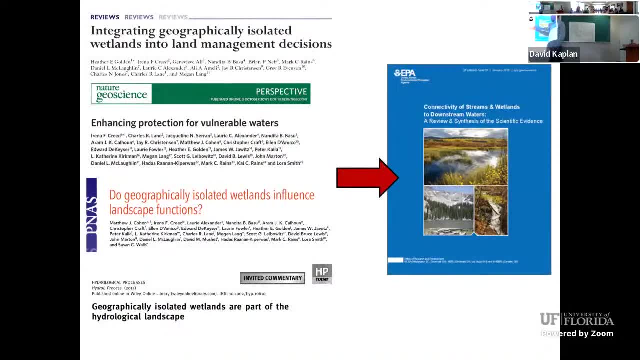 We did work, Oh and stuff in a lot of goose ship, because there's a lot of goose around this place. Yeah, Yeah, we did some work, We did a lot of work, And just not us, but a lot. of. the list of papers on this subject goes on and on and on. 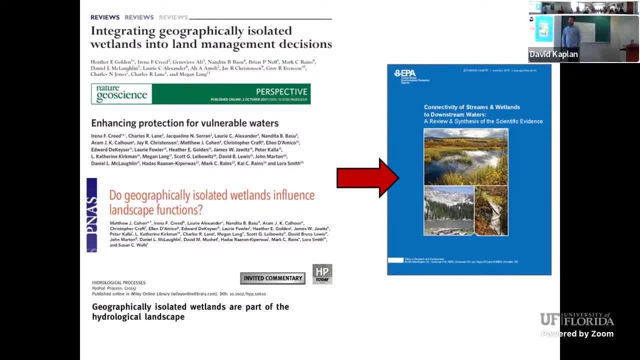 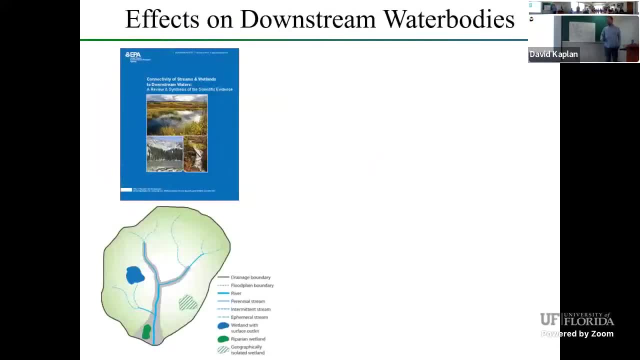 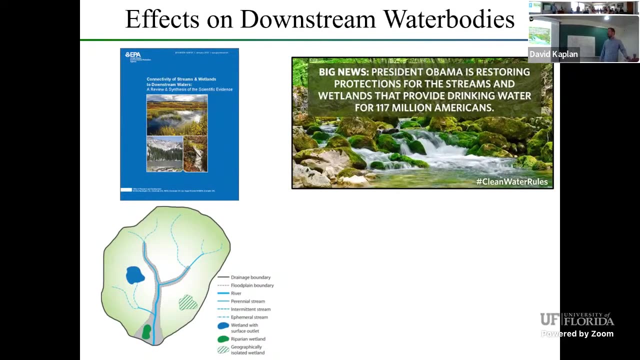 And they were subject to a review by that connectivity report with Larry Alexander, who was a good friend who led that report, which then became the precursor to the Clean Water Rule and the Obama administration, which never was enforced. It was immediately stayed in the courts. 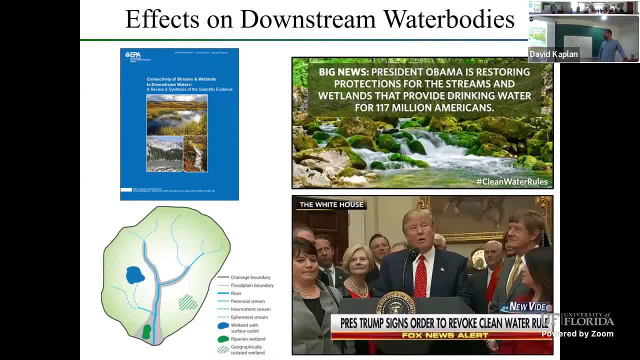 And the political pendulum swung. And then Trump revoked that and set up his own rule, which is NWPR- which I never can remember- Is it Navigable Waters Protection Rule or National Navigable Waters- And what that did was pretty much default back to Scalia, whereas the Clean Water Rule categorically extended the jurisdiction to wetlands with some adjacency and clarified these groups of special wetlands that you would figure out. 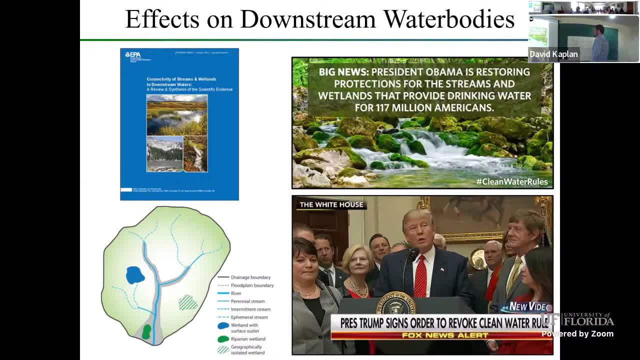 That you would address for significant nexus. So that was revoked And this administration's rule was more about Scalia saying you had to have a permanent surface water connection or relatively permanent, which of course ditched the GIWs and those types of wetlands, whatever. 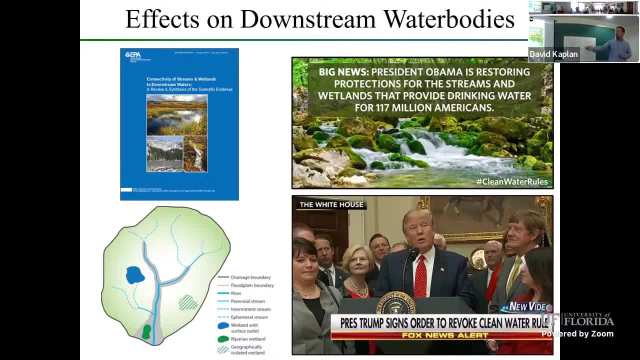 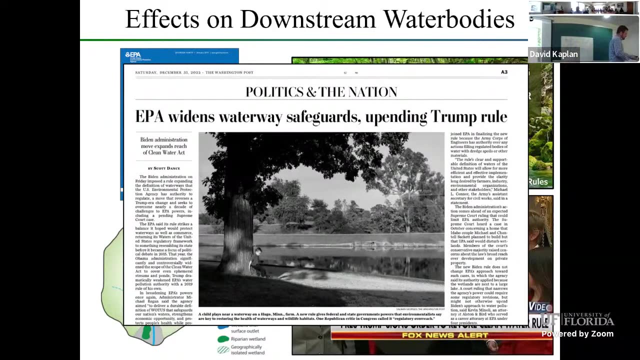 And the problem is, well, it's like ephemeral channels, right, that are in the headwaters of a lot of catchments and most catchments, including my backyard. But then this holiday break, Yeah, Yeah, Right, This December 31st, the Biden administration revoked Trump's rule, which really never played out, and went back to Obama's Clean Water Rule, more or less. 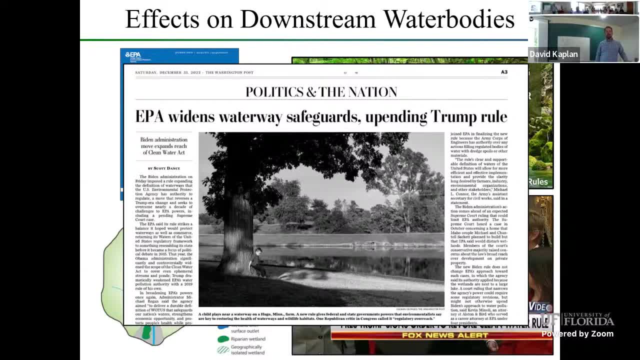 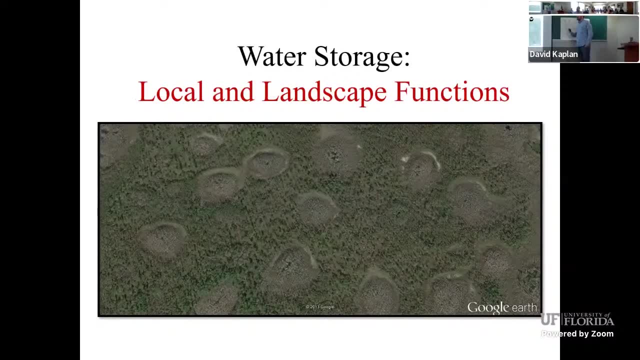 And I'm sure that this will keep on going this way, which is unfortunate, But nonetheless, one motivation- not all motivation- to understand these systems. They're important landscape elements on their own. Okay, So that's what I want to talk about today is just to give you again just kind of a broad sweep of things. 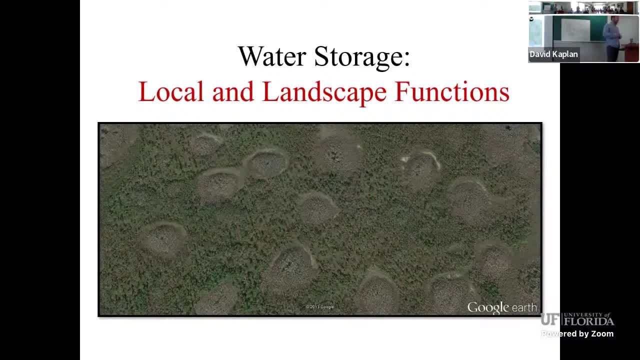 A broad sweep of the type of work that we collectively have been doing on this topic, Thinking about distributed water storage, I mean, I think that's one of the names of the. you know really one of the things that these little wetlands do, by definition, right. 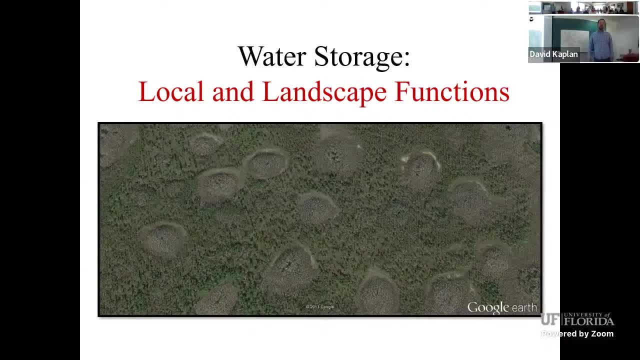 Limited surface water connectivity probably means they're increasing the sponginess of the landscape And that can mean something at local scales for functions. But of course, when you have a lot of them, landscape functions. And I want to kind of do it in three threads. 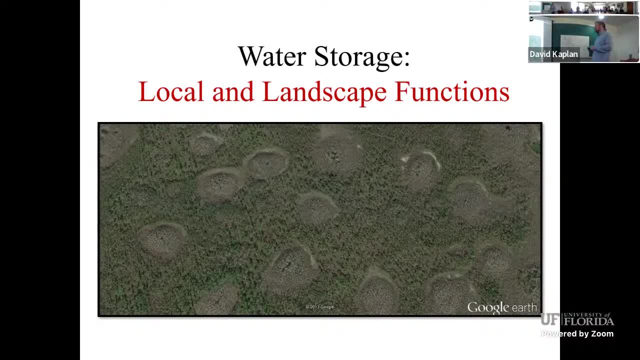 One is the clear one: hydrological functions, But also what it might mean for biogeochemistry, Carbon specifically, Some new work there And by OTA, which I've had, actual, some fun playing with critters- Not really for me playing with them, but anyway. 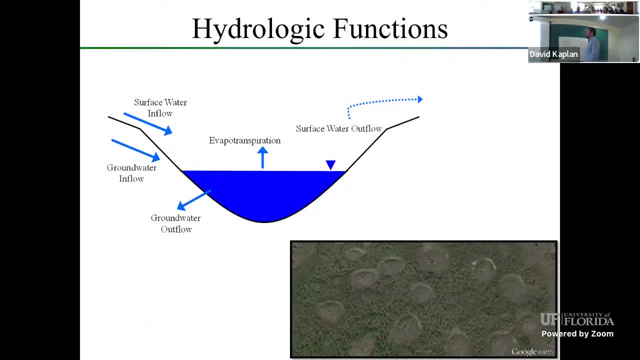 All right, So we'll start with hydrologic functions. I'm not going to talk about Coca-Cola and specific yield, But just nonetheless. you imagine these wetlands dotting the landscape They take in water: ground water flow, surface water flow. 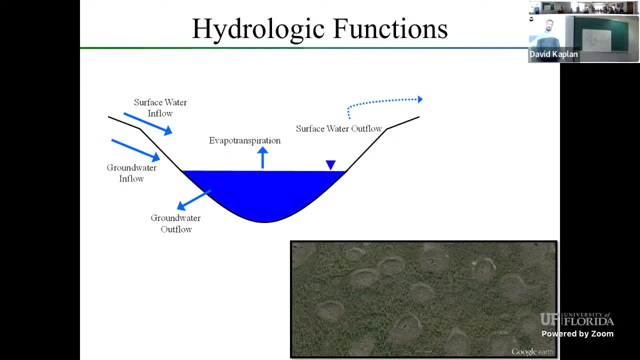 This is pretty limited. They might leave the lot this way And they might return some of that water, And so we wanted to. Matt and I and others wanted to ask the question- in addition to some other topics related to that project which I'm not going to go over, this kind of groundwater exchange deal. 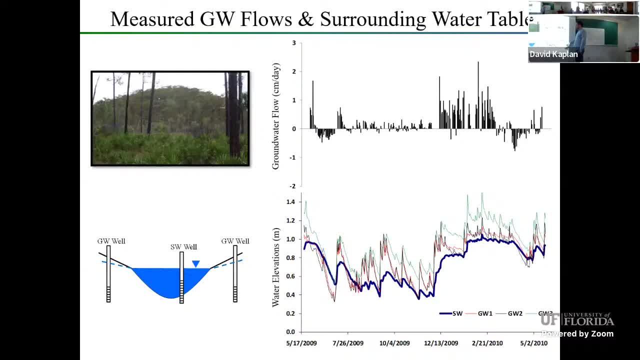 And what we found when we were in the field. and this is a dated figure, sure, clearly, but it tells a story, right. So down here is just one wetland here, Two groundwater wells around it. There's actually three. 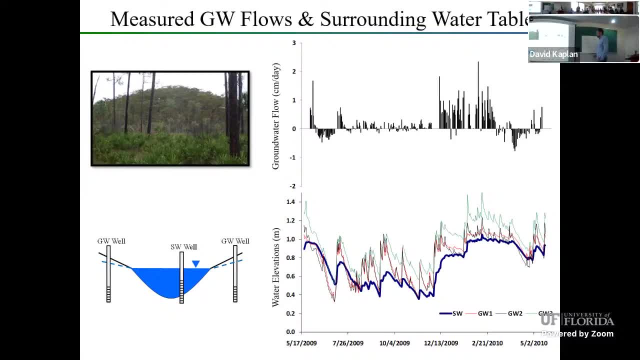 And then the dark blue on the time series On your left or, excuse me, right, is the water level in that wetland, that surface water? well, And these light lines are the elevation right, This dash line relative to that dark blue line. 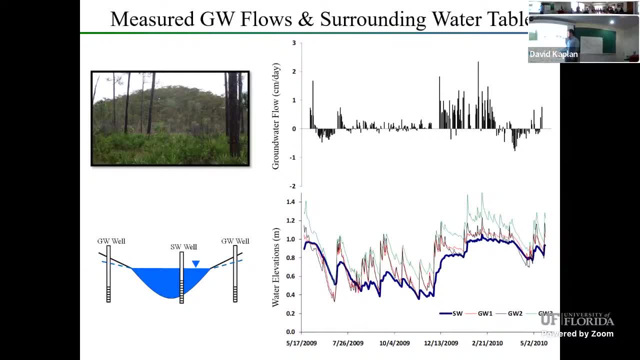 And you can see over time it goes around it, Meaning that sometimes the groundwater around it is lower and sometimes it's higher, And you can kind of mark that with dry periods of time and wet periods of time, And we can calculate those flows in different ways. 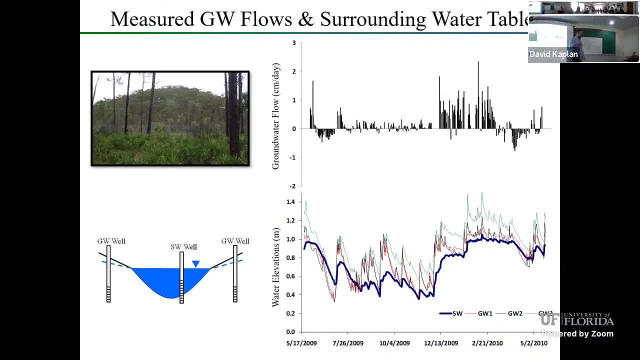 But the point is that they switch in terms of that wetland, That wetland receiving water, particularly during wet times, And then re-releasing that water, particularly during dry times. So we saw that in the field and we said, all right, well, that's pretty cool. 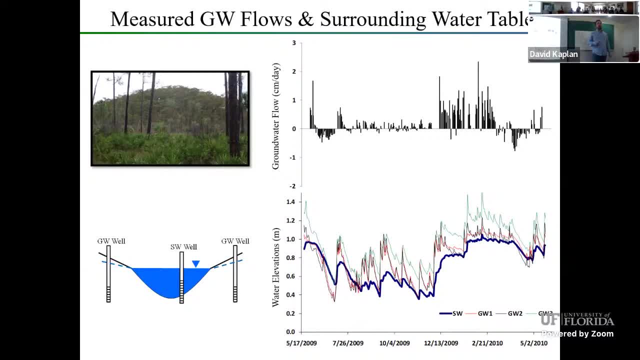 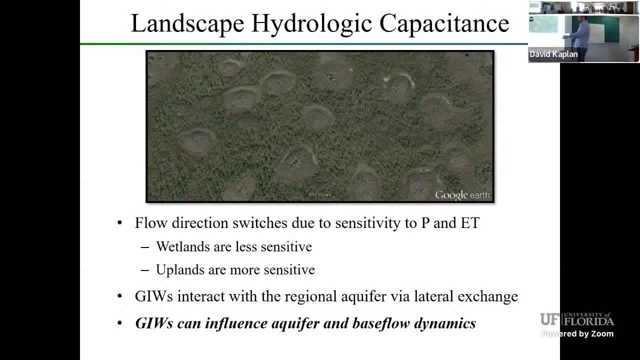 What does it mean? We can see what it might mean at local scales, But we wanted to think about what it meant at landscape scales and why this is occurring, And that's where I would talk about specific yield and all that, But I won't, just for the sake of today. 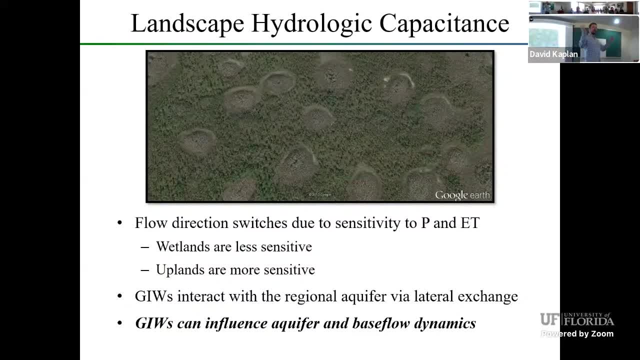 The point is, wetlands are less sensitive to precipitation events. The water level doesn't go up as much With that same precipitation event in the upland, Because the upland soils have displacement from soil particles, Whereas the same thing goes on with vapor transpiration. 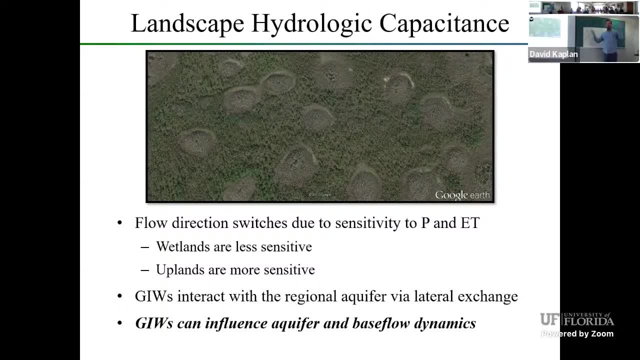 You're going to lose that water, pretty much that right depth of, let's say, 5 millimeters of the vapor transpiration. But that 5 millimeters in the upland might make a much bigger drop in the water table Because essentially you're taking water out of a cup with ice. 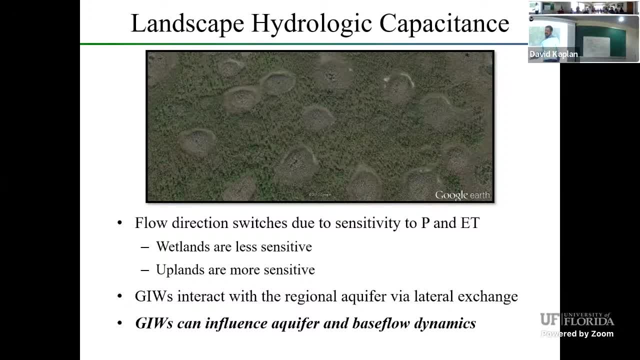 So the point is: uplands are more sensitive, wetlands are less sensitive And that switches hydrologically. It's where they can have the sink function during wet events and source function during dry events. And the question is: well, this guy is doing it. 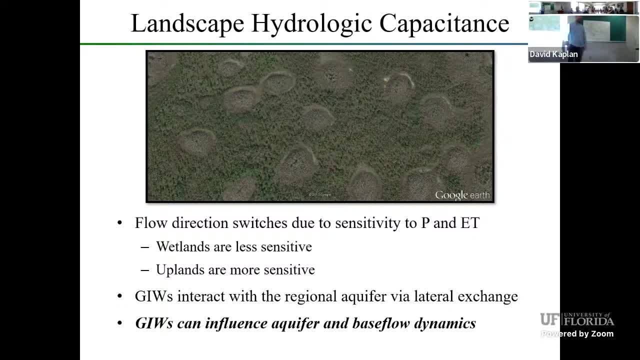 This individual is doing it. They're doing it At that scale. But if you have all that perimeter for exchange across the landscape, what does it mean for the ups and downs of the water level below this landscape And, of course, the ups and downs of that regional water table? it influences downstream base flows to nourishing. 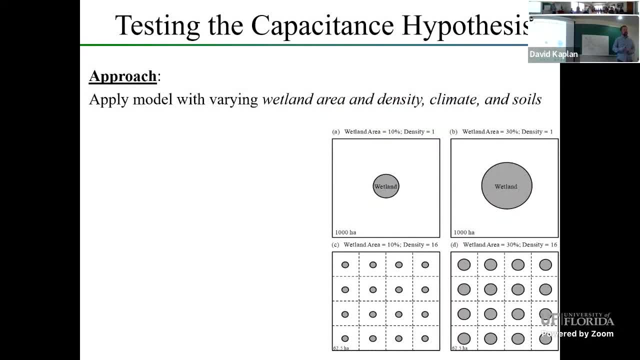 And so we had to bring David Kaplan on this question just to ask this question. with our model conceptualized but very much process-based, where we're representing each individual wetland and its back and forth with groundwater, to say, let's put a lot of those wetlands on small, a lot of bigger wetlands or maybe just one big wetland and manipulate area, wetlands, density of wetlands, a lot of small wetlands and a few big wetlands, manipulate climate, manipulate soil. 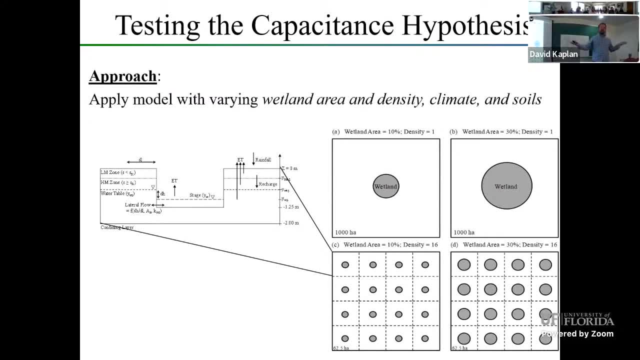 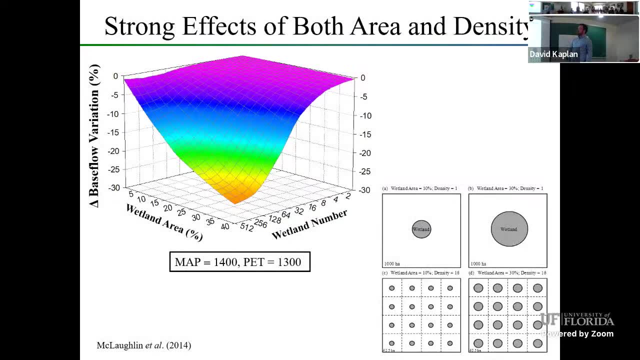 all in a generic landscape, a fake landscape. That's what our landscape looked like And we did a bunch with it. but for now this is it on it, where we have a certain potential of, after transpiration, a particular mean annual precipitation as we model those things, and so on and so forth. 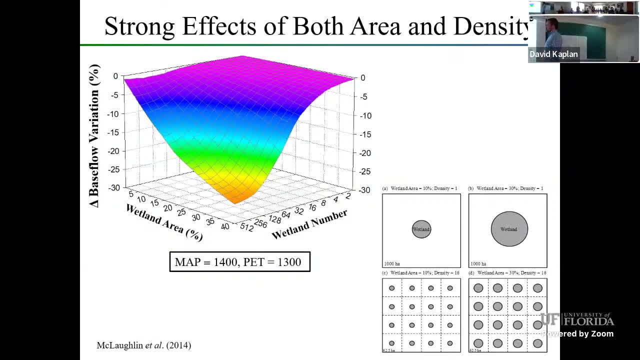 But for this particular climate, which is somewhere near where we are, we can manipulate wetland number on this axis, wetland area on this. So right here we have a lot of wetland area spread across a lot of little wetlands, right. 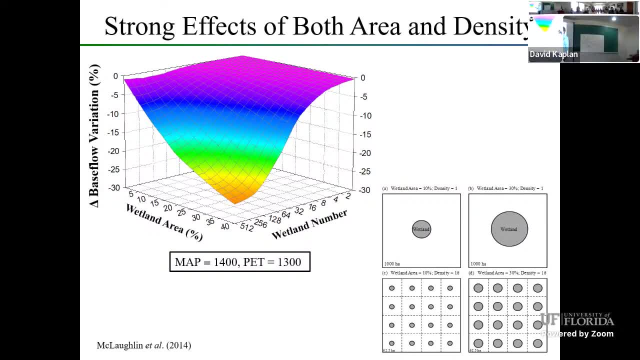 And right here we have a lot of wetland area spread across two wetlands and our y-axis response variable is the change in baseflow variation, And you see that they're negative. particularly, this thing starts sloping down when we get a lot of little wetlands, meaning that we've reduced the ups and downs of baseflow that comes out of that landscape by up to 30%. 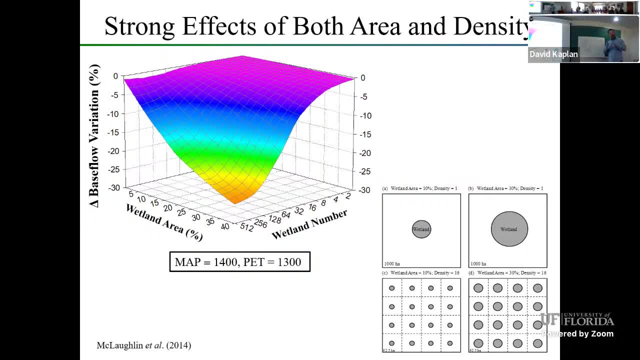 So an indirect, And that water may never make it from that wetland to that stream, but it's the back and forth of these wetlands that might come past it, as is what we like to call them. And one key point is that if we take this same wetland area but distribute it over one big wetland, we lose this function. 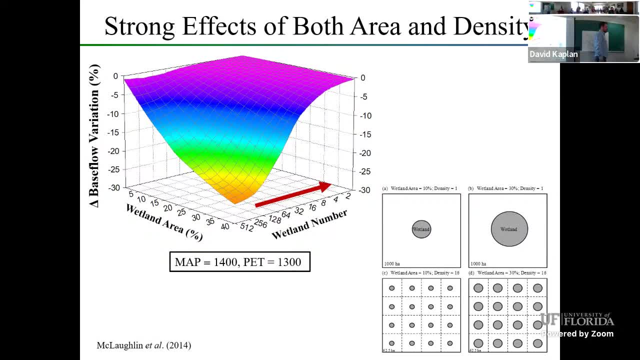 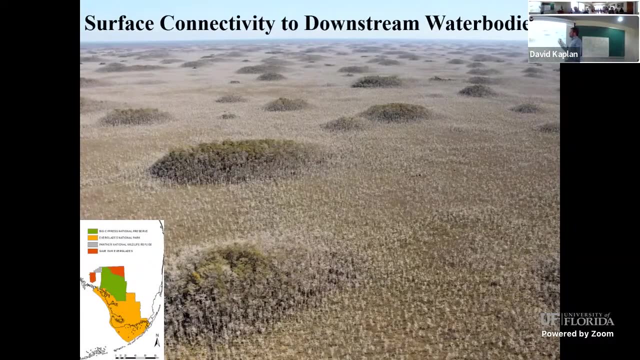 It goes back to zero And that might speak to mitigation and taking a bunch of little wetland functions and putting them in the corner of the landscape, But that might be a conversation for another day. Okay, So more recently, back to that beautiful image of Big Cypress on the ground measures. we're working with Matt and colleagues. 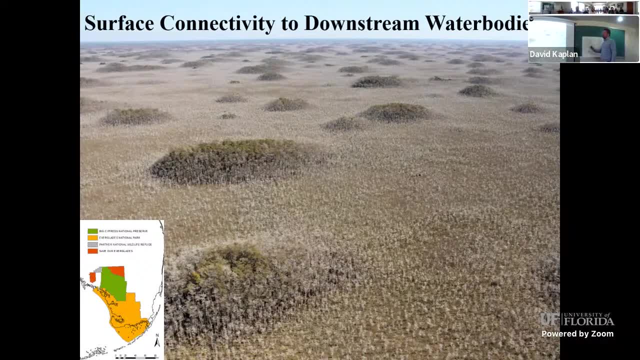 We did a lot of stuff on testing a hypothesis about how these wetlands actually came to be and their patterning, But one of the things that we did was we monitored how often they would connect via surface water. Indeed, they do, even though most times, or a lot of times, you can keep your feet dry. 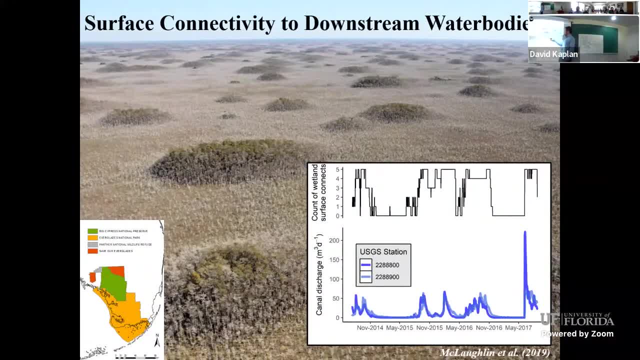 And what that actually means for downstream baseflow. And so this little squiggly line goes up. That means a lot more wetlands are connected. You can splash between them And, as they do in synchrony, you see, that creates very episodic downstream gauges. 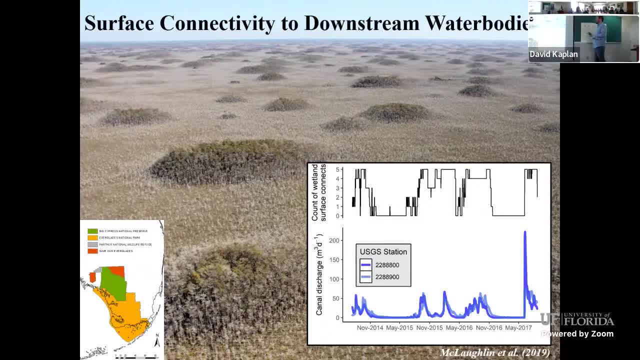 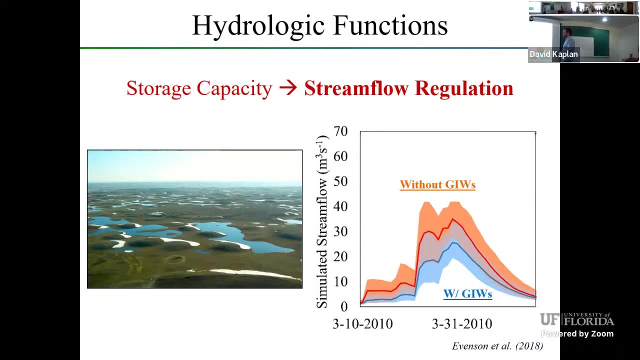 So again, both models to look at this question from a subsurface perspective, empirical observations to think about it, and surface water connectivity and what that might mean for downstream waters. Moving to the prairie pothole, asking the same question, but at a bigger landscape and with a different model. 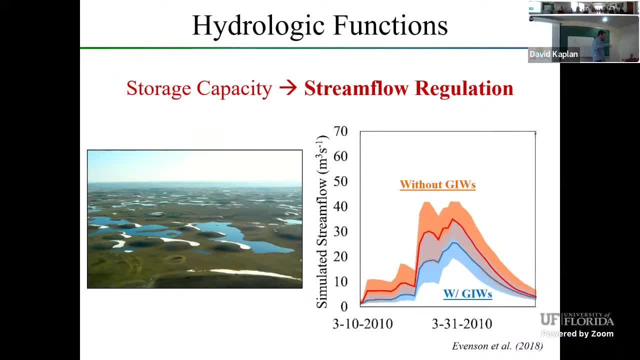 Chuck Lane, Heather Goldman- there postdoc who then became my postdoc, Greg Evanson, working on a refined SWAT model. Some of you probably heard of the SWAT model. It's just a model out there where you can represent different landscape elements. 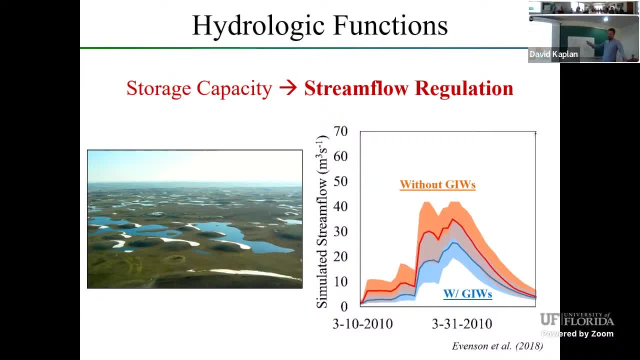 And he worked to more explicitly represent individual wetlands as their own kind of HRU or own kind of model component. And we could play games again about putting GIWs or these prairie potholes in, taking them out And see what they do to the stream soil. 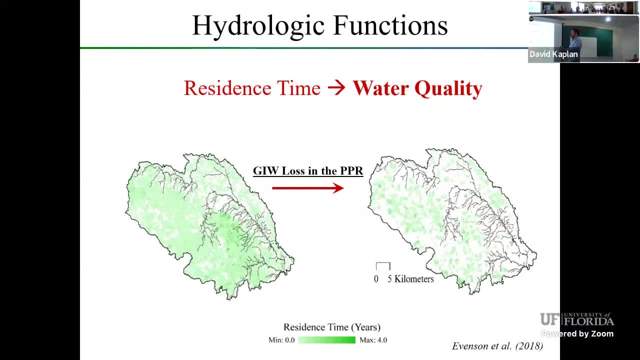 Storage capacity also clearly holds water back into the landscape and water into the watershed Right And more residence time. We can definitely think about what residence time, how long that water sits there, in terms of what that might mean for carbon processing, nutrient removal, sediment removal and so on. 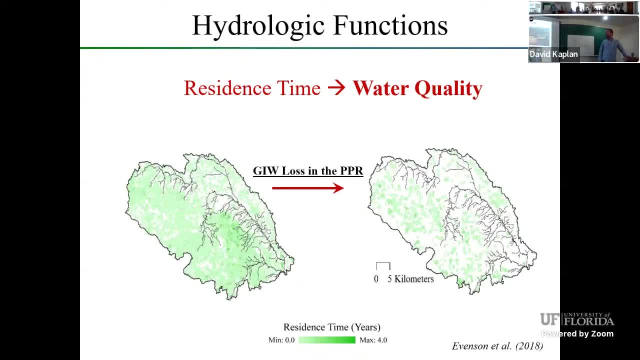 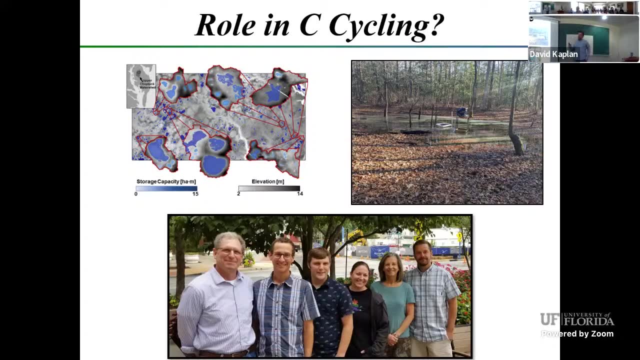 And that, which is a nice segue to think about some more recent work More explicitly on connecting now into this biogeochemical thread the hydrologic effects in that water storage and carbon cycling. So this is some work that I was lucky enough to continue working with Nate Jones, who was a postdoc with me and then came as a postdoc with Margaret Palmer at UMD. 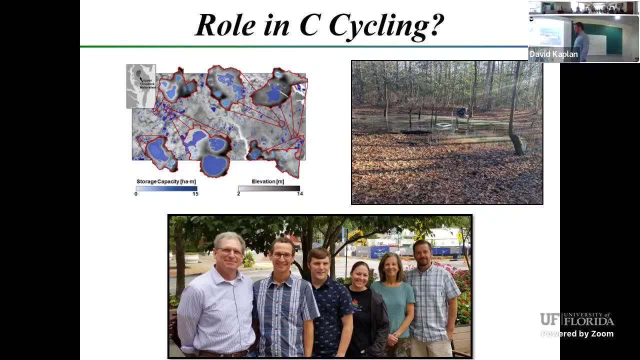 And now he's faculty at the University of Alabama, Colleagues of mine at Virginia Tech, Aaron Hotchkiss and Darrell Scott, And it's a great group to work with And we're continuing to work on it And we have a lot of questions and hypotheses. and now we're back in the Delmarva Peninsula and Delmarva bays. 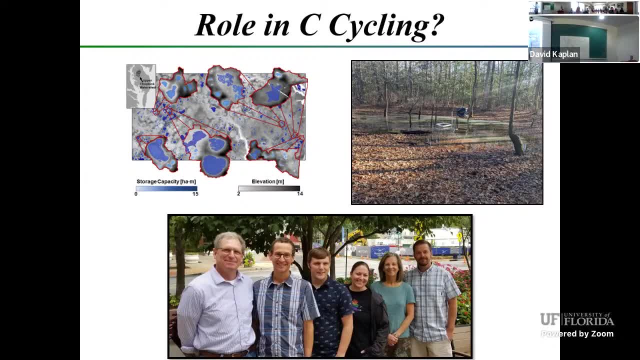 We've been there, we've seen it right through on this inset. But what I'm trying to call attention to here is all of these wetlands right Where Nate, with really good topographic lidar data, was able to calculate potential storage capacity. 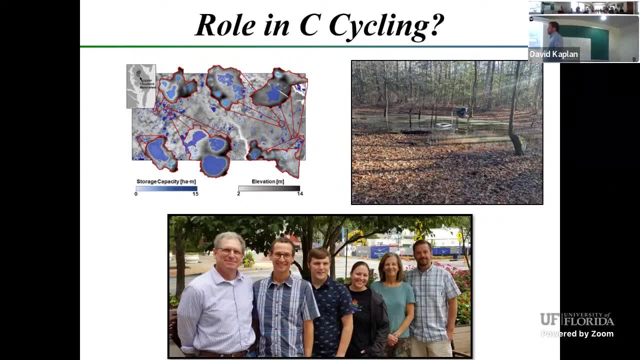 Some wetlands have a lot more storage capacity than others And we had some hypotheses of what that meant for CO2 emissions- Not just for the water emissions, methane emissions, DOC processing dissolved organic carbon and export dissolved organic carbon as well as dissolved inorganic carbon out of this thing. But right now we're 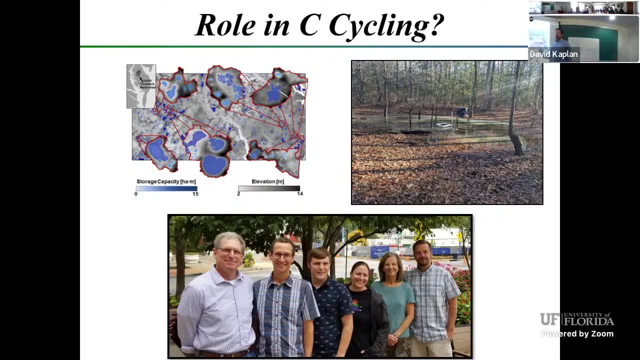 thinking about just individual wetlands. We put a bunch of sensors out there. We have dissolved oxygen sensors distributed across our wetlands, FDOM or dissolved organic matter. We have CO2 sensors which now they don't make anymore, And that's another story. Clearly, pressure 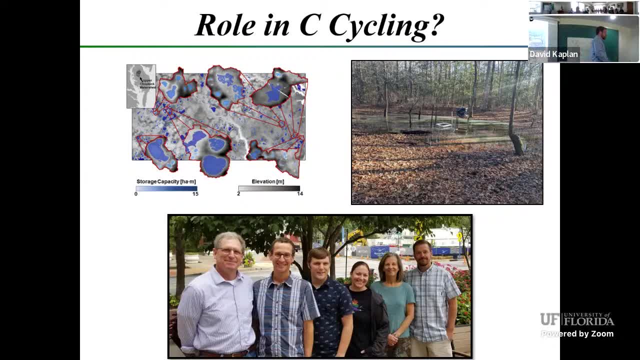 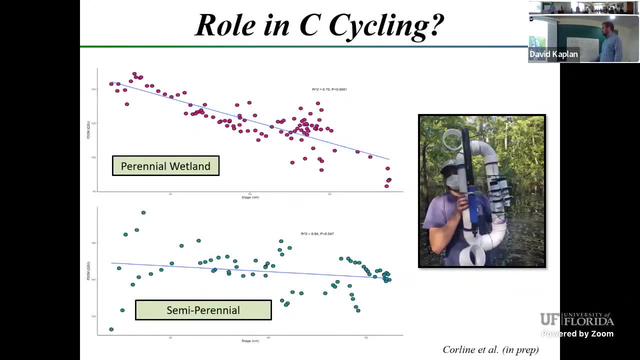 transducers to measure groundwater and water levels and emission chambers and a lot going on there. And we have a board of students on the project, One of which is my student, Nick. This is kind of hot off the press. I'm sorry for his units or the labels there. It's hard to see. So 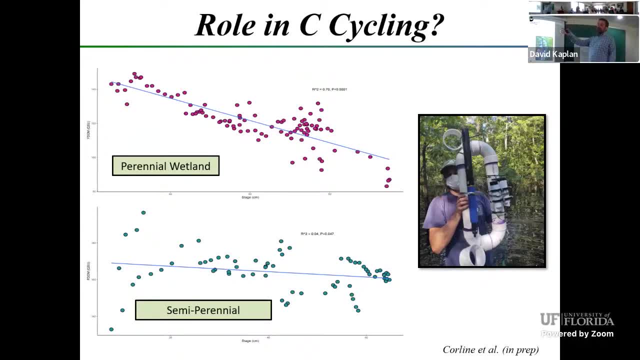 I'll just tell you what they are. This is FDOM, just dissolved organic carbon, kind of That's not necessarily one. And then this is water level. This is James Mays, not Nick Forlan, who is the best technician you? 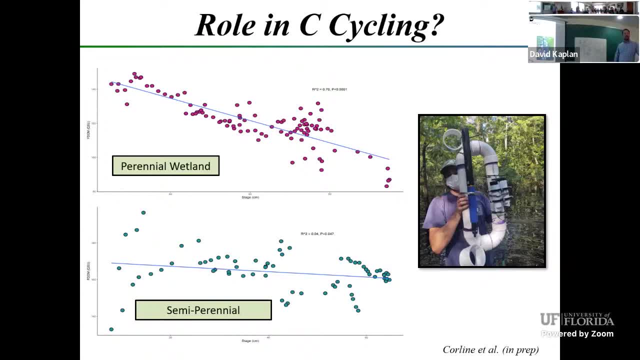 could ever have, who was nice enough to move out to the eastern shore and live out in the middle of nowhere so that he would be close to the field sites, because these sensors require a lot of TLC. So he does it like every 10 days And he recently now has gone to graduate school, which is good. 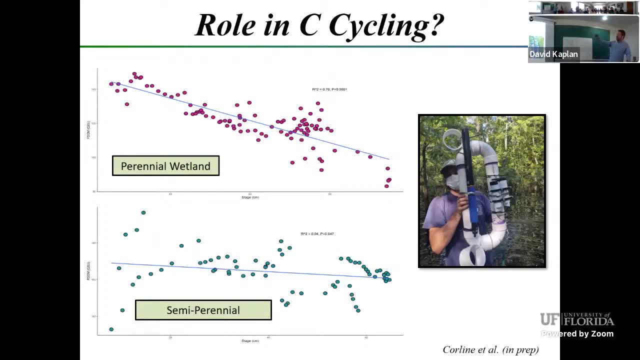 for him and bad for us. So that was the thing that would float, you know, on this kind of T-pose, so that it would always stay 10 centimeters relative to the top of the water, right, If we fixed it, sometimes it would dry out, or sometimes it would be telling me something about the bottom. 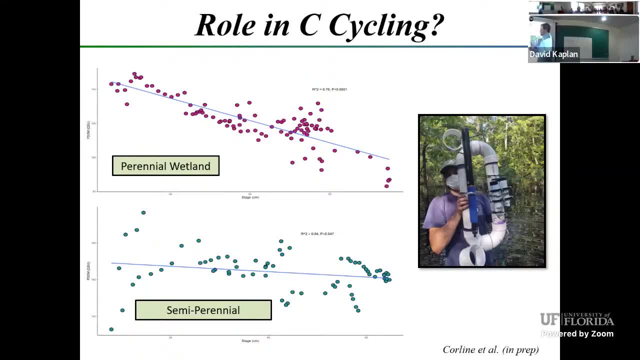 of the water, top of the water and what would be the system. So this wetland, he's calling it perennial wetland. The point is it never dries out. So this is: just think about it as kind of dissolved carbon concentration, kind of versus stage. This wetland never dries out, But more. 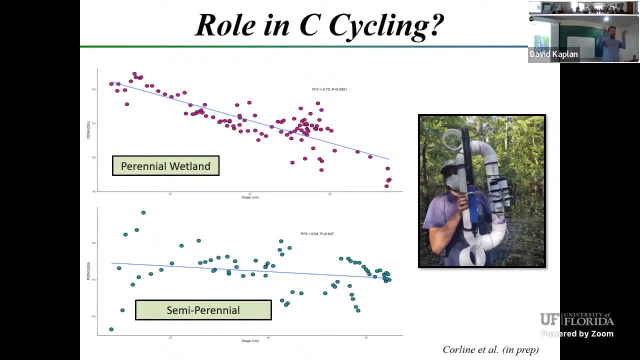 important. I probably should have had some figures in here to explain this, but its bathymetry or its topography is like that, Really steep slopes like, almost like a cylinder, meaning that when it dries down or when it wets up, 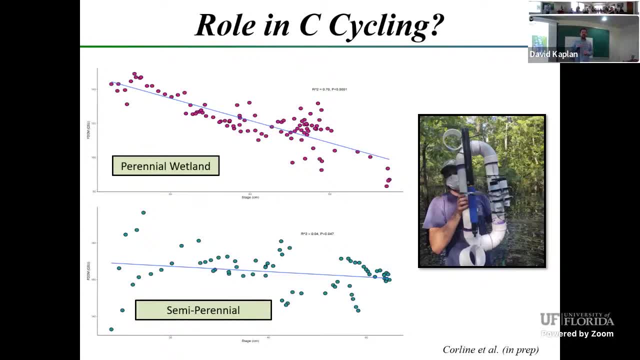 it gets deep, pretty deep, over a meter chest deep in some places, But you don't get much more flooded area right because of that steep slope. A little bit of water level change isn't going to inundate that much more soil, right, And we see that. as that happens, we get a dilution effect. 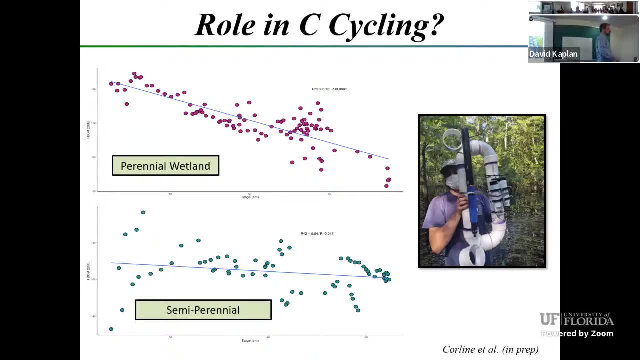 which might be predictable, right? Because you're just getting more water to dilute the source of that dissolved carbon, which is from litter breakdown and extractable from the soils. Whereas this wetland does dry down, Of course, we don't have concentrations when this dries, There's still. 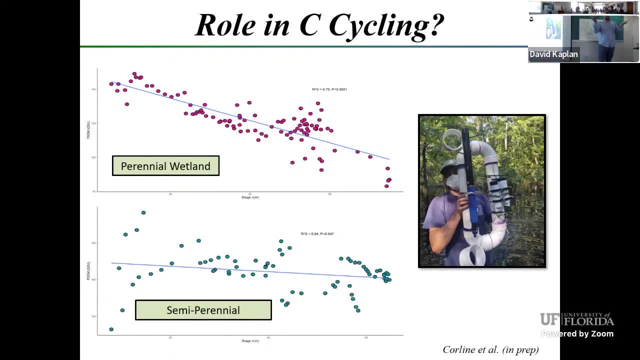 zero there, But its bathymetry is more like this. So when that water level goes up and down, it inundates a lot more area, And what I want Nick to do is to convert this stage to flooded area using some topographic data. I think he just hasn't got there. 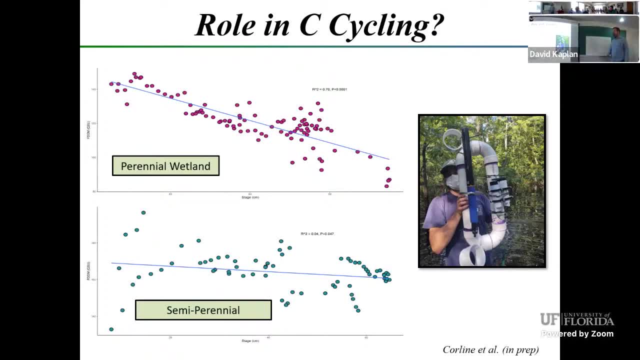 My guess is that our guess is that that might be an explanatory factor, because that dilution effect is obscured as that thing gets wetter, because it's flooding. you know organic rich soils much more because it's within the tree. So something about a local topography. even these two wetlands are 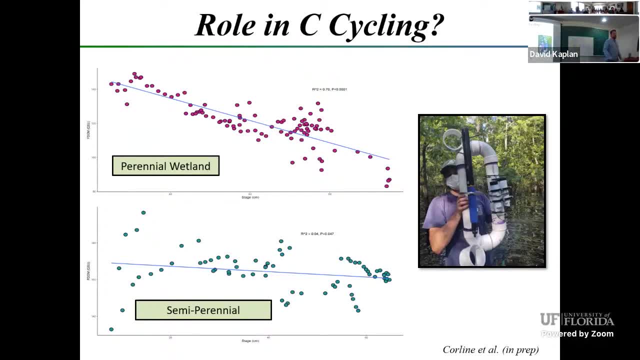 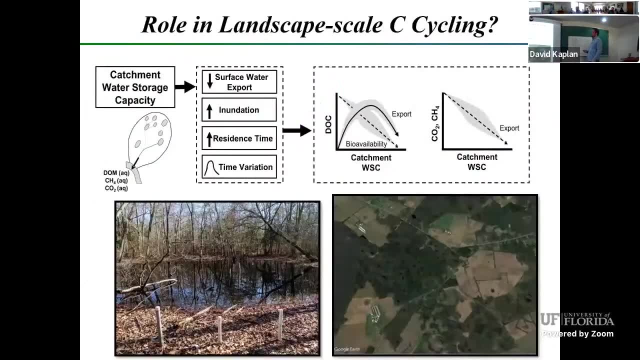 50 meters apart, but they're quite different, And how they generate DOC wherever it goes, or fuels emission can be different. But also want to do this at the landscape scale. So there's a lot of these little wetlands across our landscape. 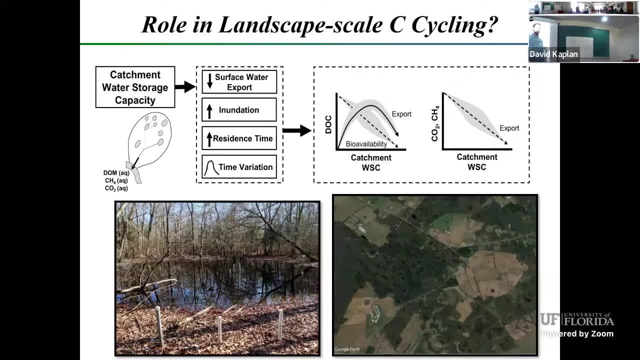 They connect, as Matt likes to call them, like a string of pearls right where there's a lot of these little wetlands And you could at times kind of splash your way through these little intermittent or ephemeral channels. And we had some predictions about how the catchment water storage, the cumulative storage of all these little 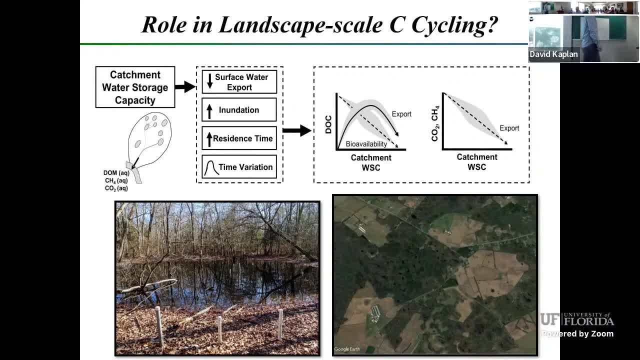 wetlands at that catchment or watershed scale influenced these little little water sources. Right is things like: as you increase that you should probably have less surface water export. you should probably have more inundation or flooding. should i have more residence time and it probably could. 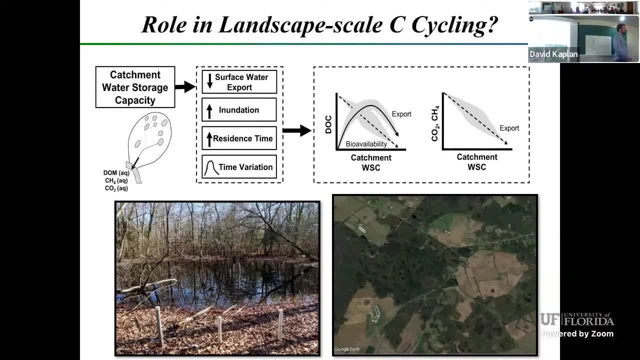 do something to the variability of those things. and we then say, well, what does that mean for carbon? because these things relate to how available carbon is. when we predicted that if you hold the water back that stuff gets more processed, less bioavailable export we predicted might have some. 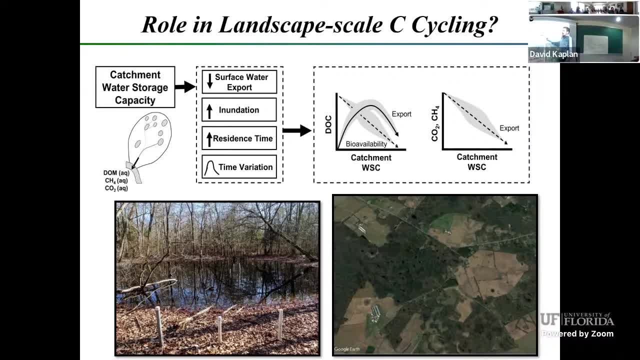 kind of intermediate effect, where we don't have any storage capacity, you don't hold water back long enough to generate doc. right, if you have a lot of storage capacity where you never export, so maybe some sweet spot. and then in terms of exploitive disc, we had some predictions there. 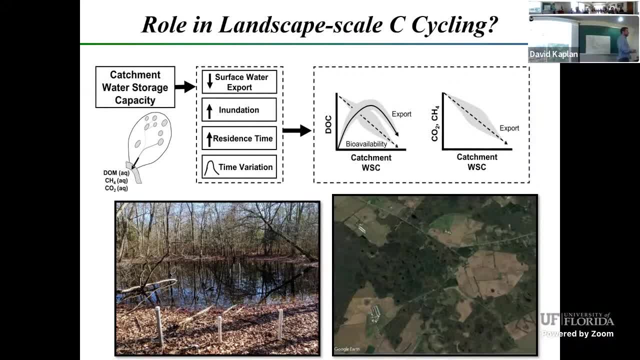 again, i'm not going to go into the findings because this work's ongoing, but just to kind of give you an idea how we're trying to connect things we know about hydrology, health, topography influences those things, as well as other drivers and what that might mean for carbon dynamics. 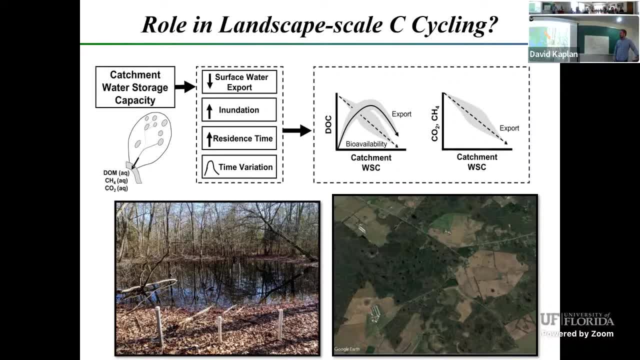 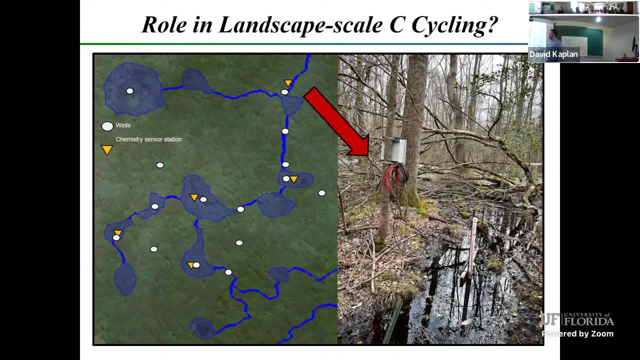 et cetera, local and landscape scales. um, from the export perspective, here is one of those channels exporting from our string of pearls and we have also censored there. here is kind of i should switch this because somebody could ignore it, but i still want to think about it as a watershed here. 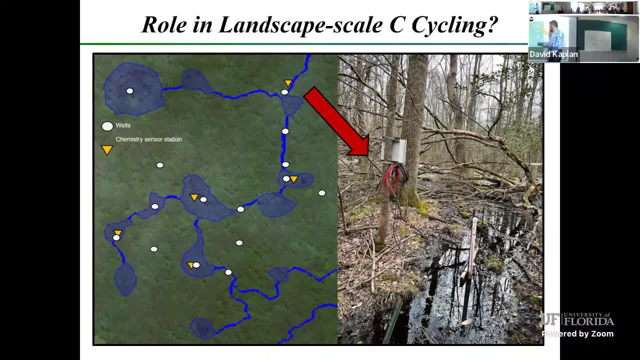 our headwater weapons right and they kind of connect. at times we have a mixing bowl we call. we have all kinds of different names and then eventually it comes out after it connects with this individual weapon and they all look different. some have have a lot more of more of these спares. they're planks, seeds. they call these stems of compassion, re石. 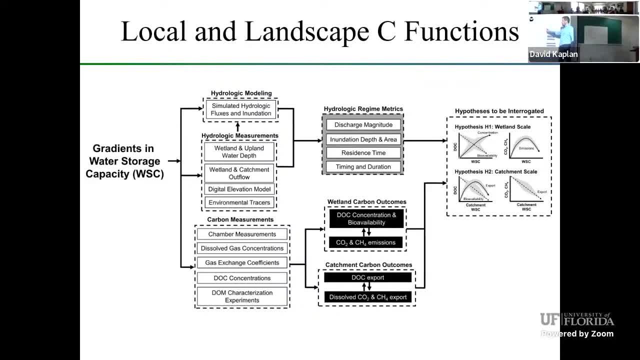 create ears. so to put it all together and ask questions, this is a lot. that is this the way we're thinking about things: logic measurements, modeling a lot of carbon measurements to try to think about the outcomes For carbon. it's the metrics from hydrology. 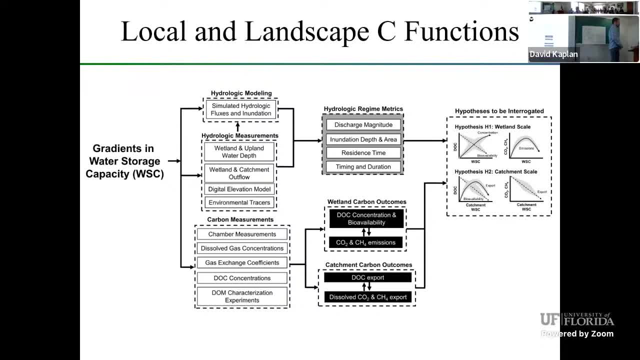 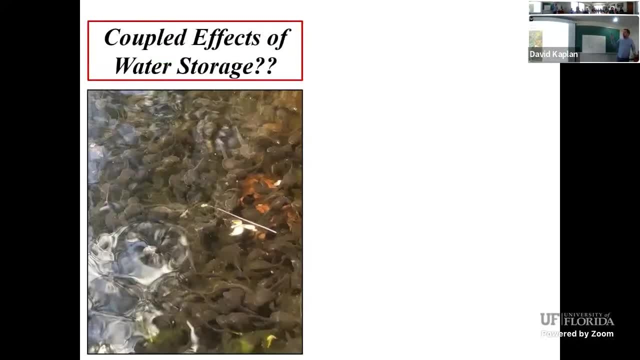 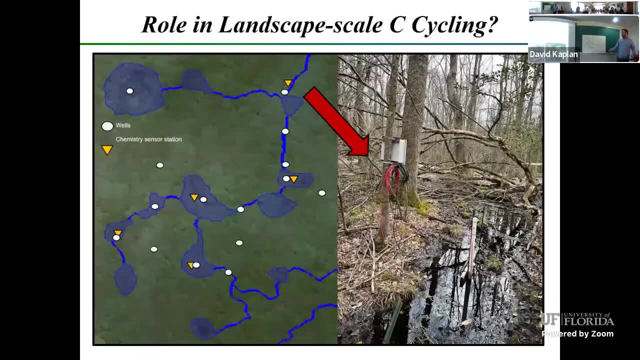 so we can ask our questions and test our hypotheses, But again, I don't have these findings that this work is ongoing. Now I'm gonna use this as a segue and this may be an aside, but Nick, my student, who's supposed to be doing this? 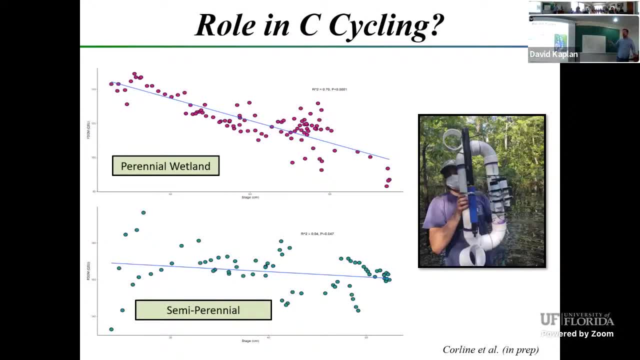 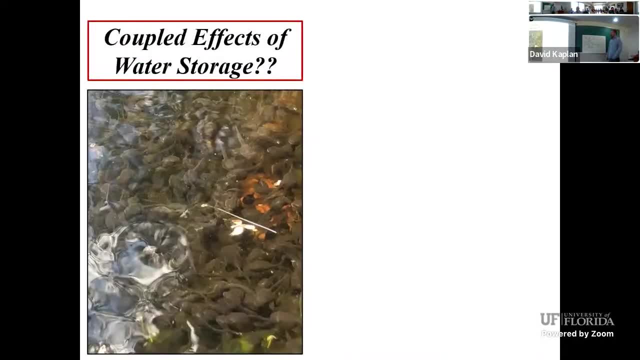 had got his master's and practiced as a community ecologist for some time, And so I can't get him away from the critters, And so when he was walking out there on the wetlands, he noticed this: a huge, huge map. 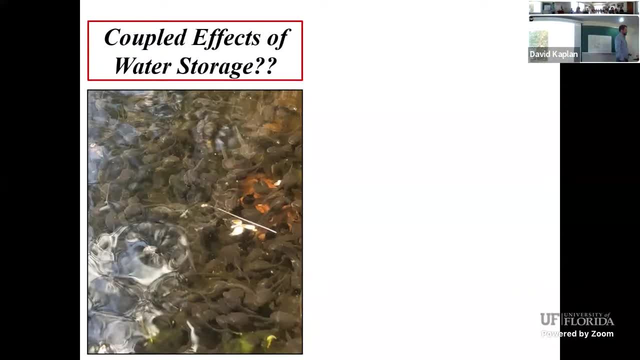 covering one of those wetlands surfaces- wood, frog, tadpoles, And so this might seem like an aside, but I'm gonna use it as a segue. but also, I don't think it is Like it's that water storage that made it attractive. 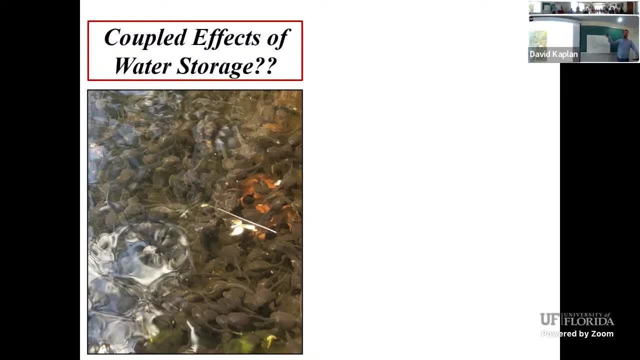 for these frogs to lay their eggs. where there's limited connectivity between waters with dish predators, It's a good refuge. It's a good place to set down your eggs and let these things do their thing and become frogs to do it again next time. 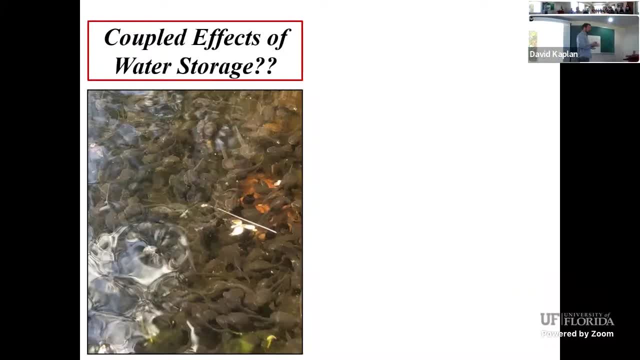 So it's this distributed wetland, smothered across this landscape, that is supporting this population. That's the biologic. that's obviously an effect of biota, But I'm gonna stick with it here around carbon, because that could be an indirect effect. 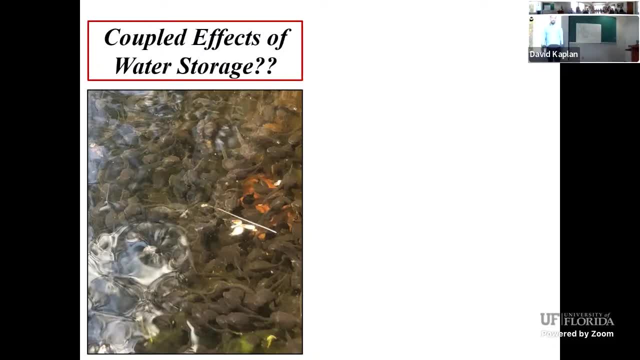 And this is what what Nick had proposed- is that these guys have to be doing something to change carbon dynamics. They're directly munching on the litter, for sure, right, But there's also they're excreting nutrients, And so there's all literature in other fields. 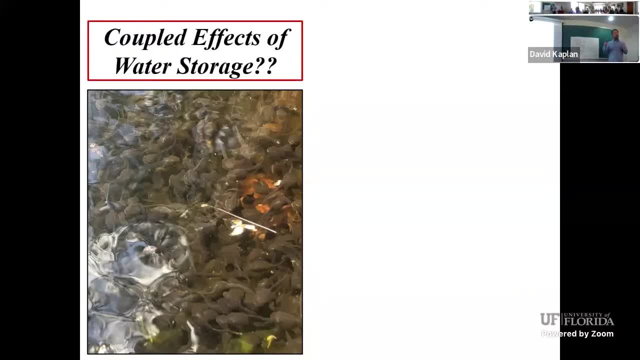 And Chris Dutton, I think, is here right, He does it- and thinking about consumer nutrient or consumer mediated nutrient dynamics, where if you get a place that's attractive to consumers, be it a hippo or a tadpole, well they do things there. 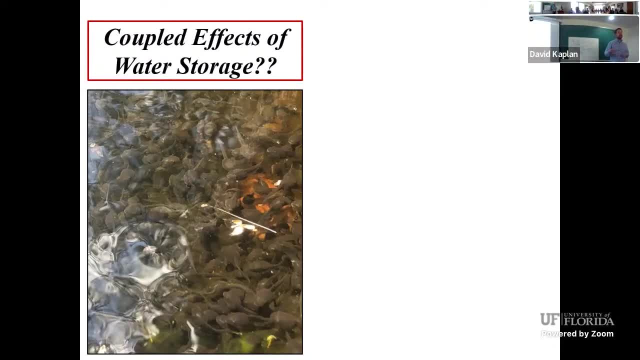 and they can change the topography like hippos, right, But they can poop a lot and they can excrete a lot And that might stimulate and alter the microbial activity. So he got excited about that And he had some field studies. 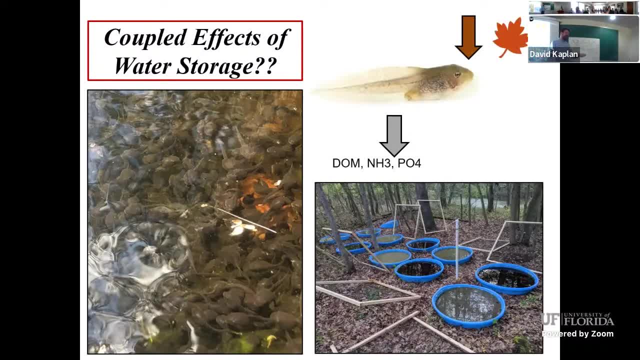 He measured excretions of these tadpoles. I had to go through IACUC training which I had never done before, which wasn't fun. He set up mesocosm down in the field where he would have tadpoles and where he wouldn't. 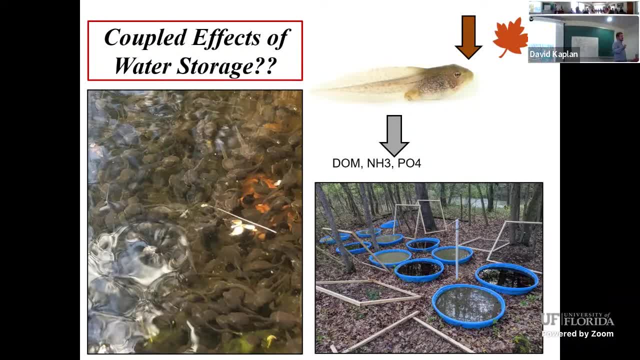 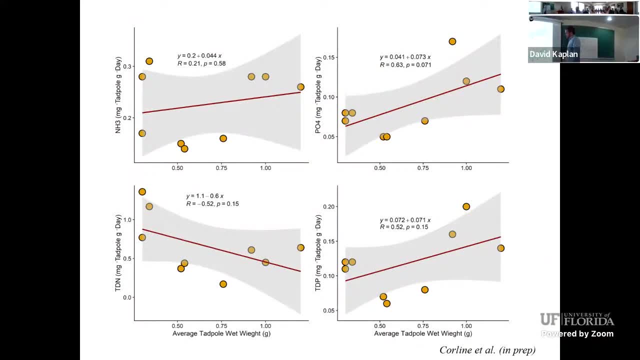 And this again. he just gave me kind of a first draft. I don't think it's close enough to even call it that, but he did give me some figures, And what he measured was excretion rates. Here are tadpoles as they get bigger over time. 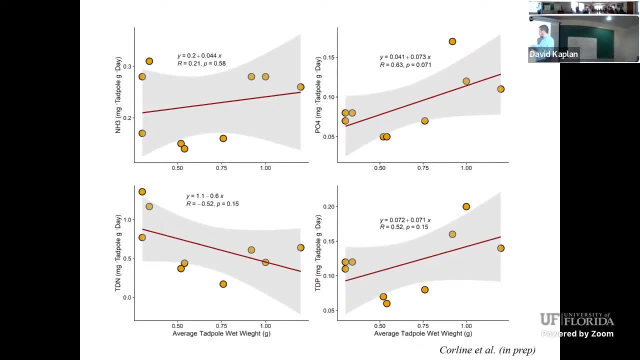 because he measured excretion over time. And here are nutrients, right: Ammonia, phosphate, total phosphorus and total dissolved nitrogen. And I don't know that the trend with tadpole weight is all that important. The point is they're excreting some stuff, right. 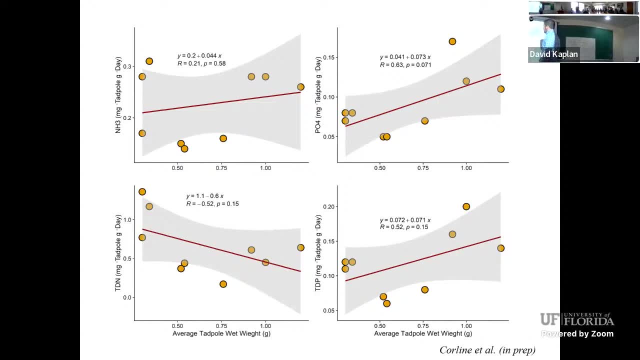 Both in the nitrogen and phosphorus. What I guess might be somewhat interesting is the phosphorus excretion rate per gram of tadpoles increasing. So as you get bigger, clearly you're gonna excrete more tadpole, more tadpole, more phosphorus, right? 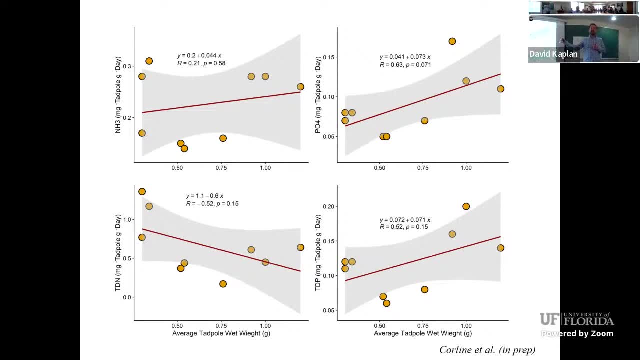 But you're actually doing even more per body weight than you would have when you're small. But the point is they're excreting stuff which is not all that surprising And as irrelevant as the next question, right, Does it have an effect? 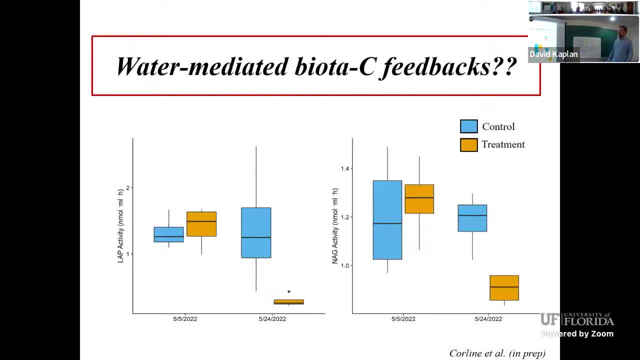 And so one thing he did was he went out and measured extracellular enzymes, microbial enzymes, things they put out to help them do their things. I'm only showing two here, the ones that had an effect: Obviously the controls in blue and whatever orange color that is. 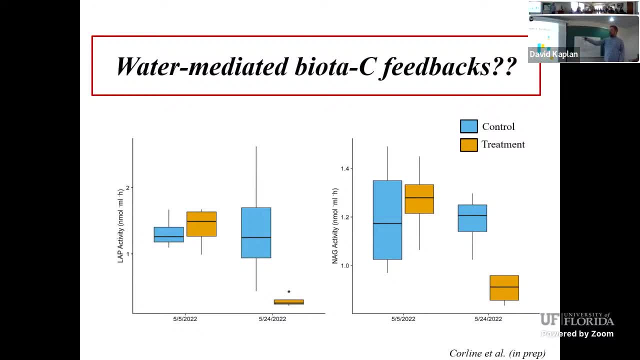 is the treatments where we have the tadpoles, Both of these enzymes which I can't pronounce them or know what they are. The point is they're related to nitrogen acquisition. If these are elevated in the water, that means the microbes are excreting these enzymes. 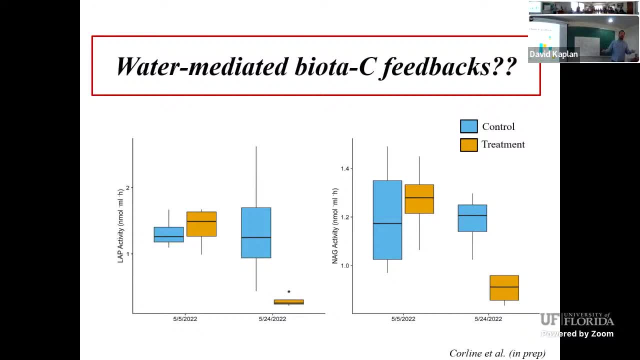 to help them go out and harvest more nitrogen, because they might have a limitation on nitrogen. And in the first part of the study there wasn't much difference. of this dissolved This enzyme in the water. But then, with time right, You can clearly see that the treatment 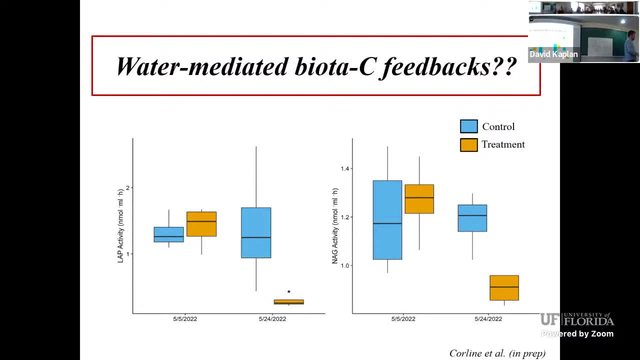 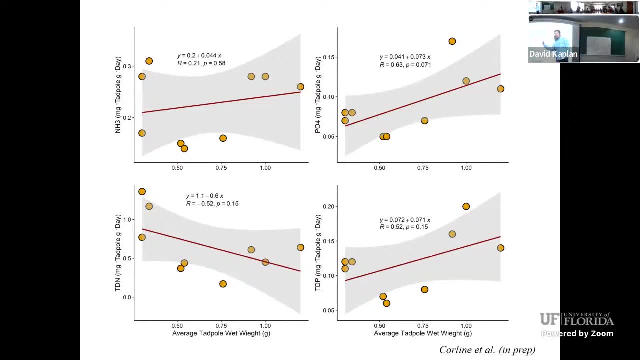 where there's tadpoles was reduced in this nitrogen harvesting enzyme suggesting coupled with this, where they're putting out some nitrogen in addition to phosphorus, we're putting out some nitrogen, Maybe that nitrogen limitation was alleviated and they didn't need to put out that enzyme to harvest more. 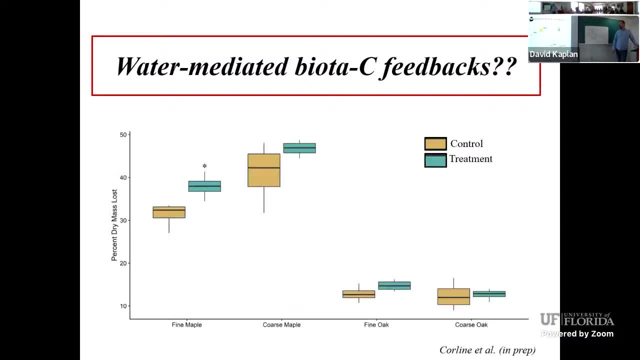 So again, is that relevant? So then the next thing he did- or in concert, I guess, I should say- was he put out mesh bags, litter bags, where you actually pack it full of litter and you have a mesh or fine mesh one. 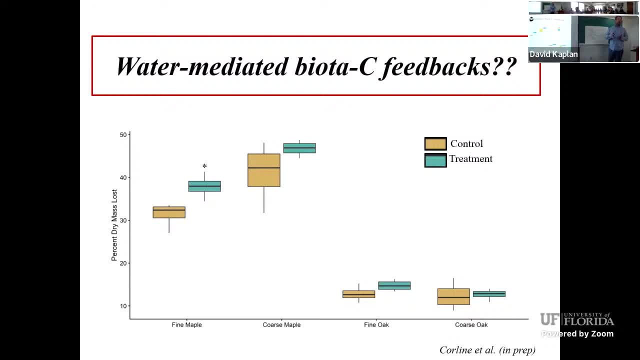 which you don't let things like tadpoles in, So they're not allowed to directly munch on the litter. And then you have coarse. So the one thing that's happened in this microbial degradation, whereas you have coarse, and that allows both things to happen. 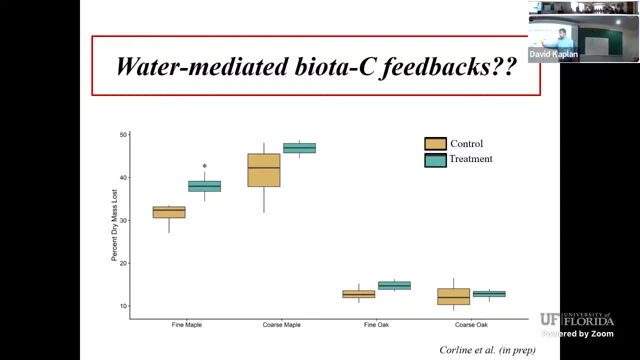 Some of you may know that our guess that maple is going to have more decomposition than oak. But particularly with the maple, and significantly, our power is limited And that's an issue that we're discussing. There are powers limited in terms of sample size. 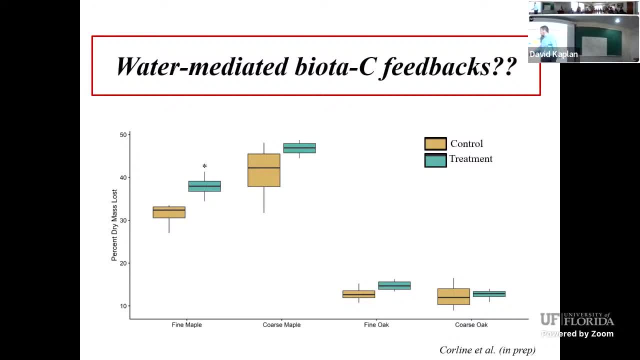 But even with that limited power we have a significant increase of the dry mass loss in the fine mesh of the oak or, excuse me, of the maple, And that pattern kind of holds, your course. But this is what I want to emphasize because, remember, 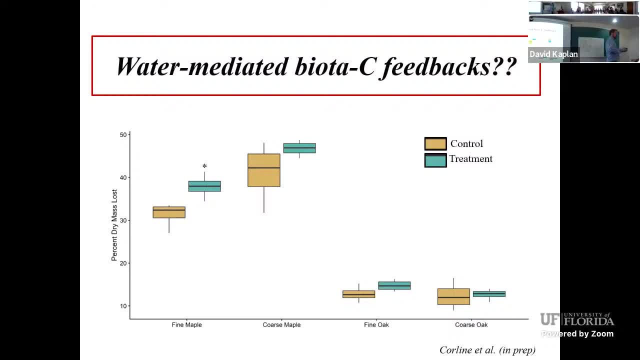 the tadpoles aren't allowed too much on the stub, But their presence and excretion of those nutrients might be stimulating Microbial activity and stimulating decomposition. All right, so I said that's still related to water storage and or biogeochemistry. 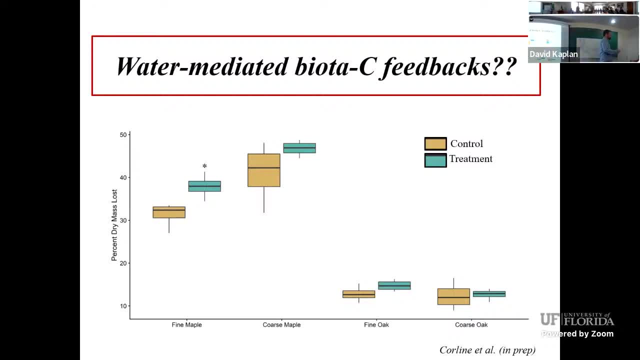 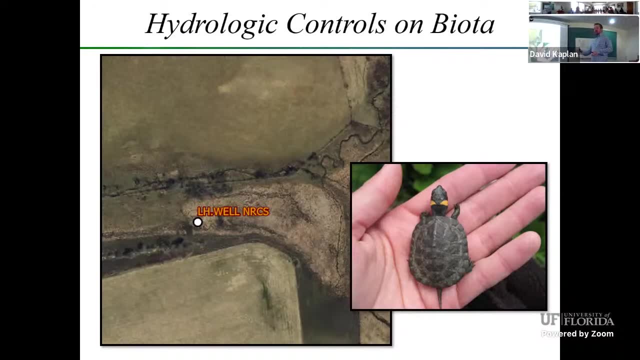 but I'm using it also to segue into biota, which is the last of the grids, And I might be cheating a little bit here, but I want to do something close to home in the mountains where I live now. So there are these bog wetlands that are seepage wetlands. 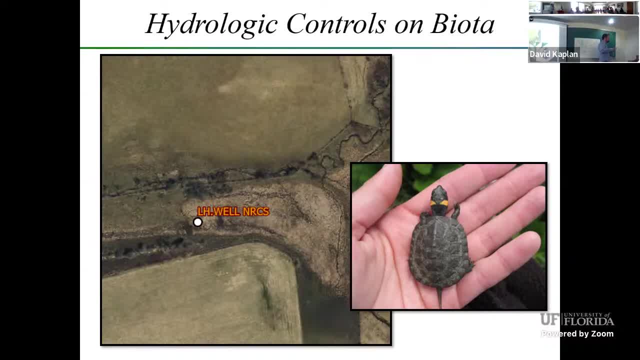 that are either kind of distant. So maybe we can consider these geographical isolated. They might be the initiation of the drainage system or that stream, but sometimes they're next to a stream. Then they're not bogs. I don't know why people call them bogs. 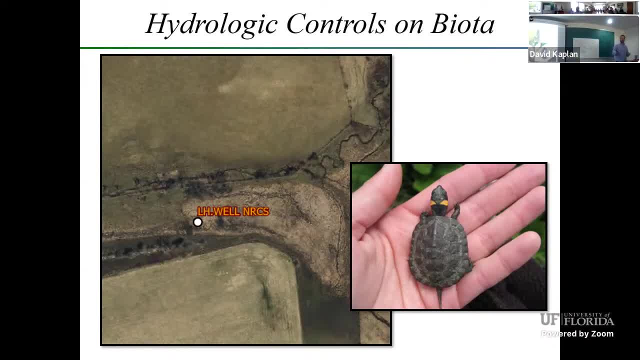 They're mineral rich soils but nonetheless they call them bogs and they're groundwater seeds And they support bog turtles, which, again, probably shouldn't be called bog turtles, but that sounds better than mineral turtles, And I never heard them out of the mud. 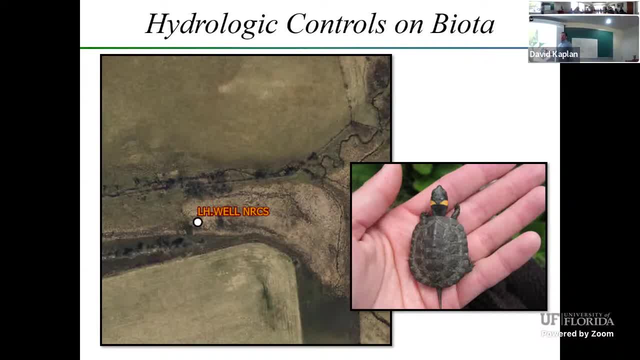 They're better than endangered because of habitat loss. They're pantomimic, They're really good pets. People like them as pets, So people always farm some good pets And I'd already had an existing collaboration with Carola Haas in wildlife on an Eglin Air Force project. 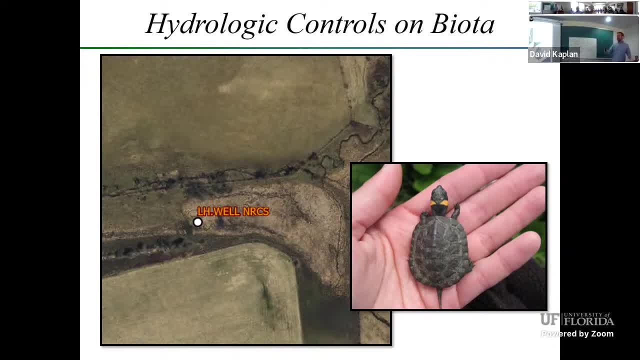 which I'm going to come back to- And she said: well, we've been working on this, working on this, but it turns out hydrology probably matters. And it does because they like constant saturated soils for their hypernicula and other kind of needs. 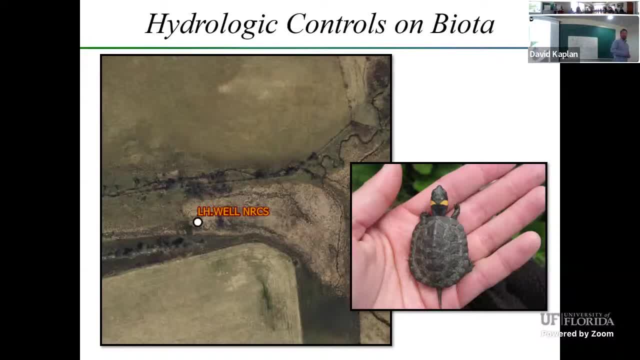 And so I have a master steward working out there where we've instrumented beyond just this. well, We've put in a lot of wells in a lot of different places. Beautiful areas again right off the Blue Ridge Parkway, Not as nice as the Bone Valley District, but it works. 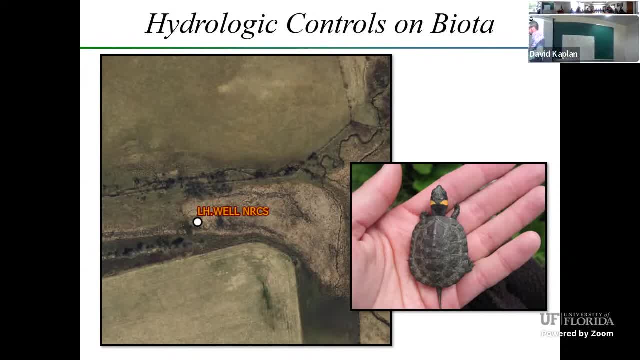 And we put multiple wells And what's crazy is it's not that big. I probably should have put a scale here, because we put five wells out in probably the area of two of these rooms And I was expecting some water table equilibration. 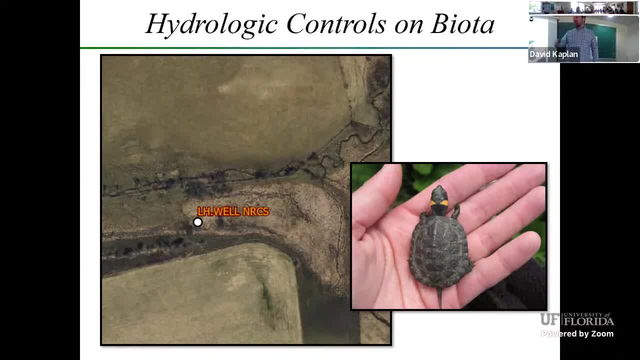 And one place. the water level's always like this, right at ground surface, Three meters over there, five meters All over the place, And it was just crazy that not much equilibration, meaning that the hydrology's quite complex. 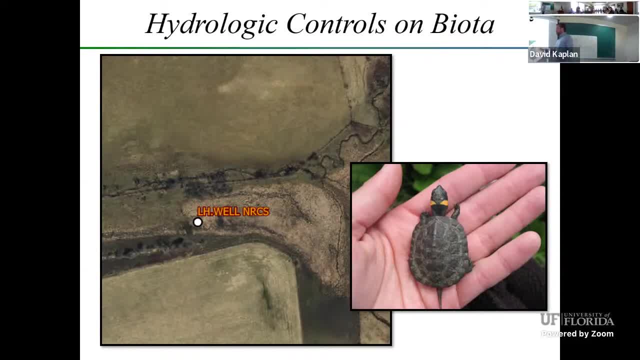 Because I came in there thinking: well, if we want to make spatial maps of hydrology, we just need water table in one place and put some topographic data out there and we can spread the water out. But couldn't in this case. 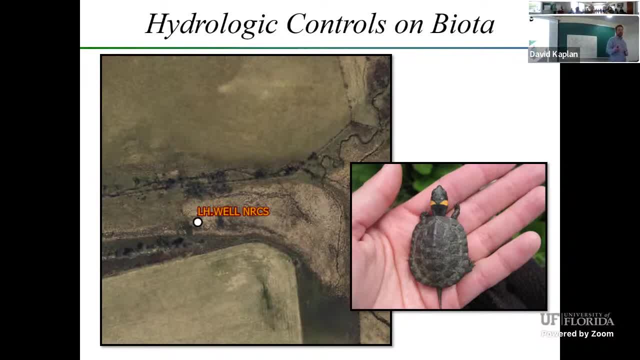 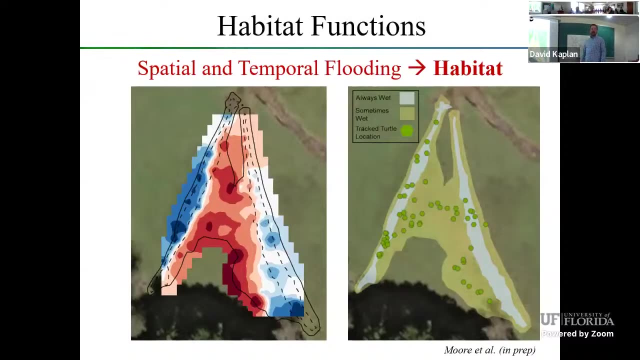 And so what came clear was these seeps, these discrete ground or seeps where the water comes up, is quite important for that habitat area, right. And so, across six to eight sites, that's what we're doing, The multiple wells, But we're also using ways to map those seeps. 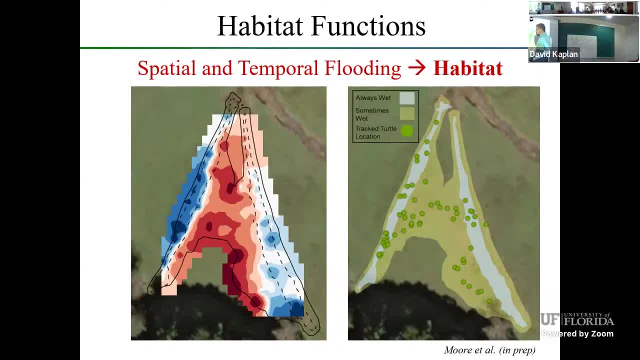 and the seep habitat. So sorry, I'm a legend. This is temperature temperature maps. So this is Ryan Wormuth, a student with a hypersensitive thermometer, always going a certain depth below the soil surface, record temperature and also specific inductance. 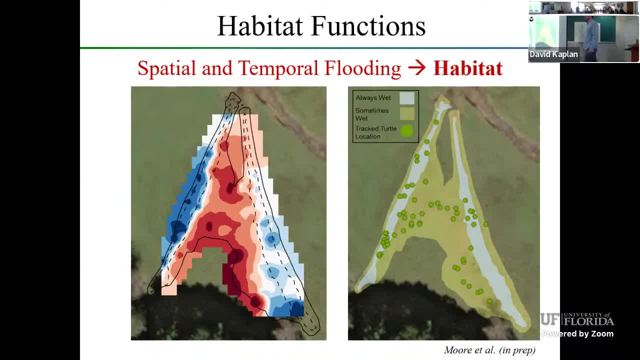 which the map looks the same And the cool spots- because this is in the summer- are where groundwaves are popping up right And some probably not saturated habitat in the middle, And you can see these two seeps here that he just walked. 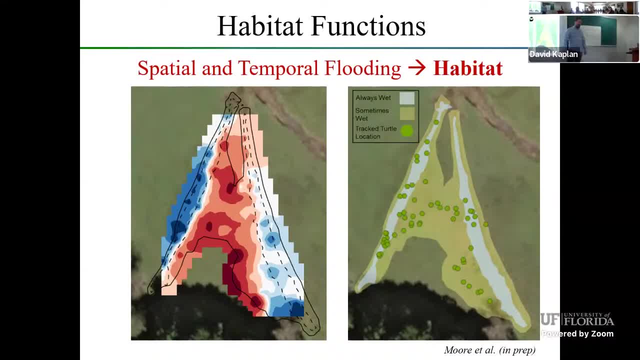 So always wet, always wet where it's based on vegetation. just him always out there, Because these seeps keep it constantly, constantly wet, And even during the driest time is when he walked and made this map. Different time he used this to make a distribution. 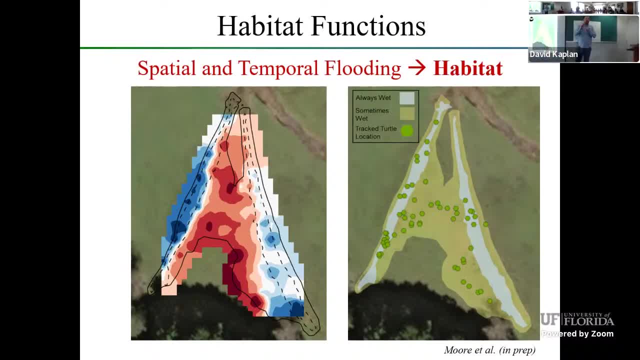 of that habitat area And he also put telemetry things on glutamon, those small 12 turtles, and mapped where they go, And so we're working now to try to align it, And we're working now to try to align those things to kind of. 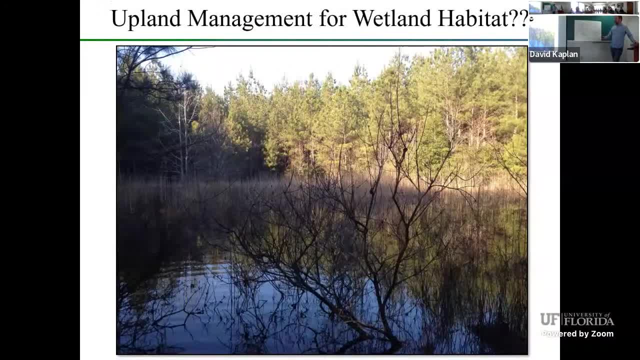 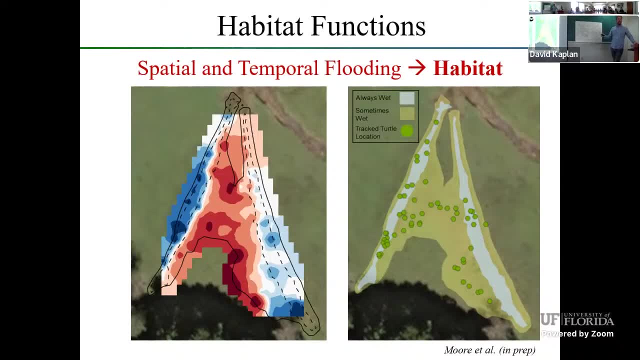 inform conservation. So the drivers of this we're trying to figure out as well, like landscape position, depth of bed rocks, so that we can kind of zoom out and think about those landscape scales, so we can maybe identify what would be good bog habitat where people aren't looking. 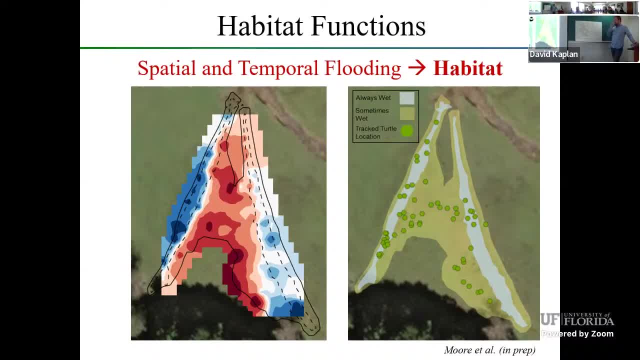 bog turtle habitat, I should say. And so that's the point of that And the driver of that is this topographic groundwaves setting right And you can look at the hill slope, which you don't have here, but you can look at the hill slopes there. 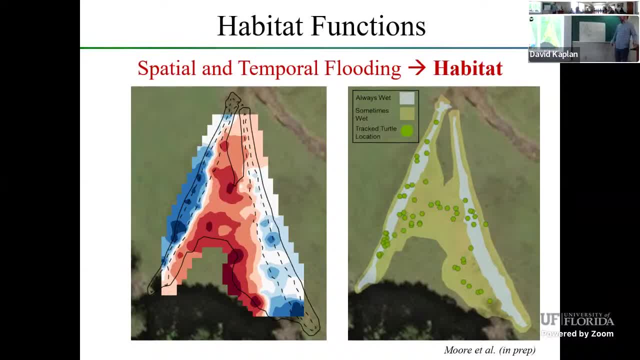 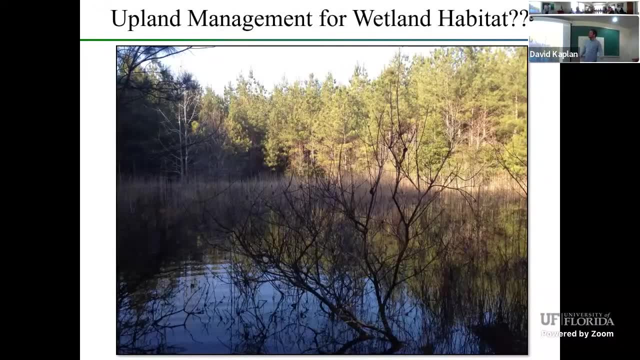 and probably guess where that water is going to pop out. But there's other drivers of water storage and what it might mean for biota And so I'll pull this in that. David has worked on quite a bit in wetlands, And David and Matt and I have worked on in uplands. 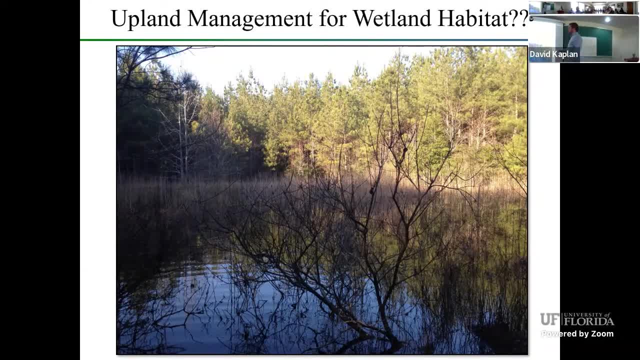 to think about upland management. So here's our wetlands. This is a thermal pool in southwest Virginia which I was lucky enough to stop by and get a bunch of country ham. Afterwards here is a very dense pine forest. this relic. 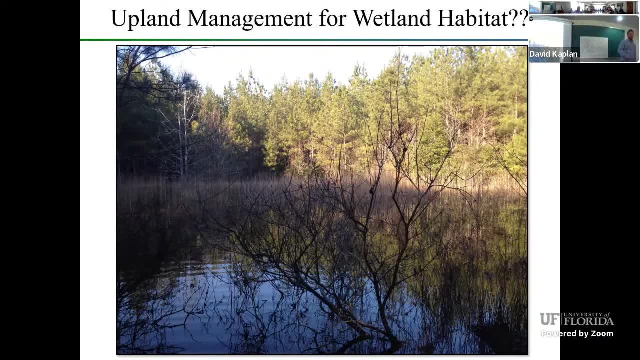 from industry Owned by, I believe, TNC, that needs some thinning, A lot of straws in the upland which connects to this wetland subsurface. We've already kind of talked about that. So is there something you can do outside of the wetland? 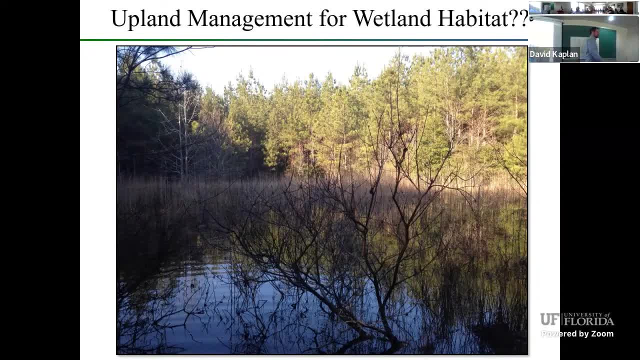 managing this upland to do something for this wetland, In this case, water levels. and how much water? right, Because when you take the straws out of the upland, where there's probably less amount of transpiration, they need more water to hydrate this wetland. 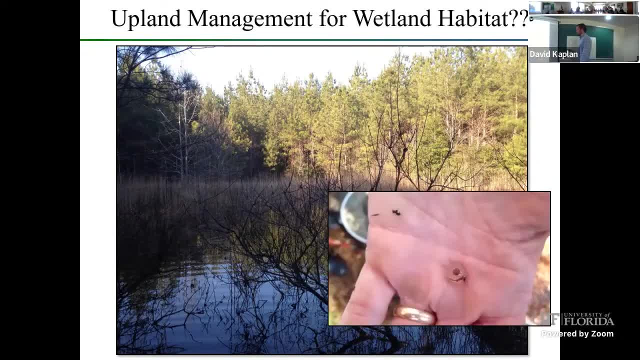 And in this particular wetland in southwest Virginia, when we walk around There's a lot of these eggs, which is a maybe salamander egg which is listed, I think, at the state level, not federally, But they also need the timing of that water storage. 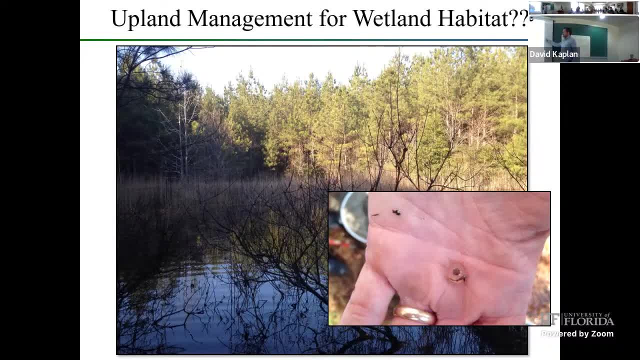 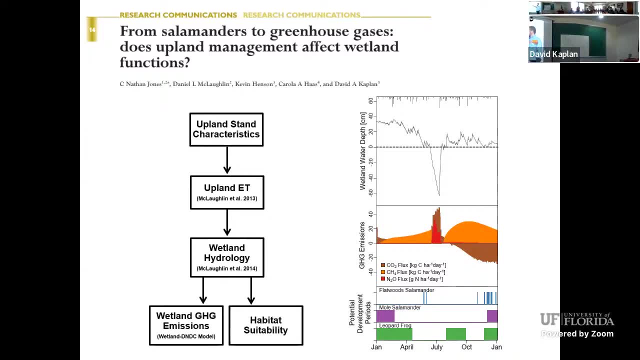 to do their thing that might be affected from upland activities. So David and I, with some others, we linked together some models we worked on with Matt and say, hey, it's all about the upland honey trees. You have probably something that says something. 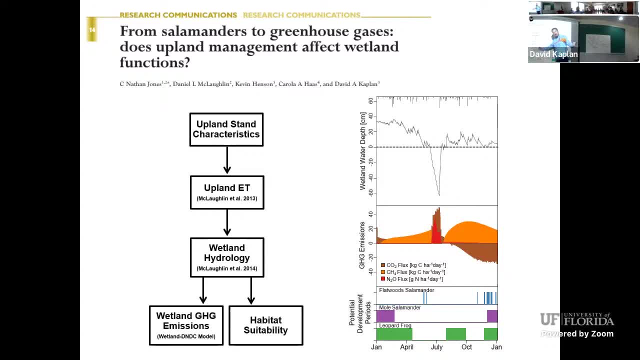 about the water use or the evapotranspiration of upland. Well then, our model to connect upland groundwater and wetland water. And then we said, well, we can get that using a greenhouse gas emissions going back to there, but also habitat suitability. 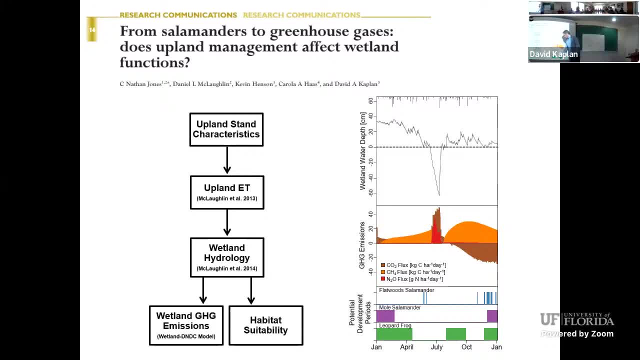 And there's something about when a mole salamander or a leopard frog or flatwood salamanders, how many periods of wet, periods of time do they need to have their potential development? It was a thought experiment. It's probably not right. 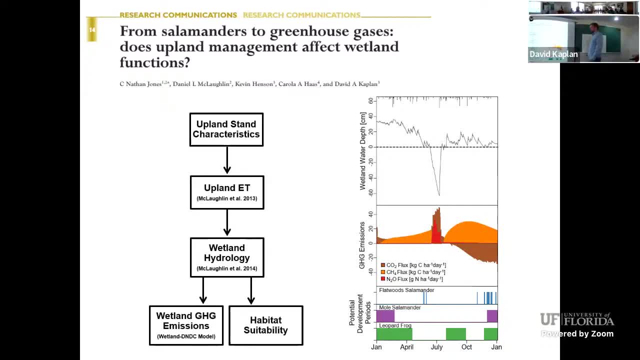 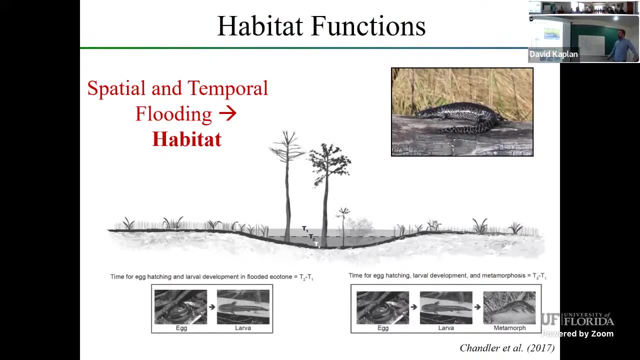 Maybe not even the direction of, it's probably right, But the idea is there that we defend. is there is some connection across these things? And then I know David and his students have taken it forward in terms of different treatments And to that same point. and now here. 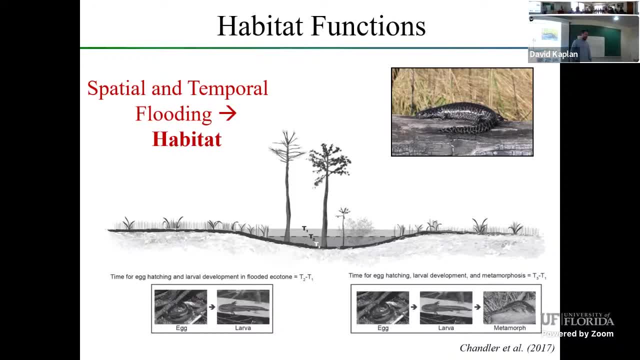 appears that flatwood salamander, which is another federally listed species that is, occurs in large part at Eglin Air Force Base, not too far from here, Panhandle, And working again with Carol Haas, I mentioned her name, her student, Houston Chandler. 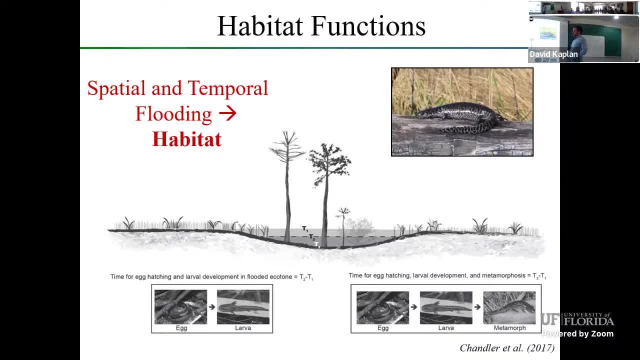 In fact, this is soon after I got to Virginia Tech And we're still doing some research on what's happening in these areas. So last day, looking at what water level data they have distributed across the wetlands, Thinking about the timing of the ups and downs of water level, 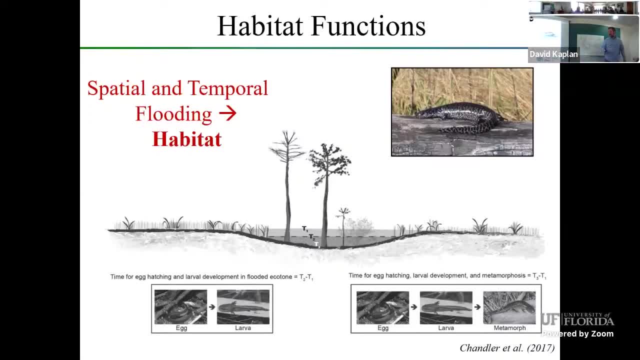 and what habitat it inundates and what that means. because this, these time periods to go from beg to larva or larva metamorphosis that these guys are thinking, no wonder they're endangered. They need really specific cues and timings and habitat. 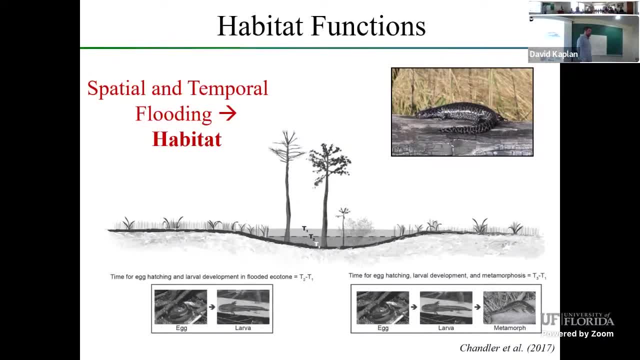 They need it to be inundated habitat, not canopy. so this is informing- or they're interested in now- things to do within the wetland, because these things have been fire excluded for quite some time, but those are naturally more herbaceous, embedded depressional wetlands in that flat flatwoods landscape. we've continued on this. 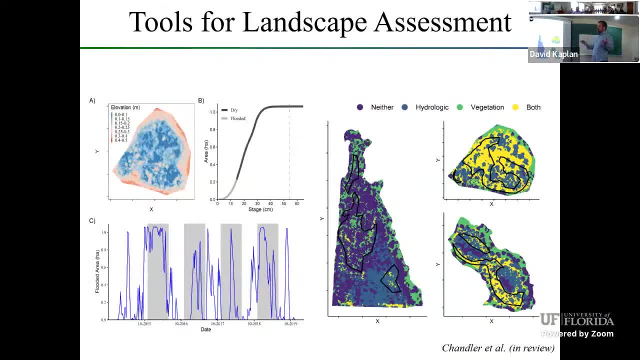 project, but at a bigger scale, where now we're using topographic data across the place- right, and with that topographic data we can zoom in on wetland, wetland here- and look at highs and low areas- right, the high areas are orange and the low areas of the blue, right- and then we can build. 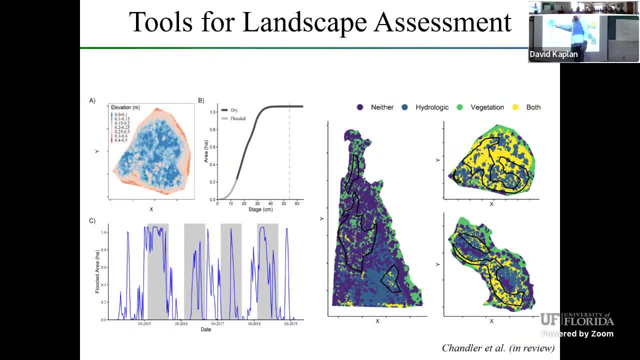 staged area curves with that information right. so if i were 30 centimeters, we know how much of the first, how many hectares are flooded, and then we go up 50 centimeters and we can do that. and then, if we indeed have a water level device recording water level areas, 15 minutes in that said wetland. 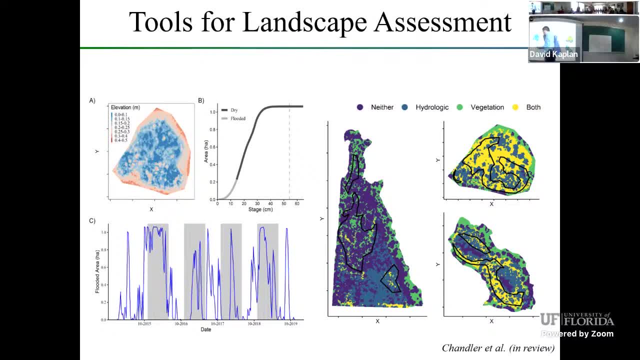 well, now we can map flooded area over time and put gray bars when those are key times for development of that species. but to extend that beyond where we can instrument with wells, we still have all this topographic data right and so we can still kind of do this even when we don't. 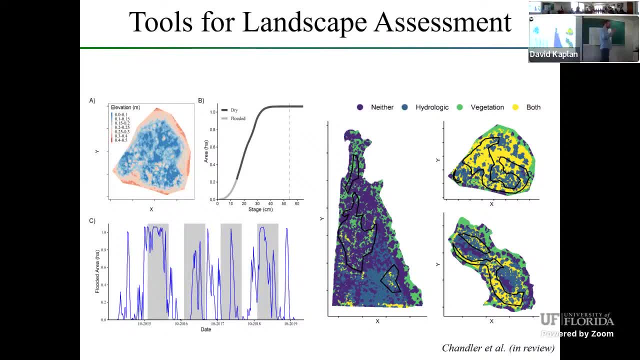 have wells, think about places which might be suitable or not from a hydrologic perspective in terms of their flooded area, as well as use it to get us something about vegetation. right light, the first returns. i can remember when mark brown said this in i don't know 2014. they just kept on. 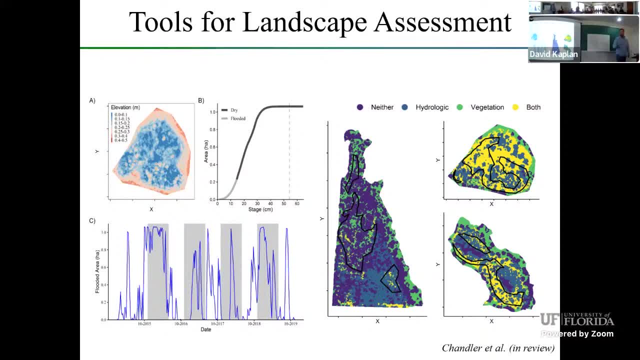 throwing all that information away and it's useful and it is and it can give you something about canopy structure and again, they like these species, like low stature herbaceous, and so trying to find areas where we have estimated good hydrologic suitability, but also so suitable vegetation across this landscape to identify what might be um potential wetlands for. 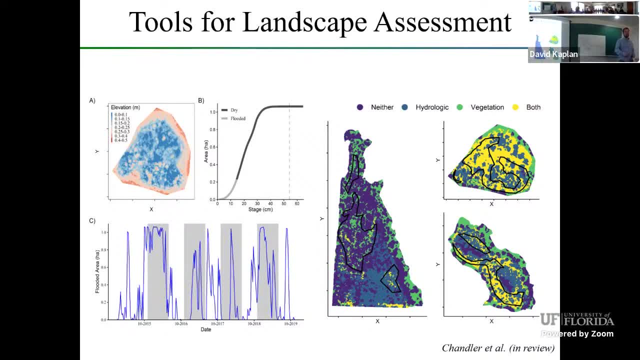 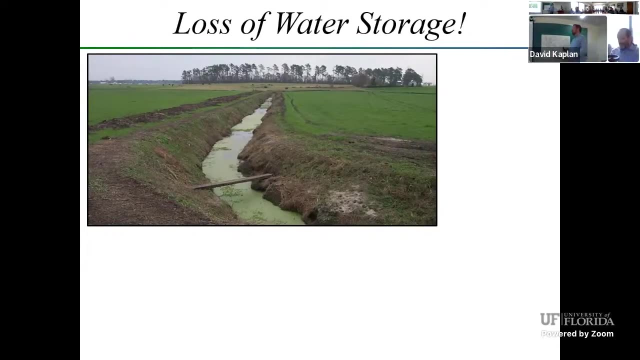 um relocation, the introduction of species, because that's what they um, they introduced and that's um and that's in review right now. so i'll end with. what time is it? we got seven minutes, nice, i'll end with. well, i hope. i mean, i would imagine most of us before we walked in think of various different ways that holding. 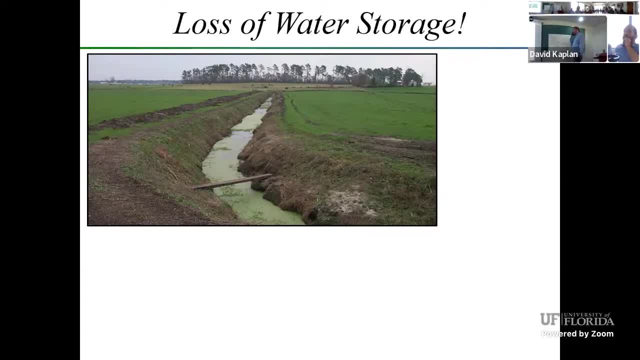 water back in a wetland probably matters, right, but what i was trying to give you today is some things i'm doing with this and what I'm doing with the wetty water relevant resolution. i'm gonna give you we're doing in that context and also the tools that you can use to determine the extent to the. 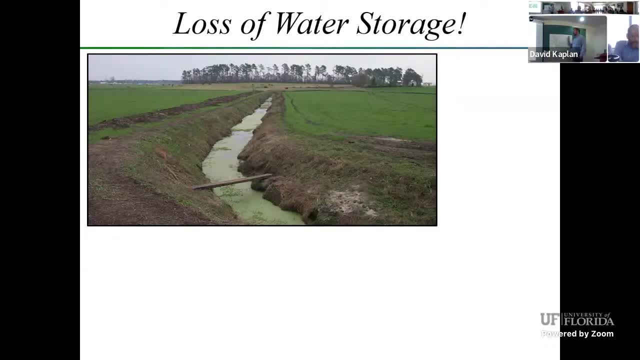 effect of that on certain functions and quantify that And also to inform largely conservation, restoration and all that kind of stuff where we have a loss of this water storage. This is in Delmarva, a ditch draining a wetland. You can see what used to be a Delmarva Bay and the ditches. 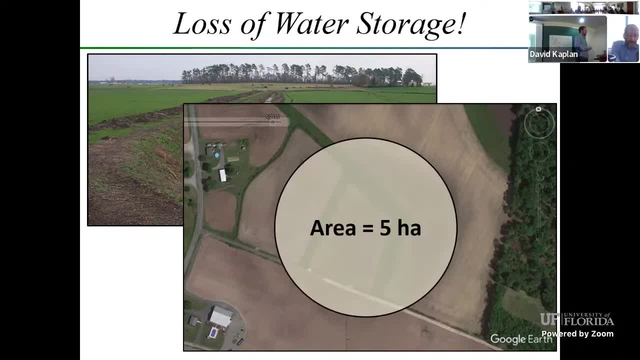 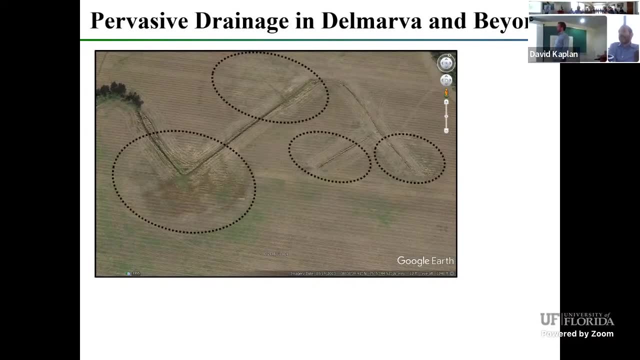 removing it. That was a five-acre wetland, probably five hectares, excuse me, And it's not just in Delmarva, it's here, it's everywhere. You can clearly see these ditches here, in what used to be Delmarva Bay's probably, And with that you're actually increasing connectivity, right, And you're. 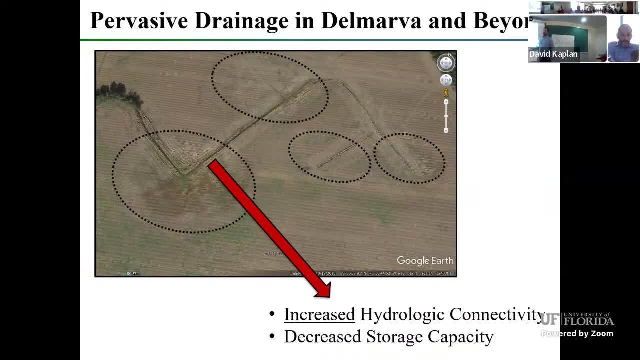 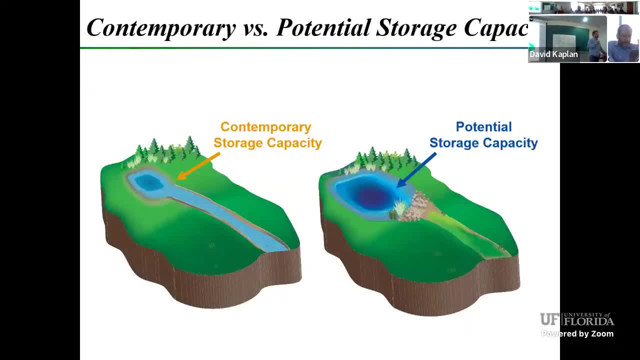 decreasing storage capacity, the ability of this landscape- or, in this case, even be a wetland- but to hold water back for these functions presumably related to storage capacity. This is a cartoon that Chuck wrote. I don't know if you like it or not. Either way, he says: hey, this is how much water you. 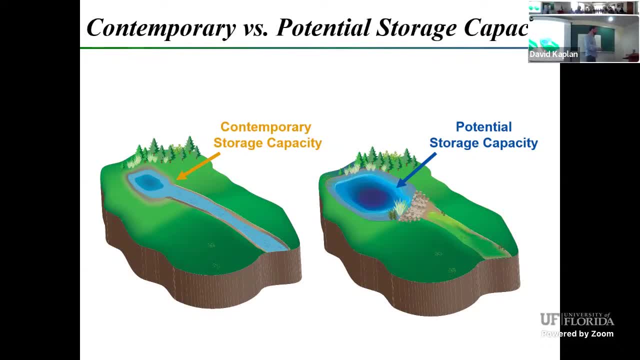 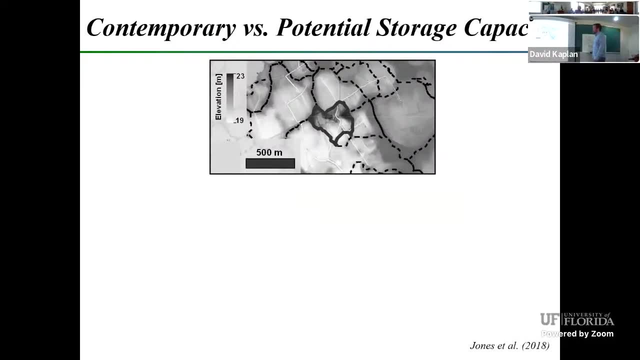 can hold back if you have a ditch, and this is how much you have if you don't, And we'll call that potential storage capacity. So then, this is work that Nate Jones did while he was with me. Again, he's been very good at LIDAR data. You can see the ditches here. Here's one particular. 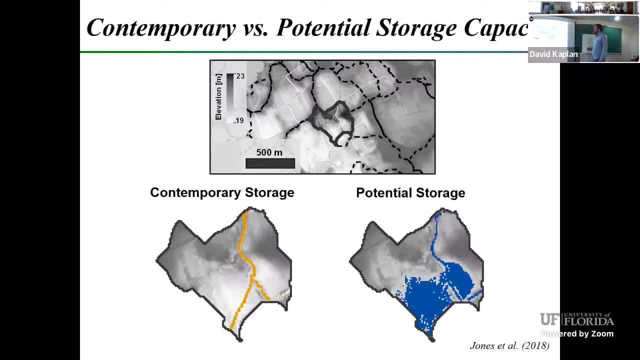 little wetland, catchment or watershed if you will, And then you can zoom in and he, with that individual wetland, he said: this is how much water you can hold before these ditches connect out and it spills out. But if we didn't have those ditches and we plugged them, 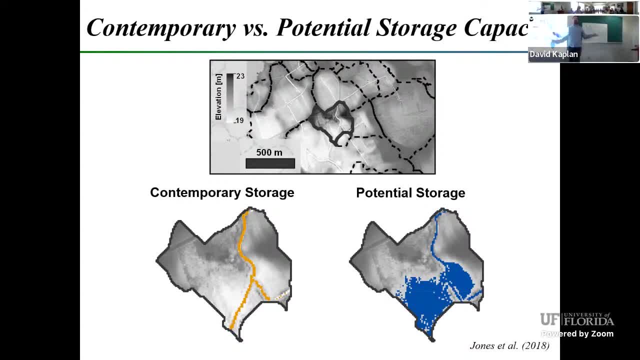 this is how much the system would hold before it spilled out of its rim, like it naturally would. And so, using that, across the Delmarva Peninsula, hundreds of thousands of wetlands, identifying where there were ditches and where there weren't, and if you had restored them. 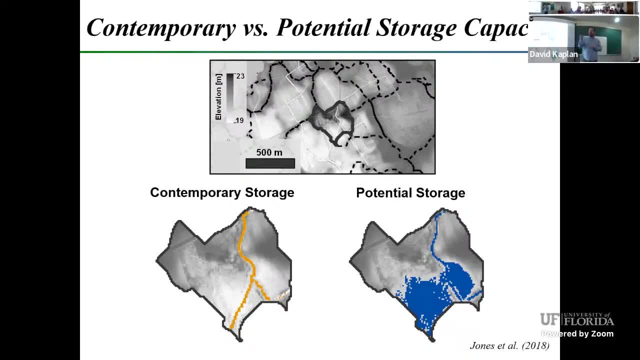 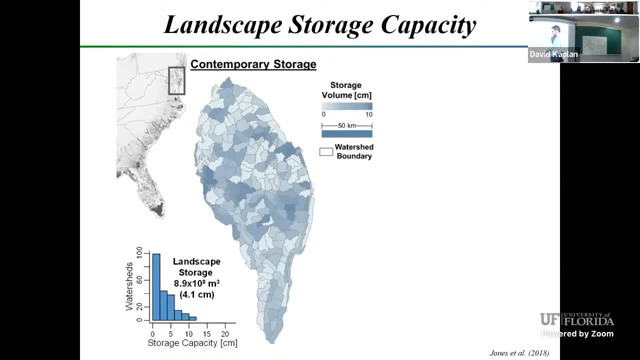 what would be the storage capacity gained? Or you can flip it and think about what it used to be and what was lost. He did that across Delmarva aggregated to the 10 level up, I believe. here We can see landscape storage and a distribution of that Hard to see with this. 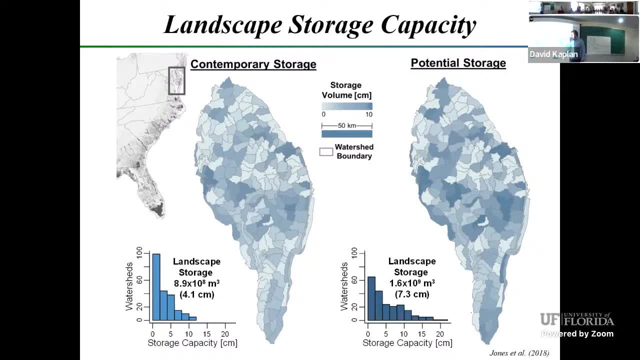 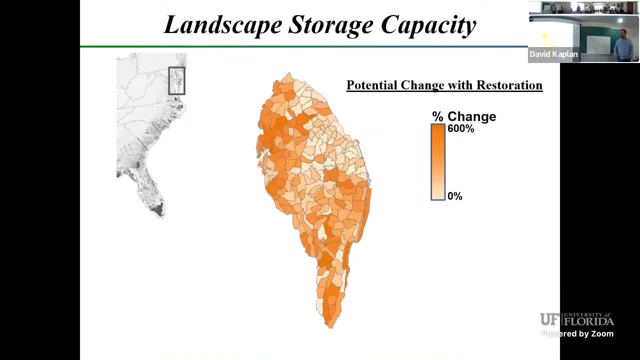 color. I never really liked it. but the unit or the numbers show you if you spread it out over the landscape or a magnitude higher. To make it clear, we can just look at percent change where there was a lot of wetlands ditched and what we would get back. Clearly we're not going to 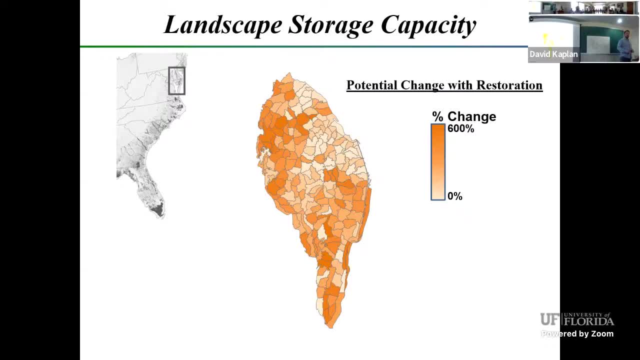 restore all of Delmarva Peninsula, but maybe a tool to identify where it makes the most sense and where it doesn't, And to build on that. I'm going to go ahead and show you a little bit of the data that we've got here. I'm going to go ahead and show you a little bit of the data that we've. 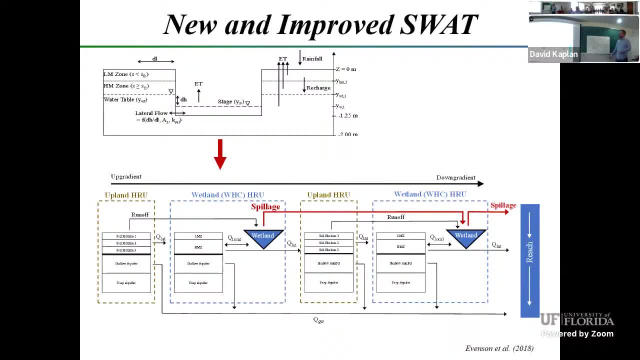 got here And to build on that, I'm going to go ahead and show you a little bit of the data that we've got here And to build on that. then we take this model back that we started with. Here is the SWAT model I alluded to that. Gray was working on the Prairie Pothole. 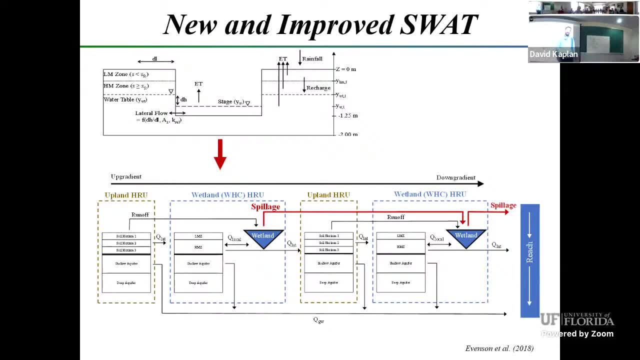 that represented individual wetlands better but did not represent sub-surface exchange. So we took this kind of version of this model and embedded it in the wetland landscape element or exchange along the spillage down to our reach, And we did this for the 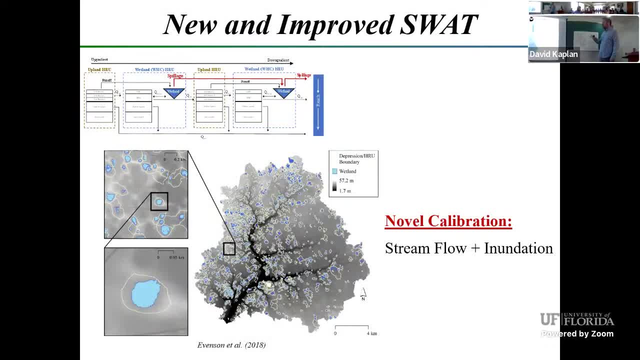 Greensboro watershed, which I'm highlighted here, And what was quite cool about this, as I thought, was that we calibrated the model not just with stream flow, but we also calibrated it with time series of inundation from Romanlinks- data Landsat to say we want to get it where. 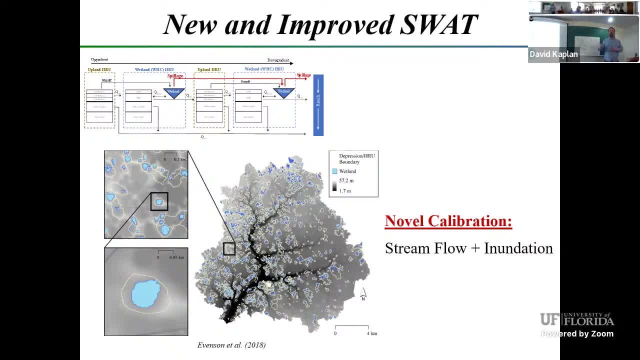 it's right on both ends, meaning that we could get the right answer for stream flow but not represent flooded area very well in reverse, and we wanted both to happen. So I thought that was a pretty cool thing thing, and then we got to play with it, and this is still in prep, and it's been in prep for, i think. 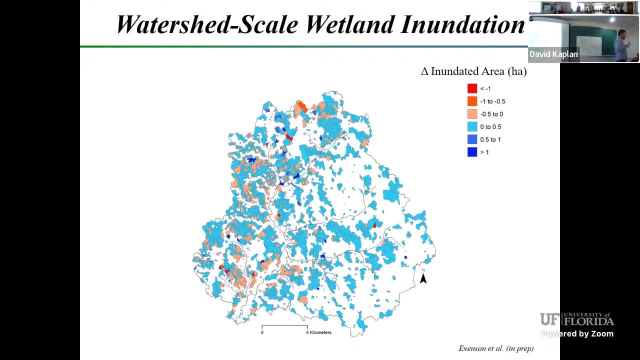 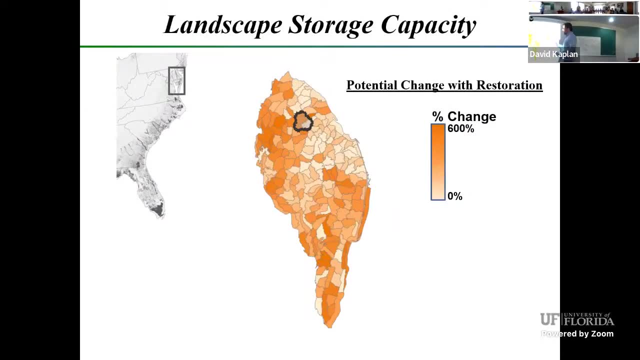 five years now, um, and i don't know that it's going to go anywhere, but it was a nice place to end this talk, i think, with colorful pictures, to show you a tool like: hey, we know this information right, we have a calibrated model. we can now say what if we did this restoration at grainsboro? what would be? 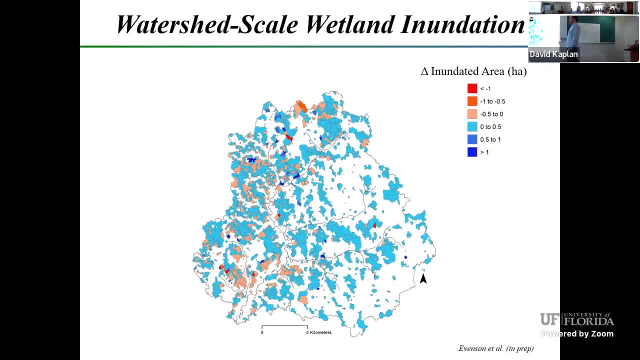 the change in certain things that we've already talked about, that one of which would be you get a lot more flooding. um some, you actually get less right, because maybe you plug the ditch that was upstream in that particular wetland that was receiving water, but on the whole, you get a. 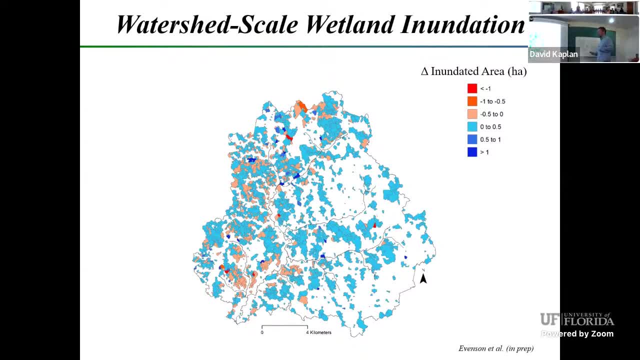 wetter landscape, which is not a surprise, but nonetheless the tool that someone could use to more target and optimize efforts where it might make most sense for other reasons. so you get a big change, and the same thing goes with residence time. i will end there with this. 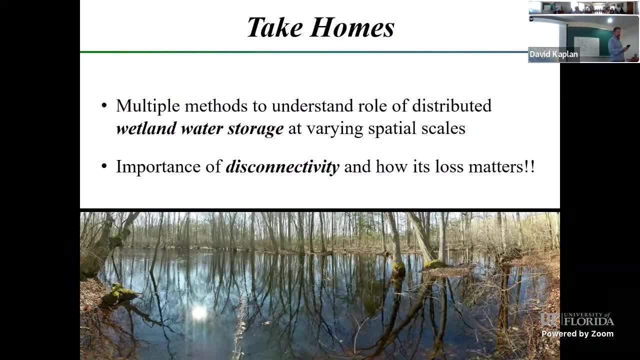 these take-homes and take questions if i have time, all right, all right, awesome, i'll check the youtube and the zoom, but we'll start with questions from the room. i've got an observation. 50 years ago, we worked with HT Oden on the wetland landscape difference. 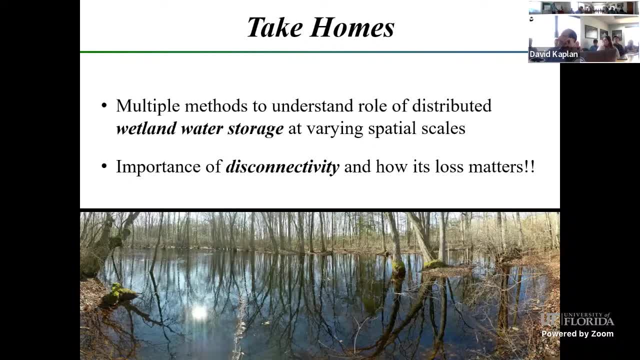 and Oden kept saying wetlands, save water. so i started a lot of times, you know. so in the back of transportation doesn't do it well, it's cute, but it doesn't do it all. right, i guess that's a good thing. yeah, go ahead, mikey, i will go to pietra. i was just with the graph that you had with the. 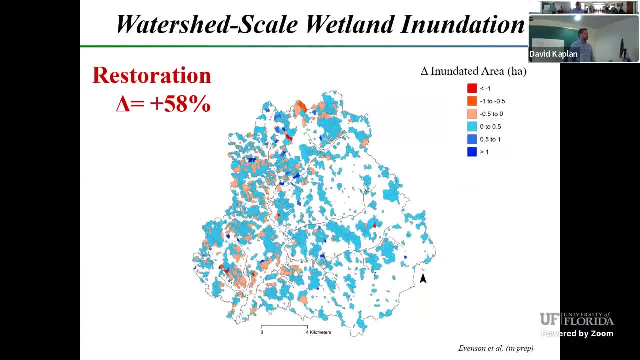 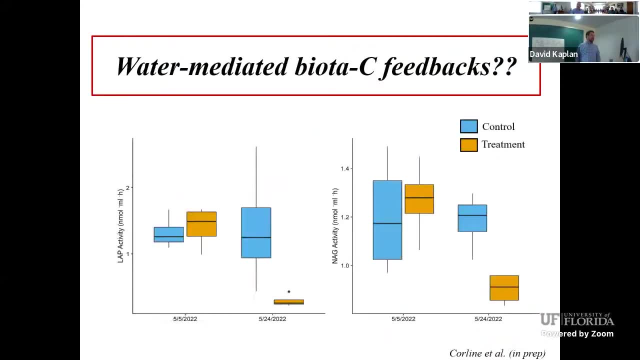 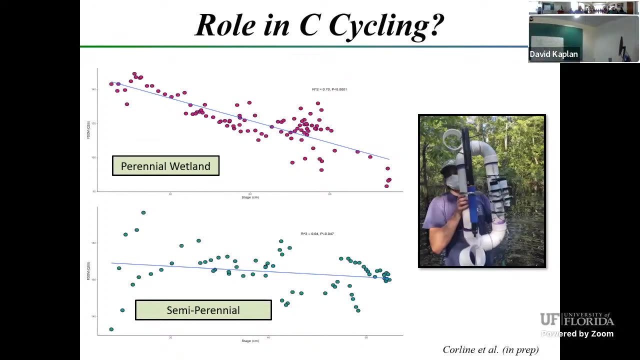 cranial and semi-cranial. i was just hoping if you could just like explain that, because i i heard you talking and then it started like yeah, it was a lot of people, probably fast. um, so this is dissolved organic matter, so how black water is like you've been on, so you're from the area- like, have you paddled black water rivers? 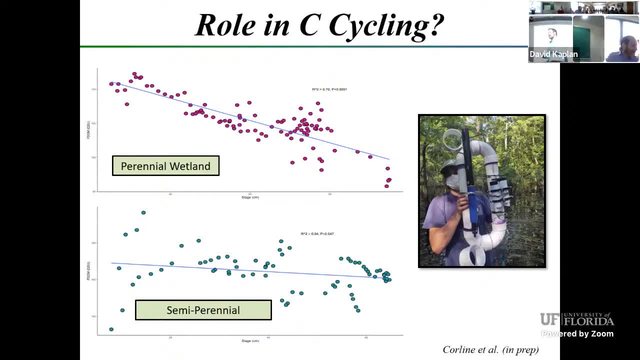 before, like on the santa fe, like tea colored water that's not sediment, that's dissolved color from panic acid and vulva gas and all these organic molecules, right um, and they're generated largely in wet systems and the export of that to those streams, and so this was just looking at some, some measure of 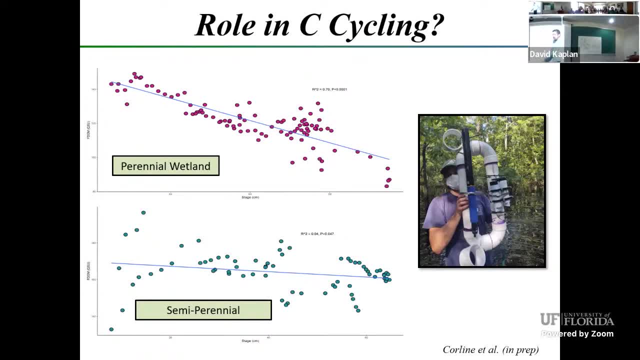 that indicator, um, a lot of caveats, and then water level, meaning that one weapon, the concentration goes down as it gets wetter, but another weapon doesn't, and we can explain that based off the shape of as well. so yeah, we'll go to pietra and then we can start to bring it back to frogs. but i was curious like: 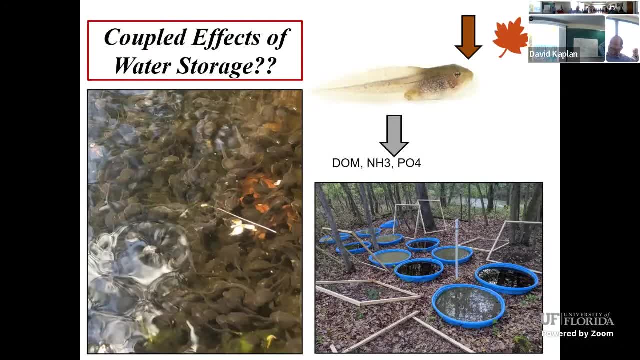 do you think it'd be possible for some of the people who grew up to be the frogs they've taken in all these nutrients and then maybe they leave and go to another weapon. do you think that could contribute to any loss? sure, i mean, that's getting to the concept of like a meta ecosystem, right, and 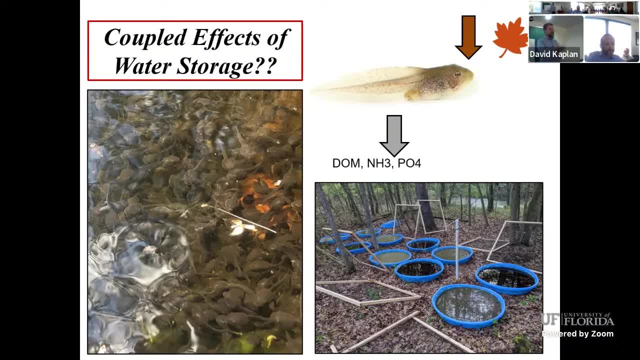 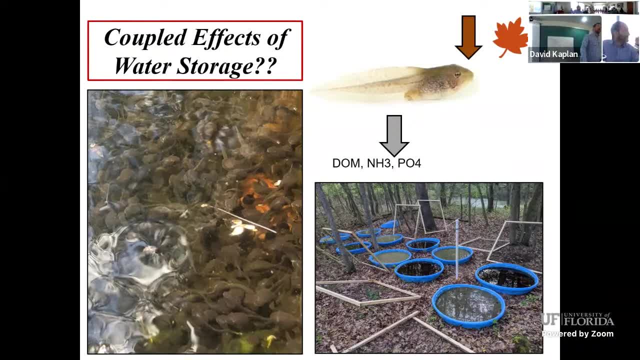 publish this as it is. i'm trying to get him to take a couple of steps, but we'll see couple of steps. but we'll see couple of steps, but we'll see. honestly, i wonder how this affects their. honestly, i wonder how this affects their. honestly, i wonder how this affects their disease rates. 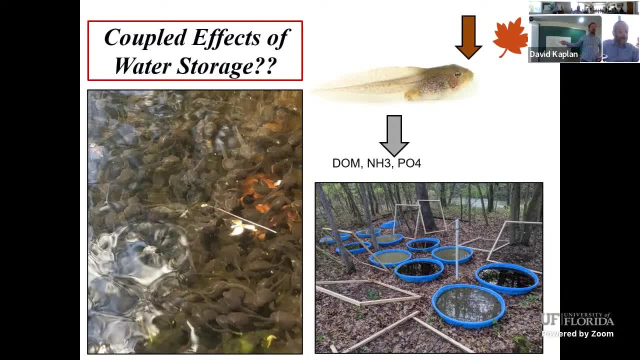 disease rates. disease rates, that's kind of it. that's kind of been. that's kind of it. that's kind of been, that's kind of it. that's kind of been. kiddie pools from walmart, like when they're this dense, yeah, yeah, like when they're this dense, yeah, yeah. 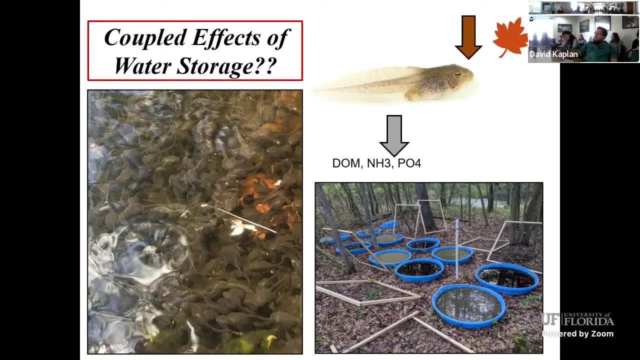 like when they're this dense, yeah, yeah, and the minerals, the, the and the minerals, the, the and the minerals, the, the types of um. what lenses are in the ones types of um? what lenses are in the ones types of um? what lenses are in the ones they choose, whether the minerals that? 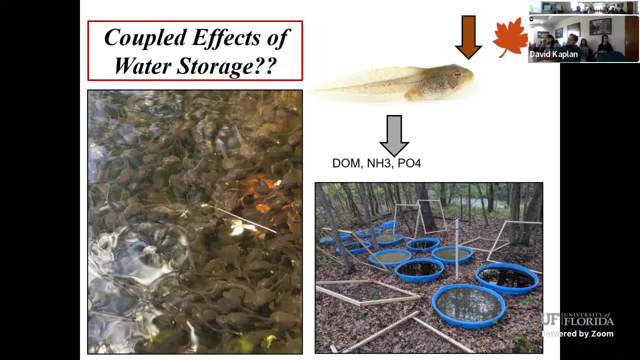 they choose, whether the minerals that they choose, whether the minerals that are found in their specific ones and are found in their specific ones, and are found in their specific ones, and the economy is a little bit effective. the economy is a little bit effective. the economy is a little bit effective. yeah, i don't know, that's out of the yeah, i don't know that's out of the- yeah, i don't know that's out of the scope question, but i was thinking about scope question. but i was thinking about scope question. but i was thinking about it yesterday. i was walking around it yesterday i was walking around. 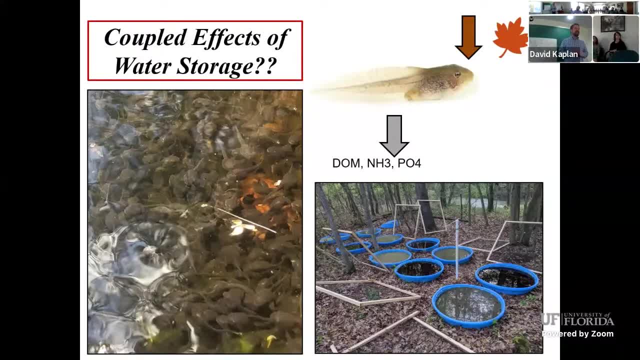 it. yesterday i was walking around sweetwater branch treatment level and sweetwater branch treatment level and sweetwater branch treatment level and think about those things, if that was a think about those things, if that was a think about those things, if that was a trap or not. 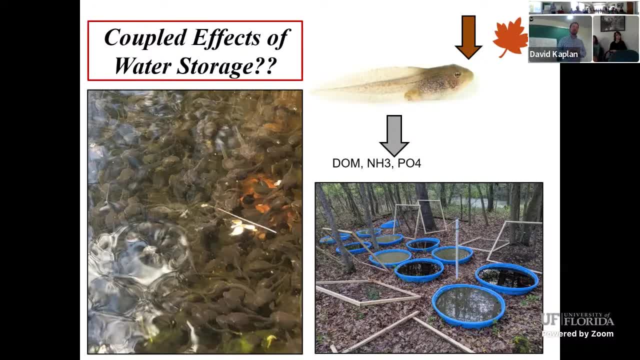 here and then the doctor comes here, and then the doctor comes here and then the doctor comes. thank you for the presentation um. when? thank you for the presentation um. when? thank you for the presentation um. when you said you measured extra similar. you said you measured extra similar. 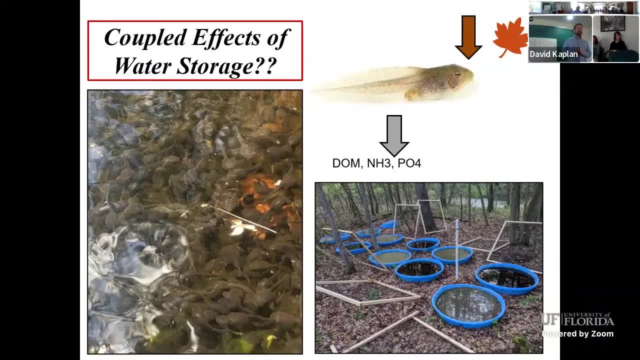 you said you measured extra similar enzyme activity. what was the method? just be on the scope with you. i can. i can uh link you up in my phd, i can. i can uh link you up in my phd, i can. i can uh link you up in my phd student who's done it and gone through. 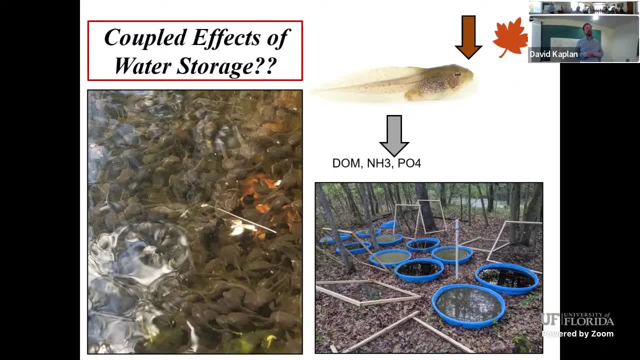 student who's done it and gone through student who's done it and gone through some trials and tribulations to make it, some trials and tribulations to make it some trials and tribulations to make it right it's not right. it's not right, it's not. it's not necessarily easy. oh, because a 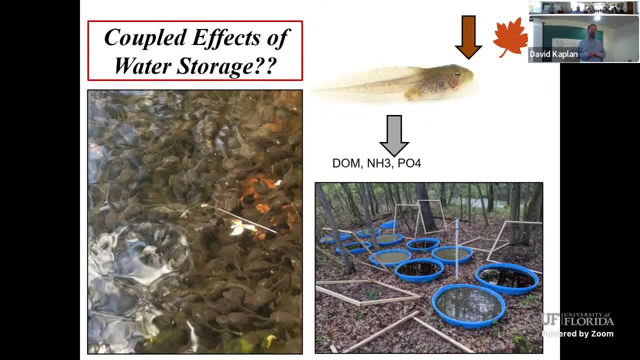 it's not necessarily easy. oh because a it's not necessarily easy? oh, because a part of it would have some part of it, would have some part of it, would have some information to what i would be doing, information to what i would be doing, information to what i would be doing with non-linear kinetics. sure, i'm happy. 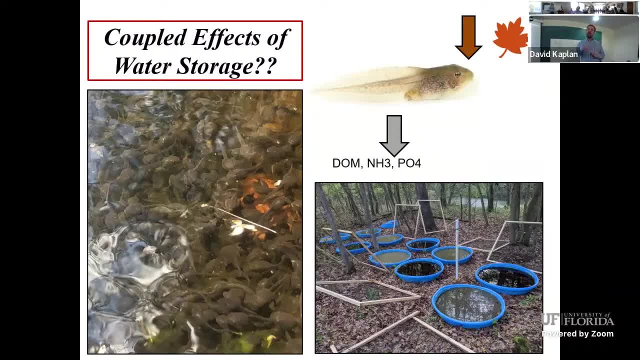 with non-linear kinetics. sure i'm happy with non-linear kinetics, sure i'm happy to. and he's done research and again to, and he's done research and again to, and he's done research and again stepped through some hurdles. so so, yeah, i can like, so you can just. so, yeah, i can like, so you can just. so, yeah, i can like, so you can just contact me here, but i don't, i don't have contact me here, but i don't, i don't have contact me here, but i don't, i don't have any ideas. 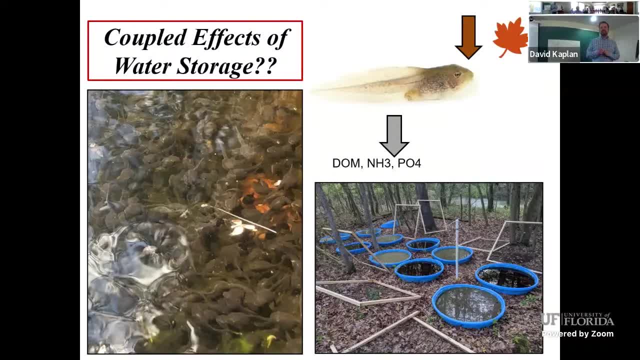 any ideas, any ideas? thank you, thank you. thank you, it's the same perennial, uh, it's the same perennial, uh, it's the same perennial, uh, that mikey was asking about. so that mikey was asking about. so that mikey was asking about. so, one of the things that has been shown. 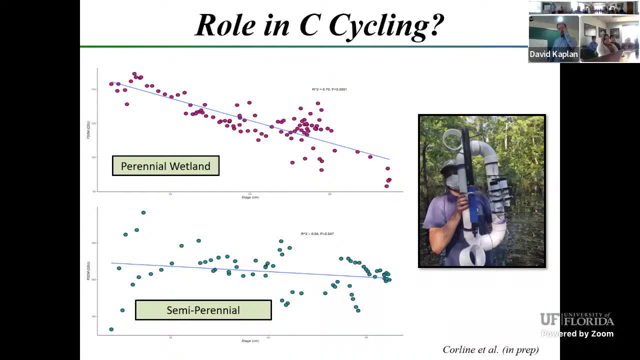 one of the things that has been shown, one of the things that has been shown like, maybe, like, maybe, like, maybe, consistently in sort of catchment, consistently in sort of catchment, consistently in sort of catchment studies, is that the concentration of studies, is that the concentration of 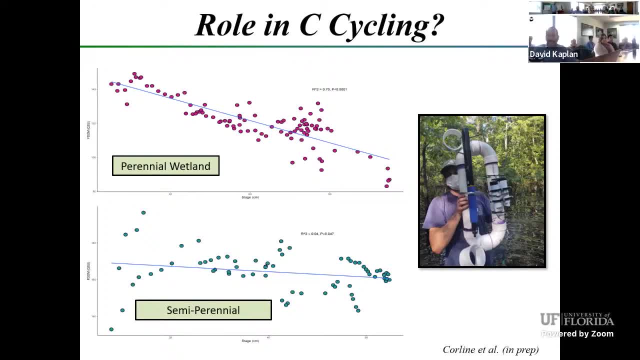 studies is that the concentration of dom and stream, dom and stream, dom and stream increases with discharge uniformly, increases with discharge uniformly, increases with discharge uniformly, and the explanation and also the mean and the explanation and also the mean and the explanation and also the mean concentration increases with wetland. 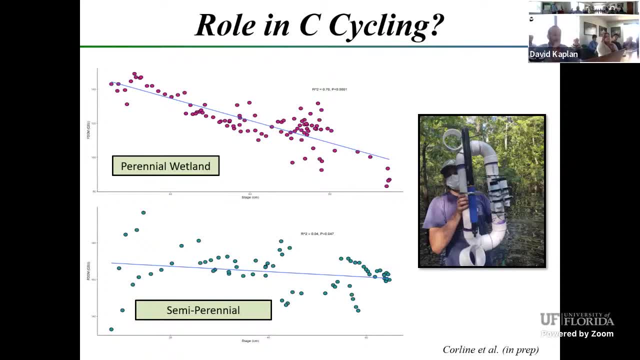 concentration increases with wetland concentration increases with wetland density. so those, both of those things i density. so those, both of those things i density. so those, both of those things, i think like they're. you know nothing in think like they're. you know nothing in think like they're. you know nothing in science is locked down. but i'm going to. 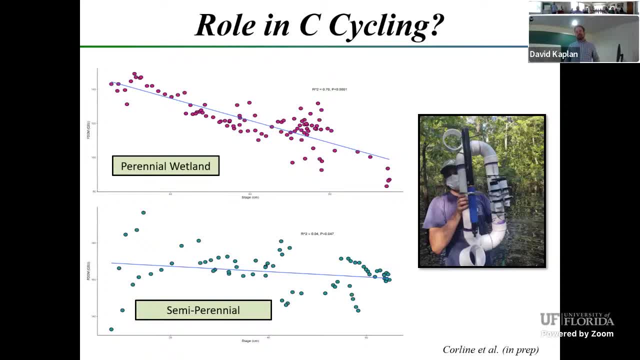 science is locked down, but i'm going to. science is locked down, but i'm going to call those a given. i get that, yeah, and call those a given. i get that, yeah, and call those a given. i get that, yeah, and so this suggests the opposite effect. 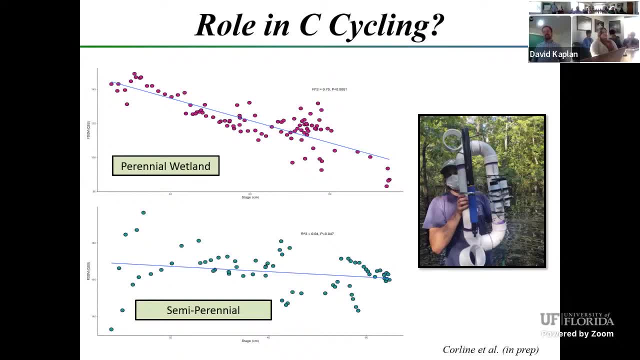 so this suggests the opposite effect. so this suggests the opposite effect: that you should see dilution of stream, that you should see dilution of stream. that you should see dilution of stream. dom as the wetlands become connected. dom as the wetlands become connected. dom as the wetlands become connected because they're producing, storing less. 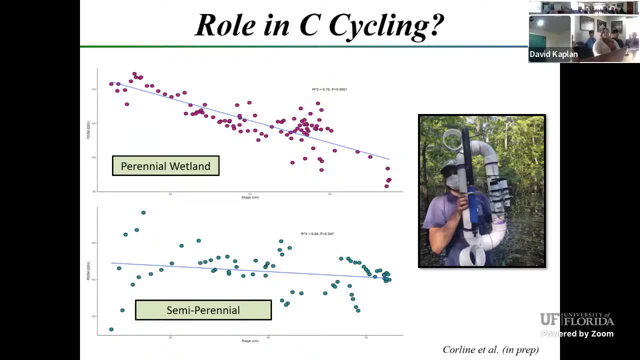 because they're producing, storing less. because they're producing, storing less, and so what's the explanation? but can and so what's the explanation? but can and so what's the explanation? but can you draw the cross section just real? you draw the cross section just real. you draw the cross section just real quick. but they're also not exporting. 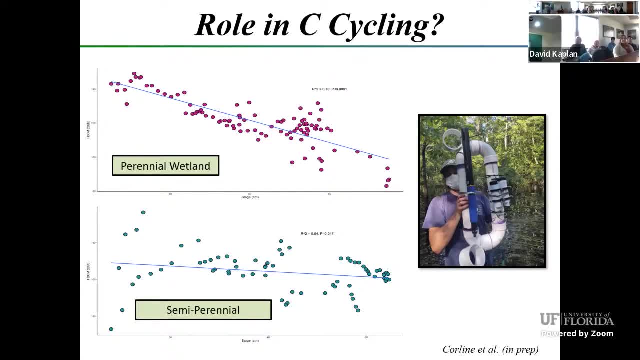 quick, but they're also not exporting quick, but they're also not exporting when they're high, unless it's such purpose. unless it's such purpose, unless it's such purpose because you've got this wetland over, because you've got this wetland over, because you've got this wetland over here, and so you've got this is your area. here, and so you've got. this is your area here, and so you've got. this is your area where you're creating your dom right. where you're creating your dom right. where you're creating your dom right, we're at chalk top, but then the other. we're at chalk top, but then the other. 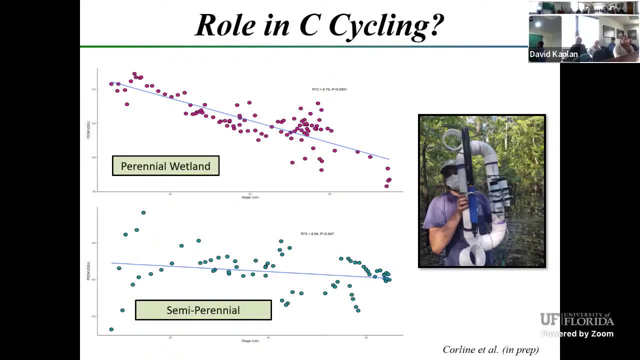 we're at chalk top. but then the other weapon is like this: right yeah. so your weapon is like this: right, yeah, so your weapon is like this: right yeah. so your stage is just getting more and more, stage is just getting more and more. stage is just getting more and more participation. 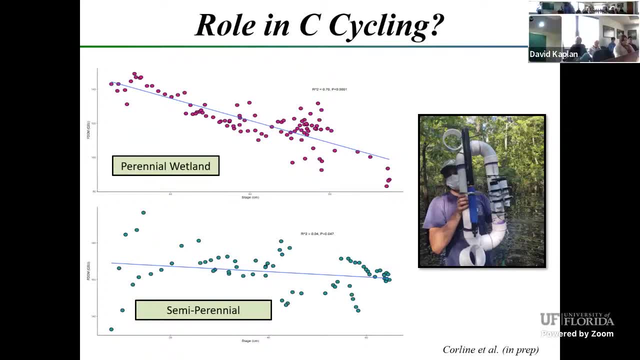 participation, participation, right, i mean that's exactly what you're right. i mean that's exactly what you're right. i mean that's exactly what you're saying and we have saying, and we have saying, and we have not me. uh, scotty has a student who is. 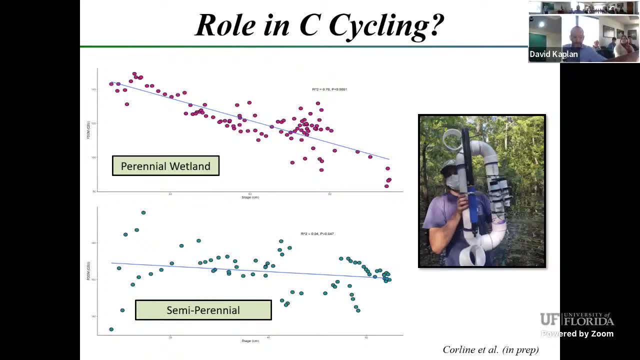 not me. uh, scotty has a student who is not me. uh, scotty has a student who is actually measuring extractable organic, actually measuring extractable organic, actually measuring extractable organic matter. going from this matter, going from this matter, going from this down from, but to your point, i think. 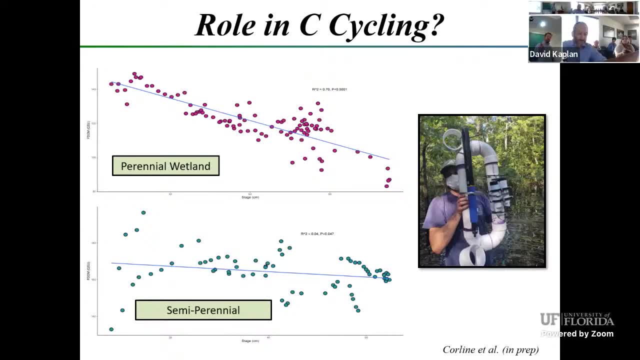 down from, but to your point. i think down from, but to your point. i think it's, maybe, it's, maybe, it's maybe. well, if it was just isolated weapons, well, if it was just isolated weapons, well, if it was just isolated weapons, then i would suggest it might be. 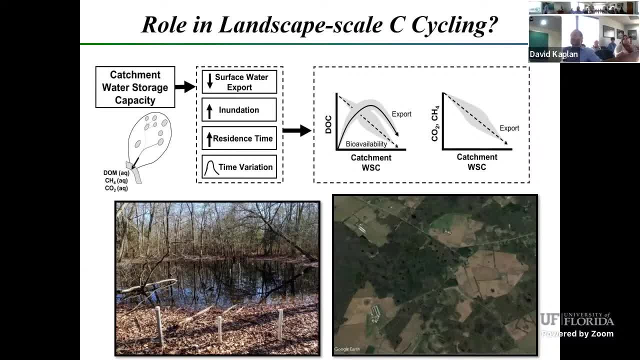 then i would suggest it might be, then i would suggest it might be right, right, right, do that right, do that right, do that right. you have to have the connections right. you have to have the connections right. you have to have the connections to have the export. but if you're really 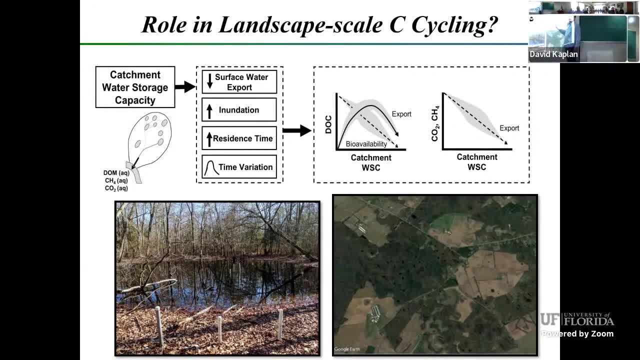 to have the export, but if you're really to have the export, but if you're really wet, wet, wet, you are having that dilution effect across. you are having that dilution effect across. you are having that dilution effect across the land. has that ever been observed? 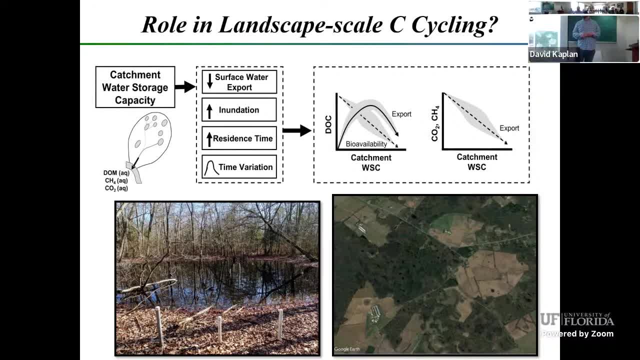 the land. has that ever been observed? the land has that ever been observed? because i think you have floodplains, because i think you have floodplains, because i think you have floodplains, wetlands, wetlands, wetlands. they're also probably generating this. they're also probably generating this. 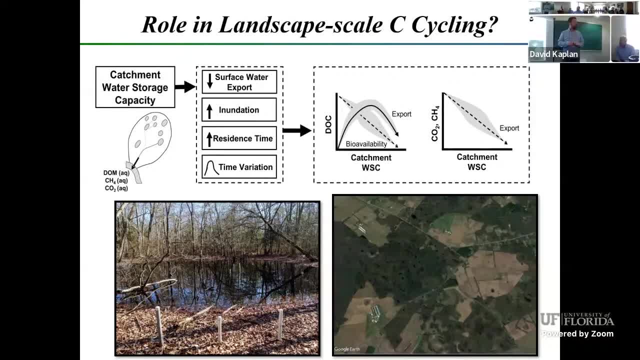 they're also probably generating this right, right, right. but it's not just the symmetry of the but it's not just the symmetry of the but it's not just the symmetry of the wetland right, it's also the connectivity. wetland right, it's also the connectivity. 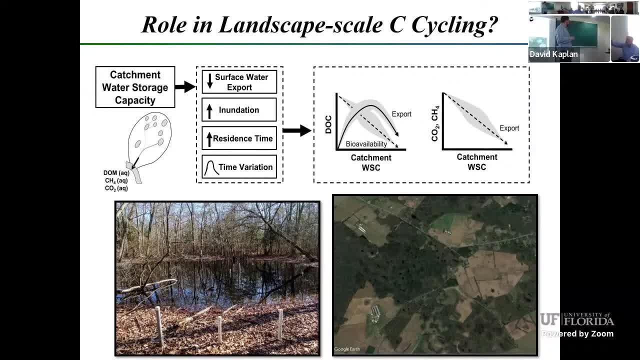 wetland right. it's also the connectivity to the landscape of the running event. so to the landscape of the running event, so to the landscape of the running event. so where you have the dilution, it may make, where you have the dilution it may make. where you have the dilution, it may make sense that it really is isolated from. 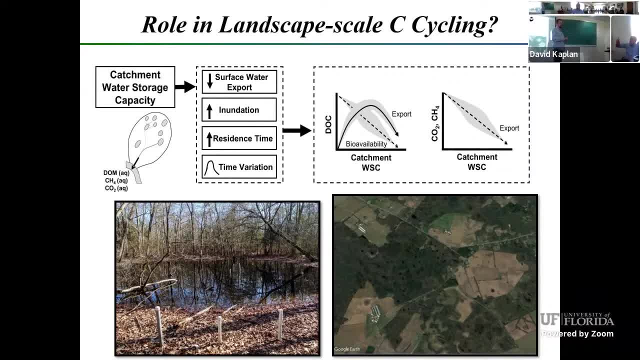 sense that it really is isolated from sense, that it really is isolated from running and you're really just getting running and you're really just getting running and you're really just getting atmospheric input and the doc is just atmospheric input and the doc is just atmospheric input and the doc is just coming from the sediment underneath it. 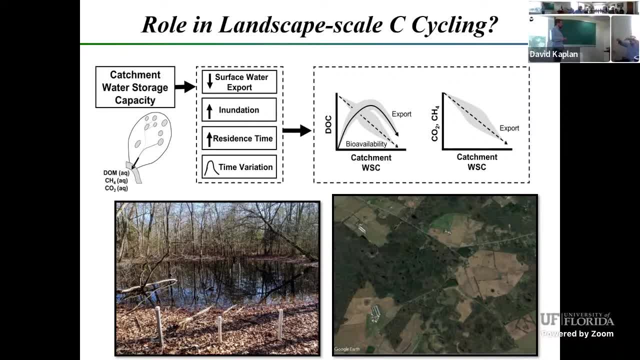 coming from the sediment underneath it, coming from the sediment underneath it, whereas other wetlands, including this, whereas other wetlands, including this, whereas other wetlands, including this bathymetry one, you may have a catchment bathymetry. one. you may have a catchment bathymetry. one. you may have a catchment area around it that you're getting. 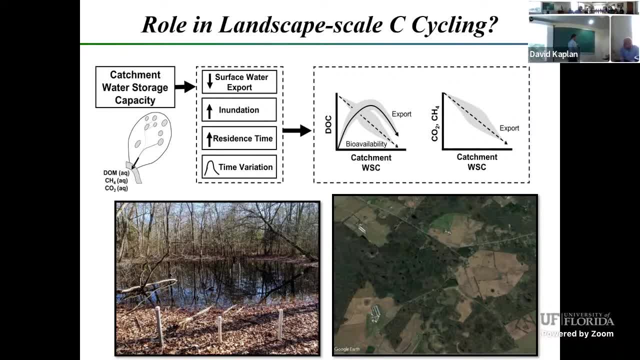 area around it, that you're getting area around it that you're getting, you know, run off through our, you know run off through our, you know run off through our already inundating more area and this already inundating more area and this already inundating more area, and this one's more connected than this one is. 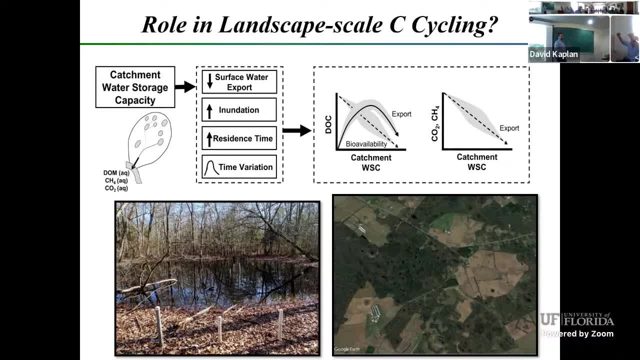 one's more connected than this. one is right, but you could have a shape like right. but you could have a shape like right. but you could have a shape like that, but still have a contributing area that, but still have a contributing area that, but still have a contributing area during the rain event. that's still. 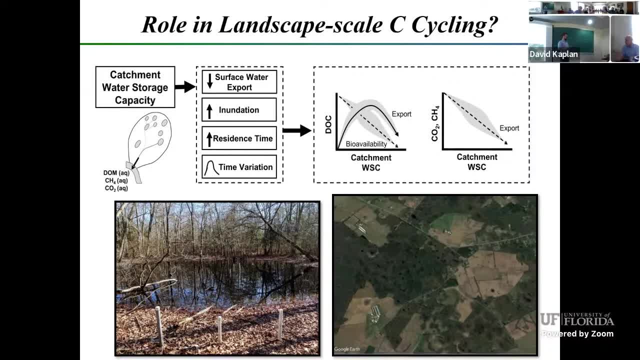 during the rain event. that's still during the rain event. that's still dragging quite a bit of doc. so yeah, it's dragging quite a bit of doc. so yeah, it's dragging quite a bit of doc. so yeah, it's not just the bathymetry of the wetland. not just the bathymetry of the wetland, not just the bathymetry of the wetland, it's also the connectivity to the. it's also the connectivity to the. it's also the connectivity to the watershed. sure, and i would say that the watershed, sure, and i would say that the. 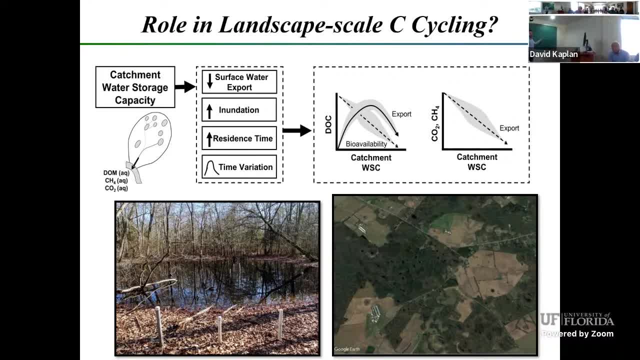 watershed, sure, and i would say that the symmetry of the wetland, probably symmetry of the wetland probably indicates its potential connectivity, indicates its potential connectivity, indicates its potential connectivity, right, so it's not too bold like you, right? so it's not too bold like you, right? so it's not too bold like you have this wetland that it's more doc. 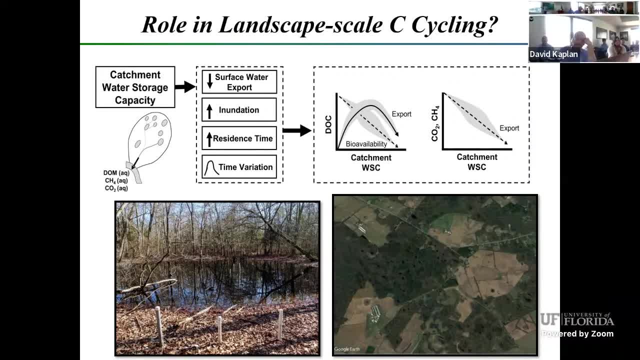 have this wetland that it's more doc. have this wetland that it's more doc, but probably is more often connected, but probably is more often connected, but probably is more often connected. and is that i mean it's that barrel of and is that i mean it's that barrel of? 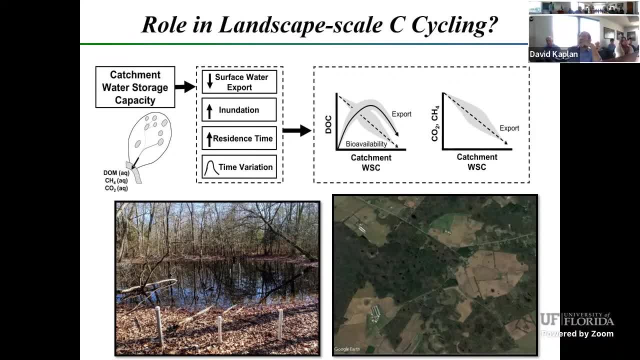 and is that? i mean, it's that barrel of like recession rates, like recession rates, like recession rates, just the cylindrical one has got a, just the cylindrical one has got a, just the cylindrical one has got a slower recession rate. and yeah, slower recession rate and yeah, slower recession rate. and yeah, it does. it does. it does all right. we'll do one more and we'll let all right. we'll do one more and we'll let all right. we'll do one more and we'll let you go, of course. if you have to run to, you go, of course, if you have to run to. 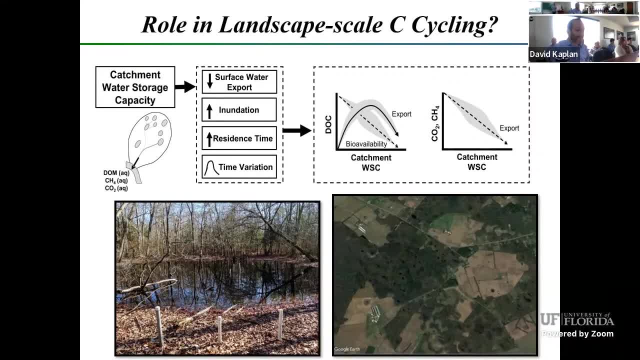 you go, of course, if you have to run to class. please do one more question from class. please do one more question from class. please do one more question from the group. i know i hear it and i hear dr. i know i hear it and i hear dr. 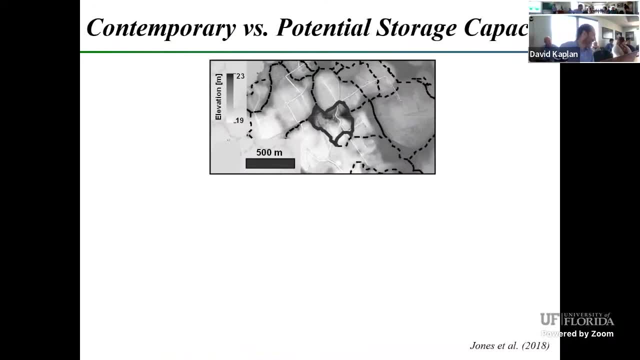 i know, i hear it and i hear dr: well, yeah, but if you're registered, make well, yeah. but if you're registered, make well, yeah, but if you're registered, make sure you sign up, sure you sign up, sure you sign up, yeah, and one of the two sheets.